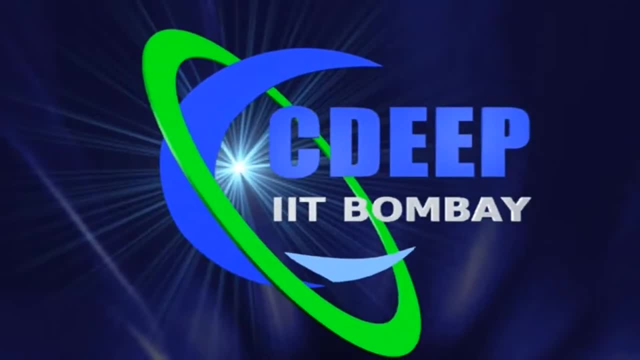 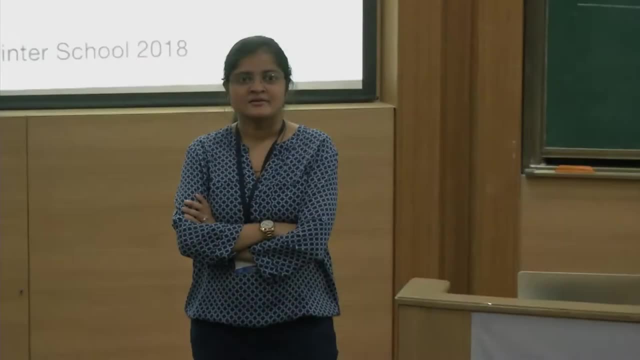 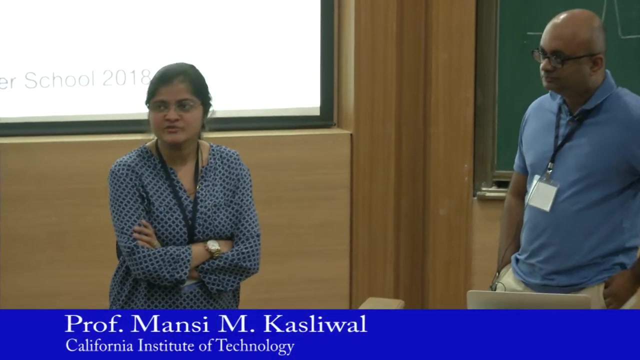 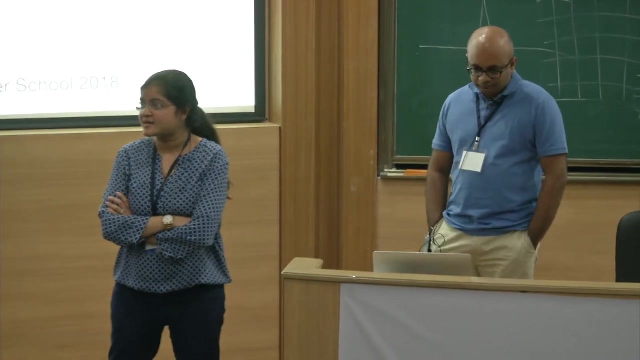 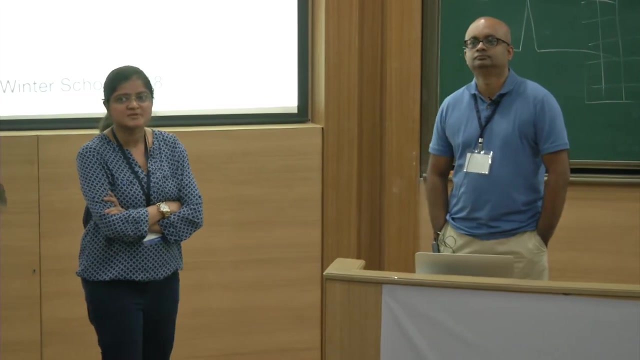 All right. now that you have reduced images, it's time to learn how to do some photometry. So your lecture for how to do photometry will be by Professor Sudarshu Bhatni, also from IIA. Professor Bhatni did his PhD at Frankfurt University and then went to IIT, worked with 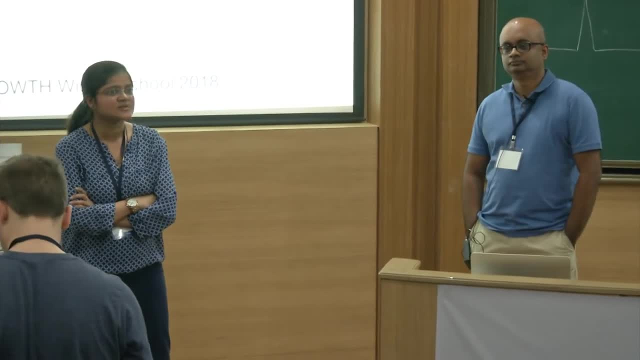 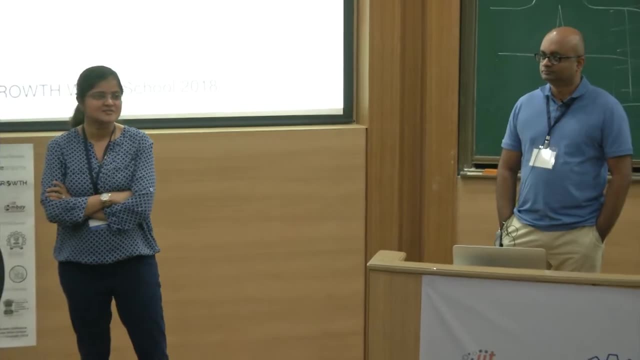 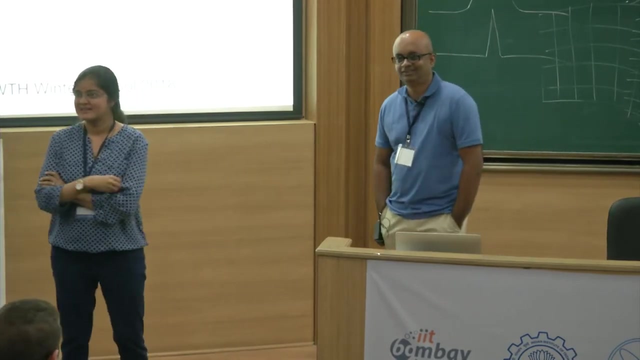 Professor Nitin Pari, and then spent a decade in South Africa working at SAO And during the gravitational wave events of August 17, 2017, a lot of the beautiful infrared data that you see was data collected by him, So you can hear straight from the watcher's mouth. 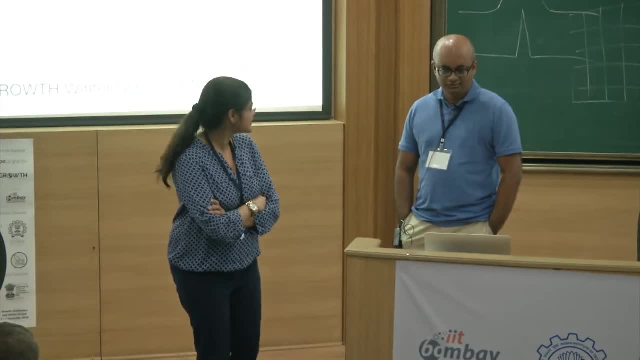 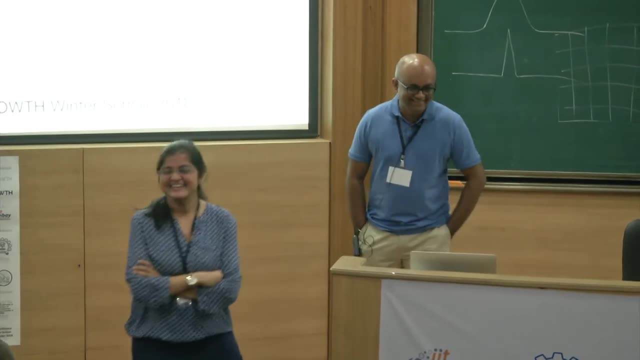 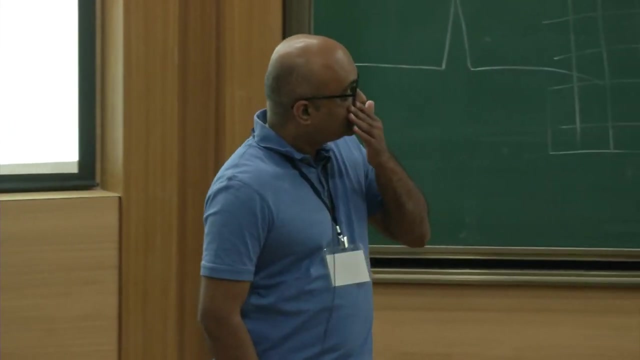 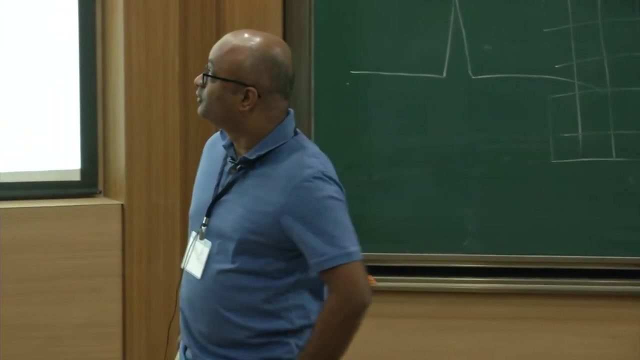 how to actually do photometry And that gets published in 10 papers all in one. I don't know. Lost account, Okay. so yeah, this talk is about how to basically do the photometry From your previous tutorial. you have reduced image with you. 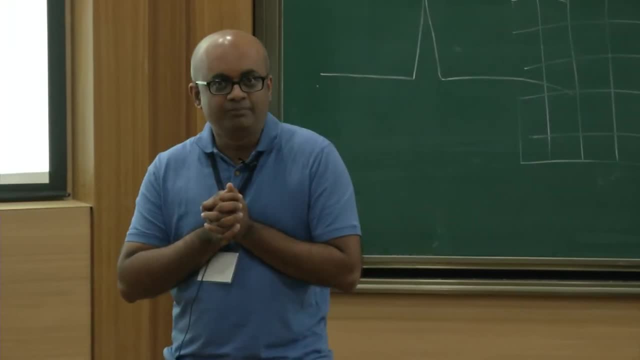 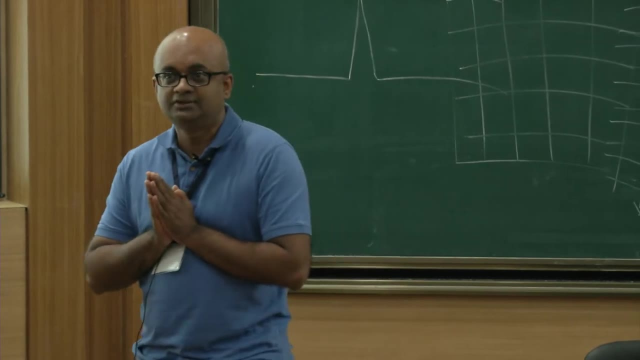 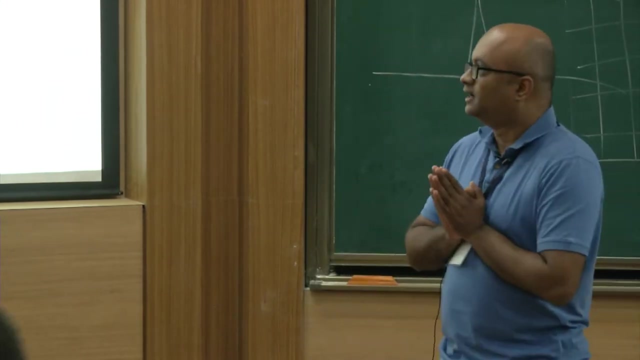 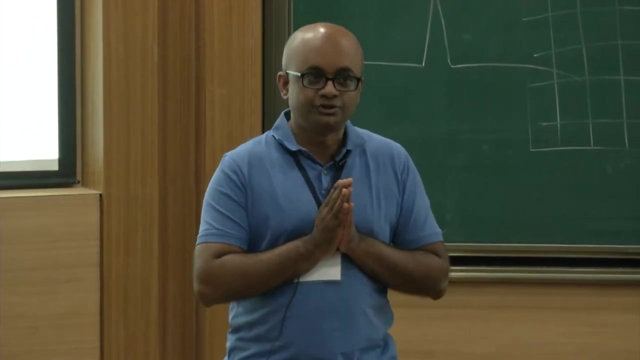 So now you have an image And, well, briefly, well without going into much detail, I will tell you what photometry is and what are some of the requirements that you should know before you actually do the photometry And then afterwards, hopefully, you will be able to do the next tutorial okay. 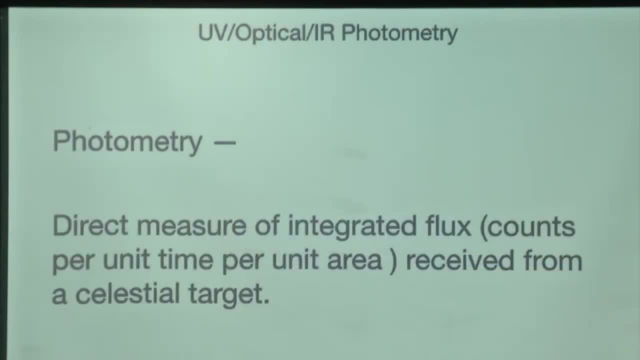 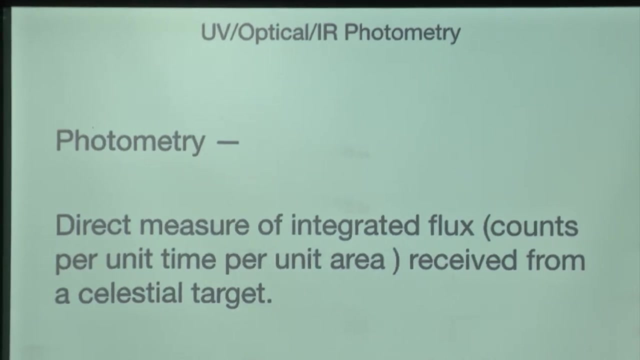 So what photometry is? It's basically a direct measure of integrated flux, That is, counts per second, per time, per unit area received from a celestial object. So once you have an image, you have to measure counts or integrated flux from the object of your interest. 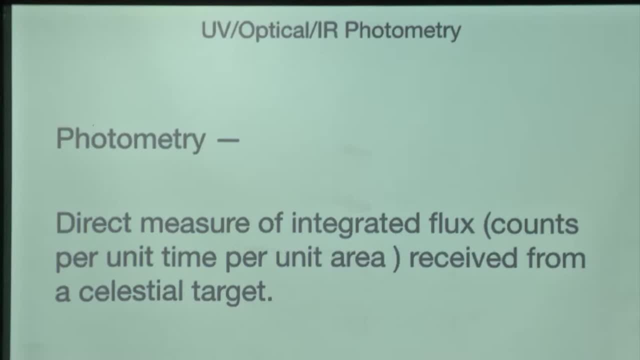 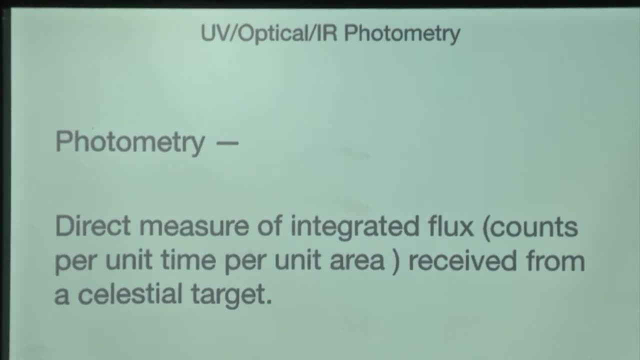 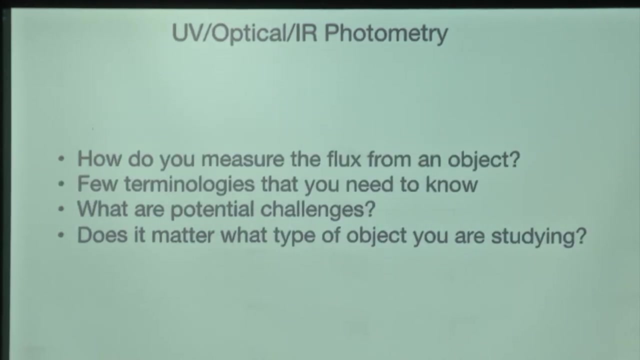 And then, in this session, we are going to learn the techniques and tools, how we can measure the fluxes, or integrated flux, from your object of interest. okay, So The thing that we are going to see in this session: how do you measure the flux from? 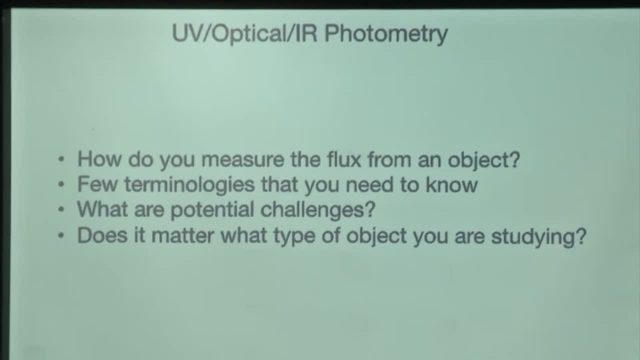 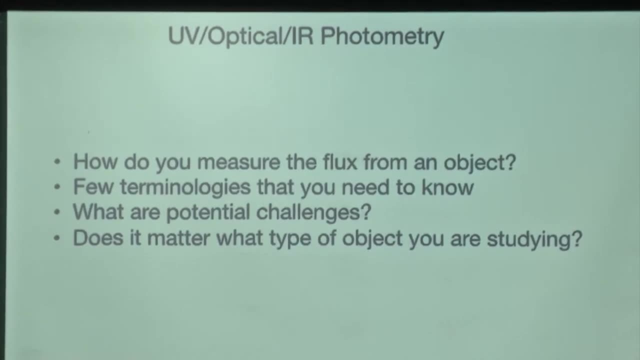 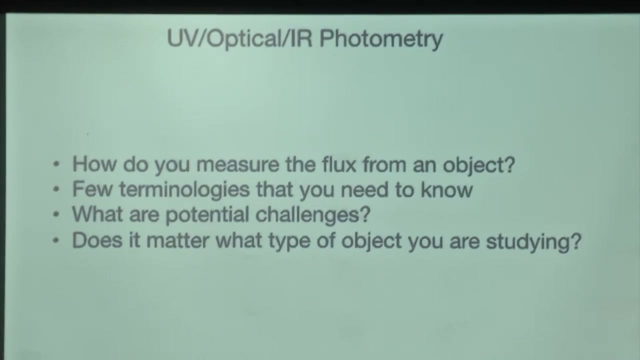 an object, An object before actually doing so, some terminology that you may need to know. And then, what are the challenges that you might face, apart from the software tools, techniques, And obviously, does it matter what type of object you are studying? 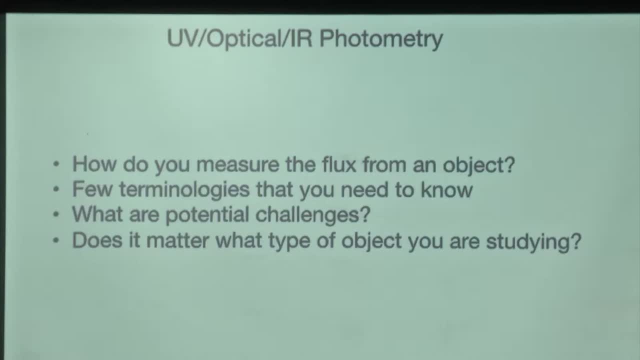 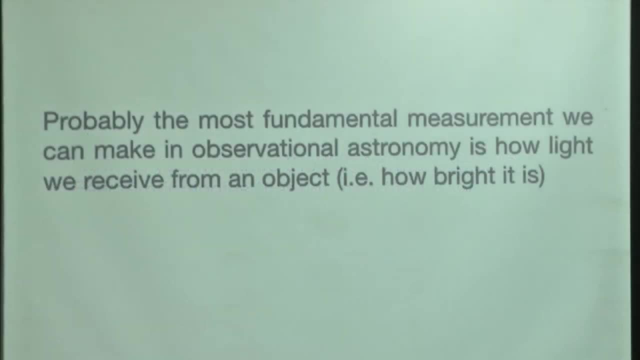 That is, What is the type of photometry or techniques that you are using. that depends on the type of object you are studying. So it is probably the most fundamental measurement that we can make in observational astronomy. That is how actually we measure the light that we are receiving from an object which 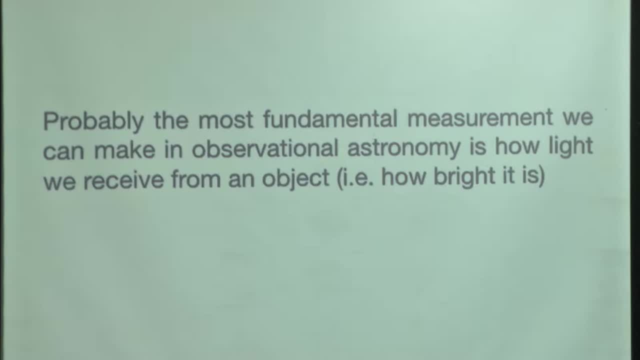 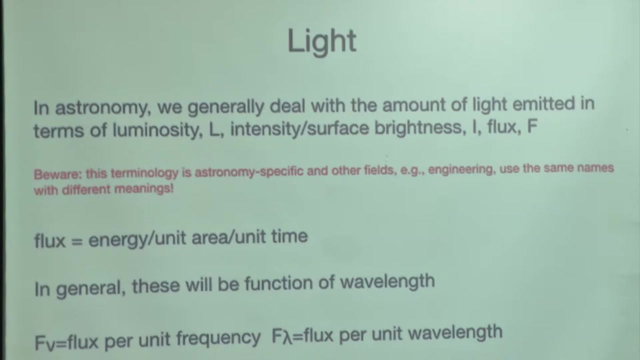 means that how bright or faint that object is. So that is what basically we are going to see. Okay, So that is basically one thing we want to do in observational astronomy and in photometry. So just briefly, what the light is. In astronomy, we generally deal with the amount of light emitted in terms of either luminosity, 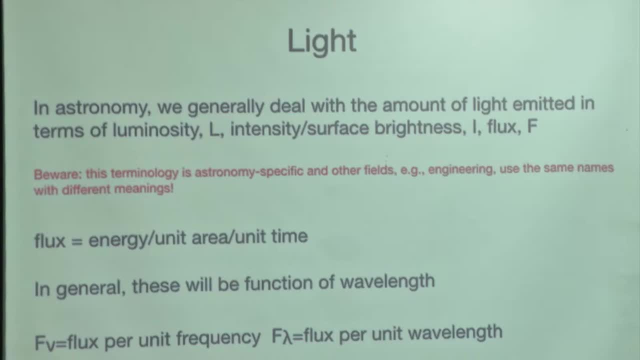 or intensity, or if you are measuring, if you are having extended object, that is, in terms of surface brightness or in flux. So flux typically you define as Okay: Energy per unit area, per unit time and this will be generally a function of wavelength. 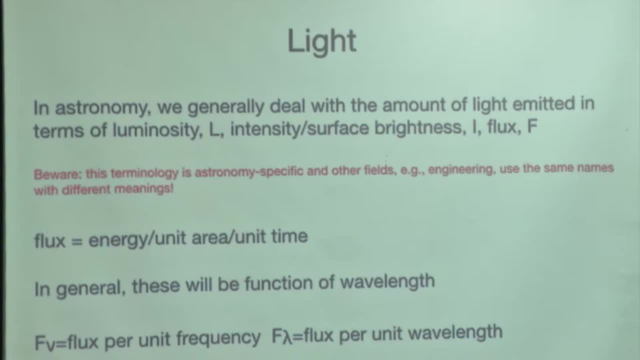 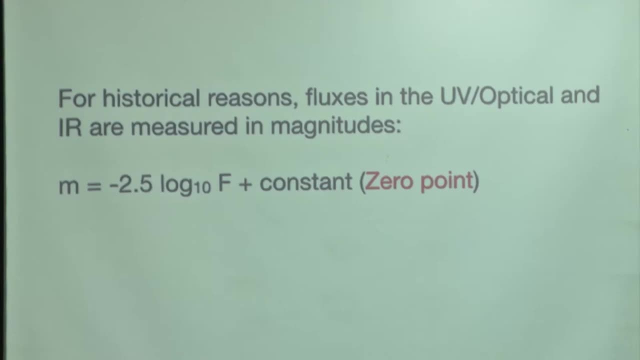 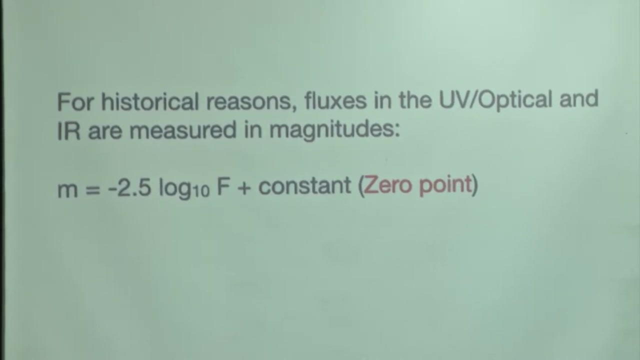 So lot of the time you will see either F nu or F lambda when you basically measure the flux. So for historical reasons, in UV, optical and IR astronomy we measure the fluxes or we represent the fluxes in terms of magnitudes. Okay, 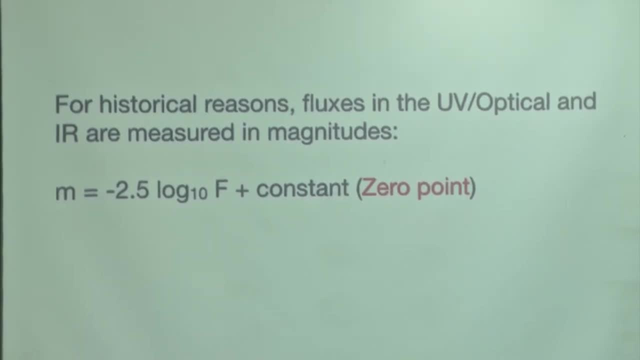 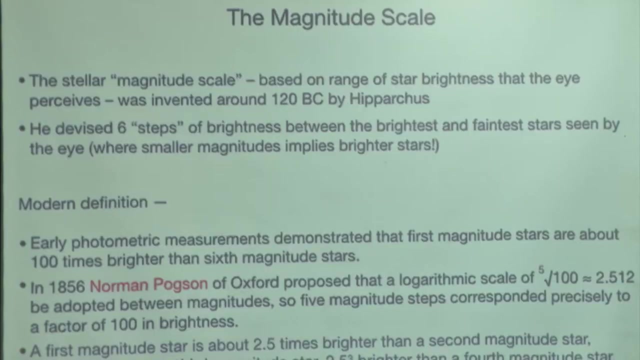 So the magnitudes we define using this equation, minus 2.5 log of 10 F, plus a constant, which many times we see a 0. So let us first see what this magnitude is, and this slide basically gives a basic information about a magnitude or a stellar magnitude scale. 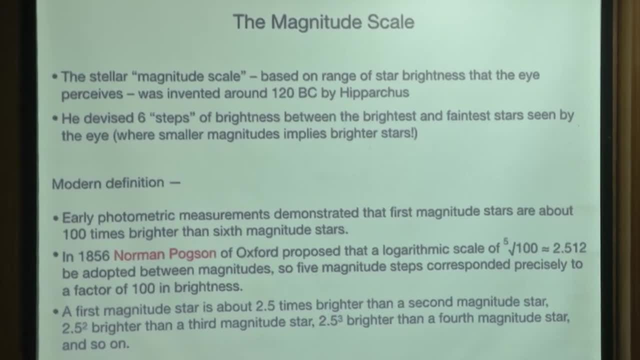 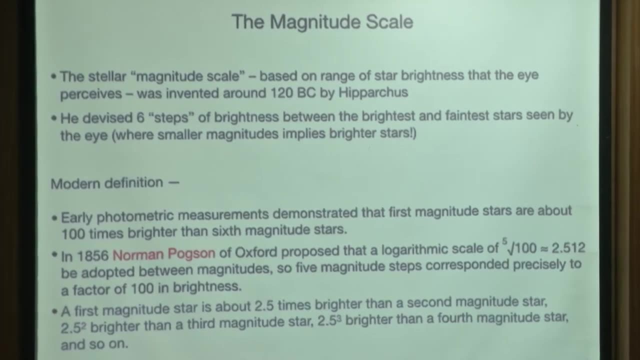 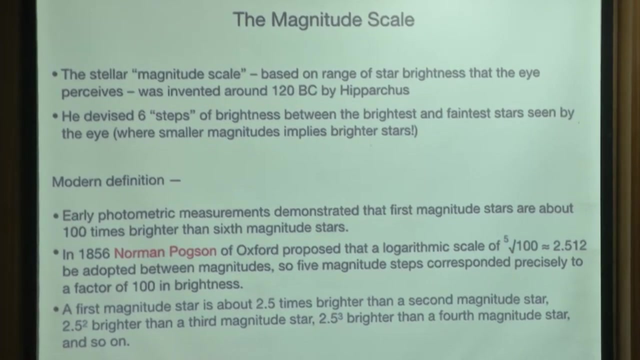 So the stellar magnitude scale is basically based on the range of star brightness that your eye can perceive, which was invented around 120 BC by Hipparchus. So he devised the 6 step brightness between the brightest and the faintest star seen by eye, where the smaller magnitude implies a brighter star. 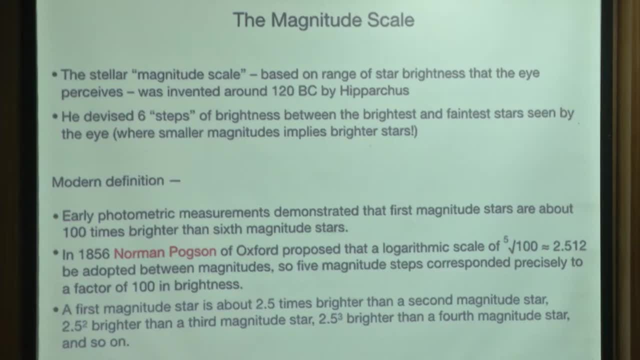 So, if you are talking about a magnitude 1 of a star, which means you are seeing a brighter star compared to a star which has a magnitude 5 or 10.. Okay, Okay, Okay, Okay, So this definition got modified, and what the steps that we have taken to modify this definition? 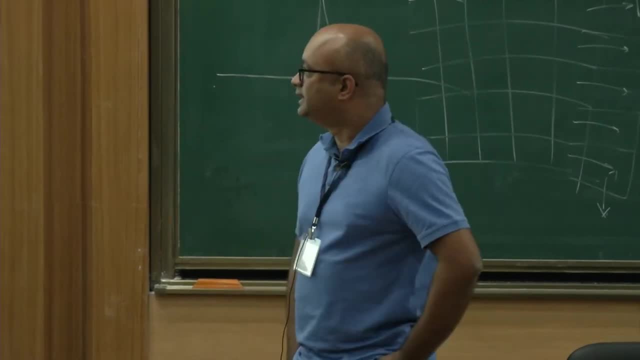 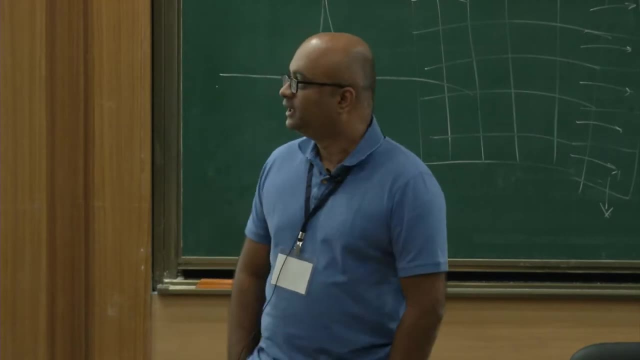 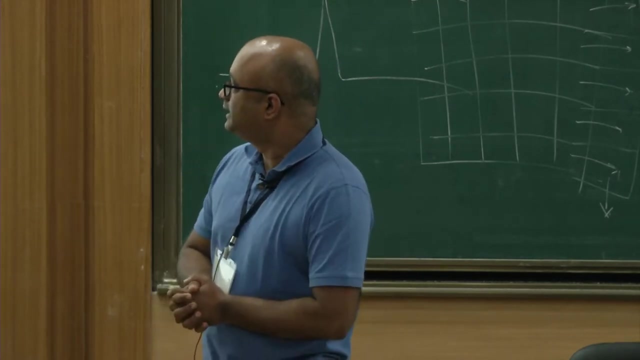 is that early photometric measurements that demonstrated that the first magnitude stars are about 100 times brighter than the 6 magnitude stars. Okay, So in 1856, Norman Foxen of Oxford proposed that the first magnitude stars are about 100 times brighter than the 6 magnitude stars. 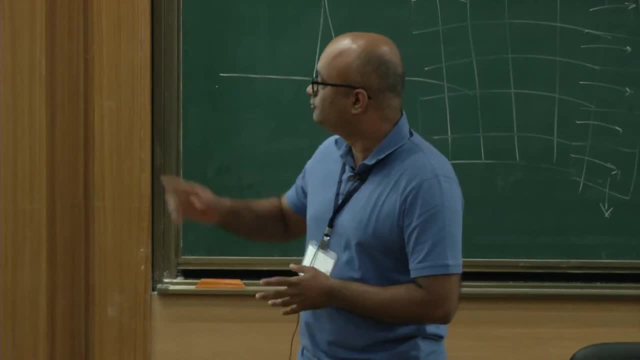 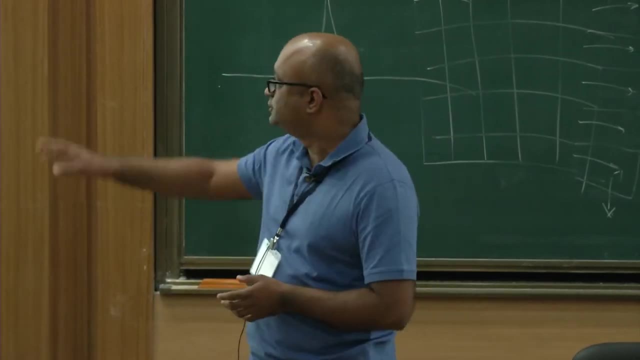 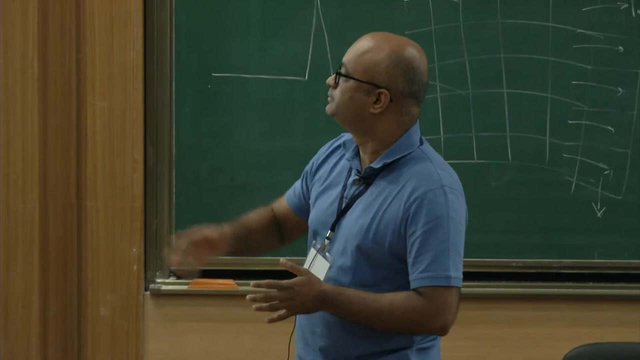 Okay. Okay, There should be a logarithmic scale of, of this number, 100, the root of 5, which approximately gives you a 2.5 to be adopted between the magnitudes. Okay, So that the 5 magnitude steps correspond precisely to the factor of 100 in brightness. 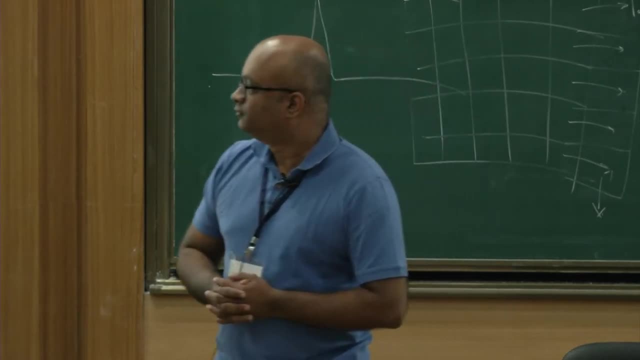 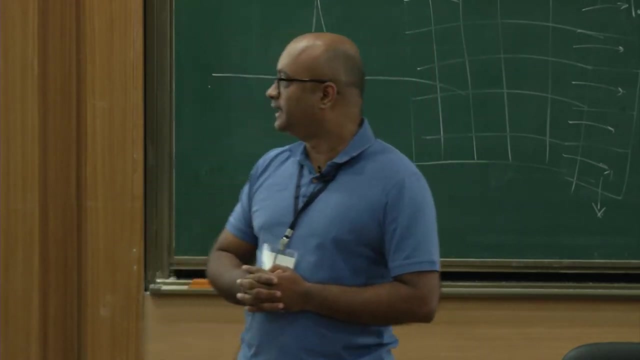 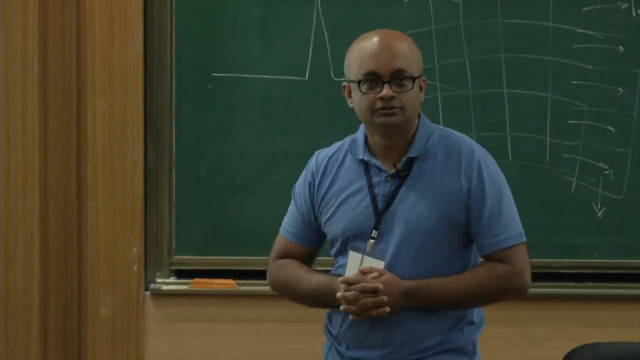 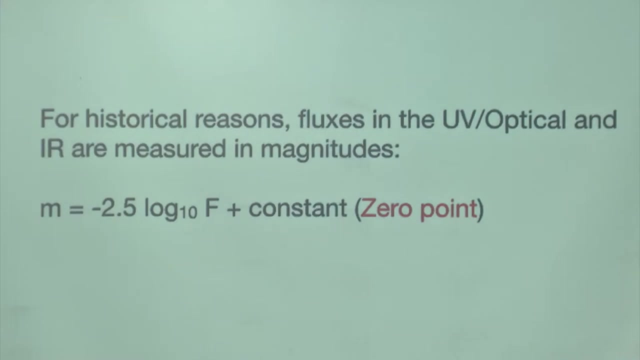 Okay. So, for example, if you have a first magnitude star that will be 2 point times brighter than the 6 magnitude stars, Okay, than the second magnitude star, and 2.5 square times brighter than the third magnitude star, and so on and so forth. ok, So that is how you get this equation where you can actually 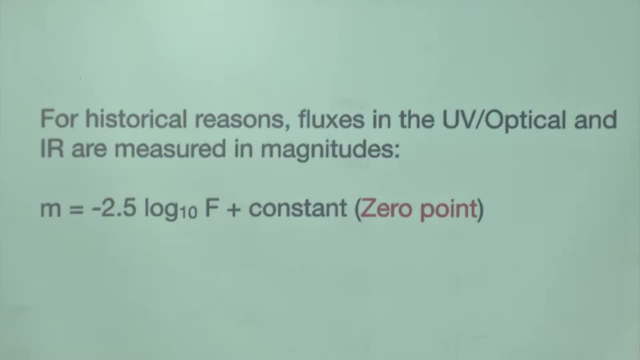 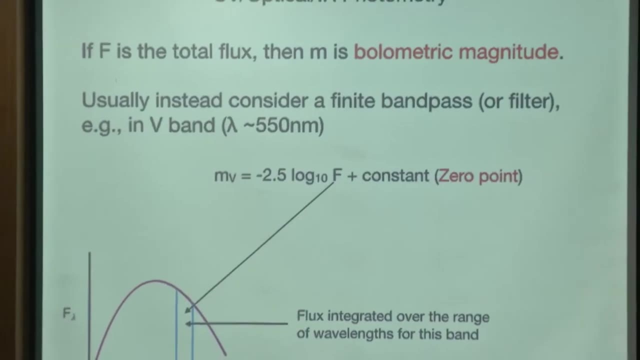 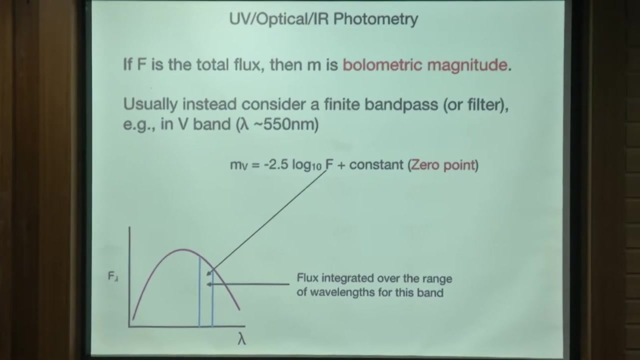 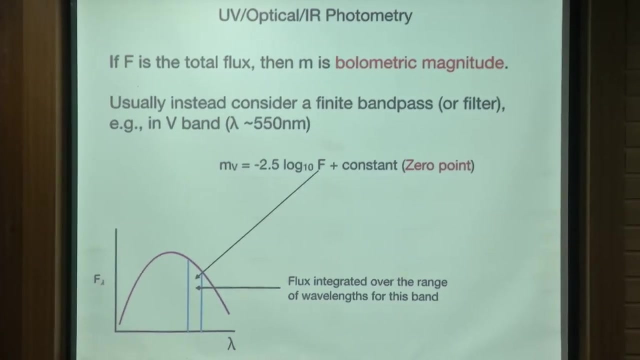 get the magnitude, which is minus 2.5 log 10 of the wave length. Now, so what we have? So this is a plot between the wave length and the flux that we receive at any particular wave length, and if we just measure the total flux under this curve, then 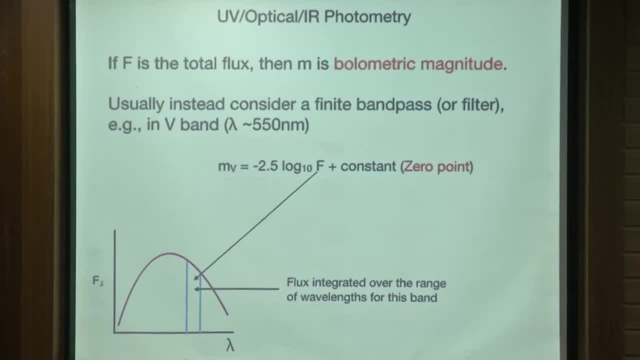 our magnitude, what we call is a volumetric magnitude. ok, But instead of doing this, normally what we do is we consider a finite band pass, or what we call filters, and we measure the fluxes in these finite band passes. So, for example, in this, in this cartoon, we are measuring the flux, a certain range of the wave length or 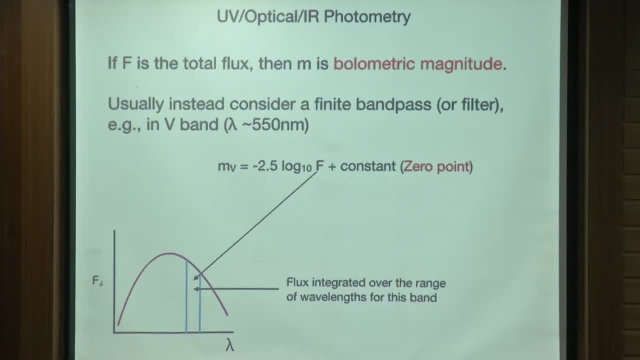 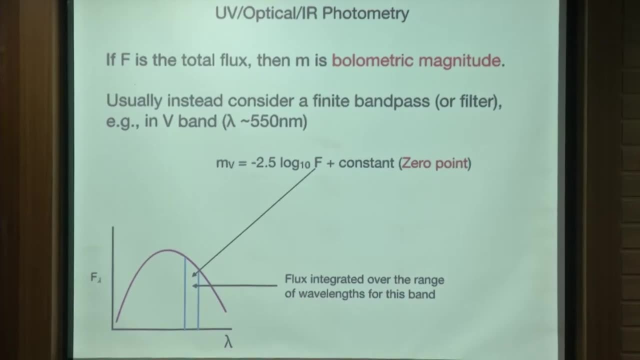 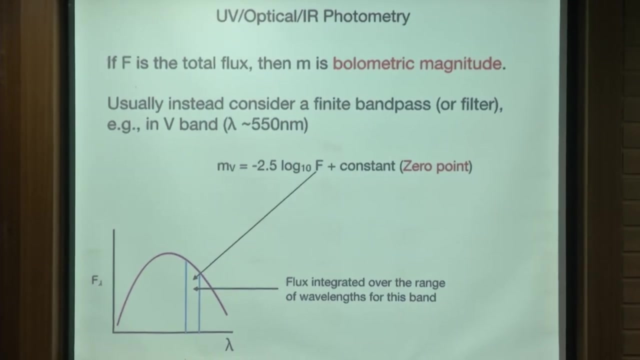 we are actually integrating the wave length, So we are integrating the flux over this range of wave length. and let us say, for example, we consider that that range is around 550 nanometers. ok, So in astronomy that we defined as a visual band, ok, So, which basically gives us a lot of information that what we are doing. 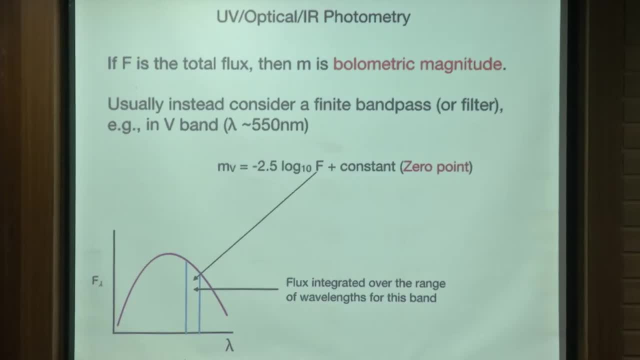 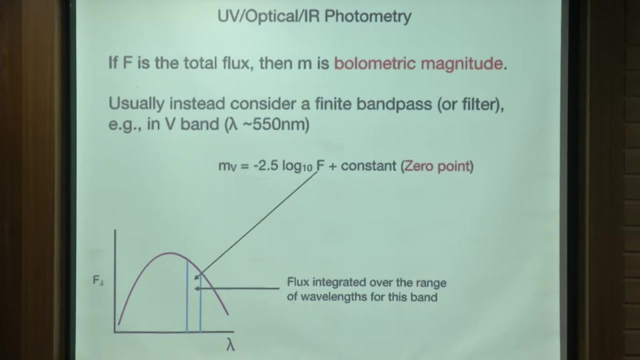 we are dividing whatever the total flux we receive into a different wave length bands. Ok, Ok, So. so that actually gives us as an idea that what sort of the fluxes we receive at a different wave length, broadly speaking, and what are a broad characteristics of these. 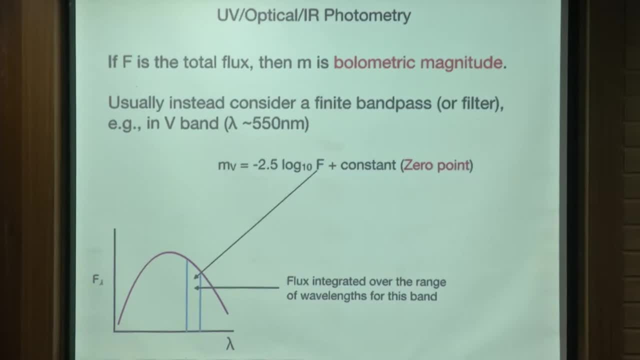 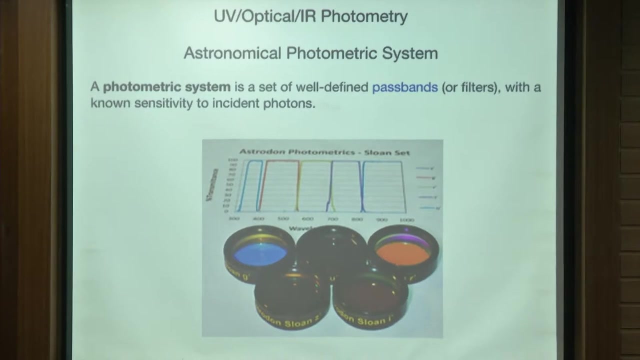 object based on the differences between the fluxes that we receive in these two bands. ok, So I will just give some more information about the fluxes, Ok, Ok. So let us look at these band passes. So what we call this, these filters or band pass, is the astronomical photometric system. 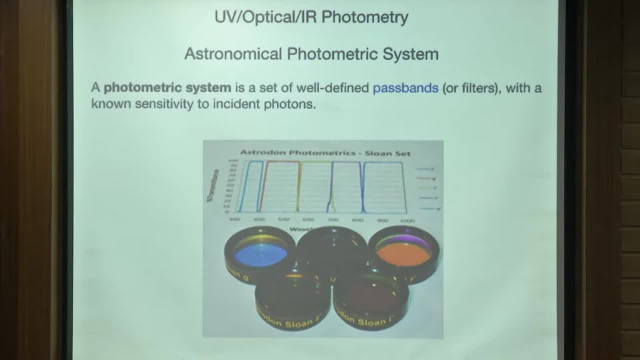 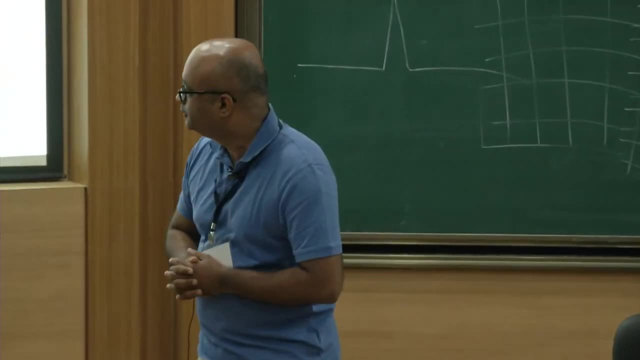 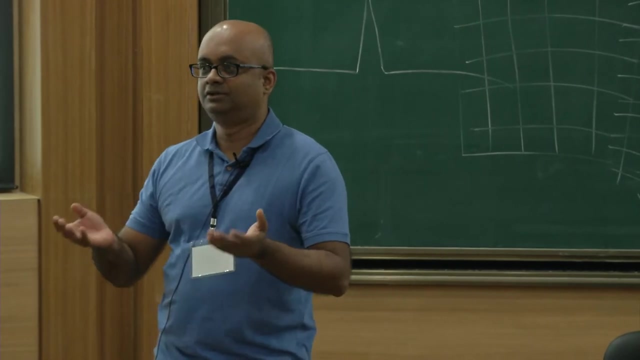 which means that they are a set of well defined filters with a known sensitivity to the incident photons. ok, So in this figure, what I have shown is basically a set of five Sloan filters. yesterday we were talking about measuring or using the filters in G, I, R. 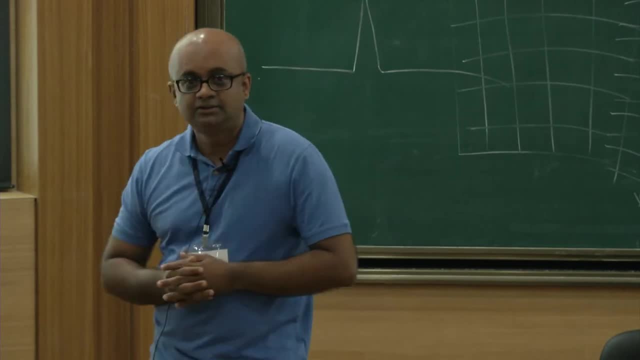 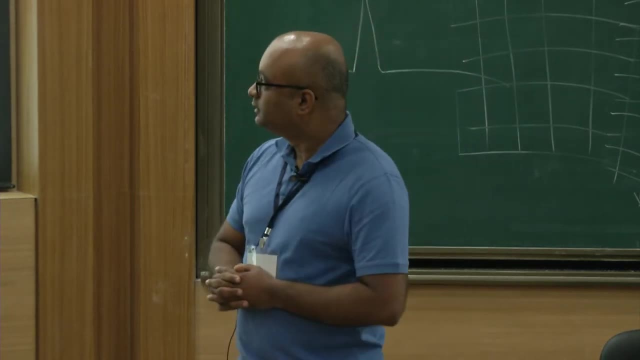 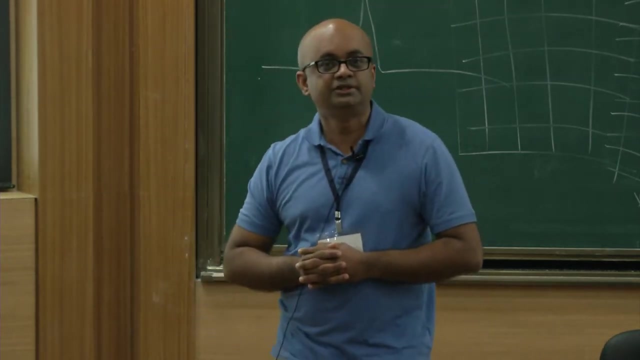 Ok, Ok, Ok, Ok. So these are basically bands, So these are basically those filters. So what it does basically is it basically allows only those photons which are sensitive to these filters to pass through it, and then you are measuring the photon in that certain 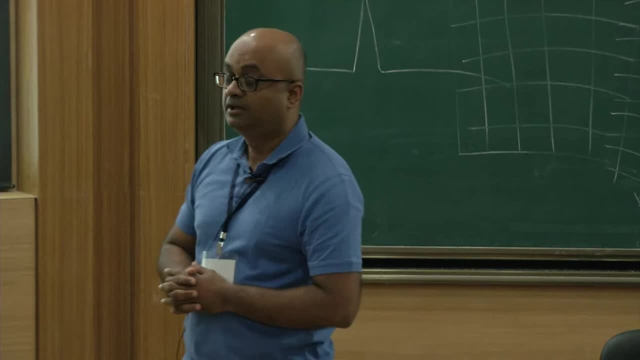 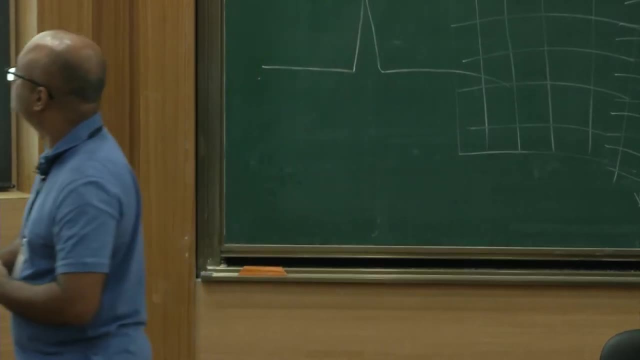 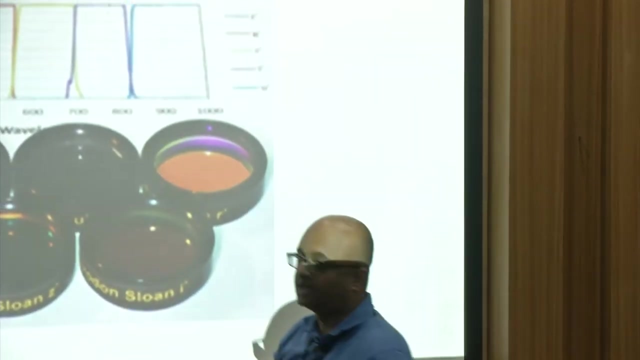 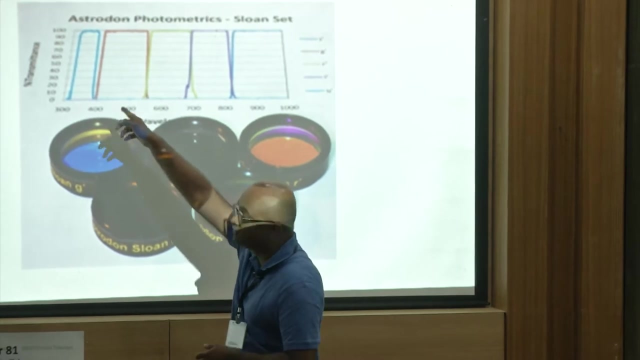 band pass. So, for example, yesterday we were measuring the fluxes of photons in G band pass, which is just somewhere here. Ok, So it basically this curve that I have shown here is a transmission curve, which basically a wavelength versus the transformation function for the filter, and it basically tells you: 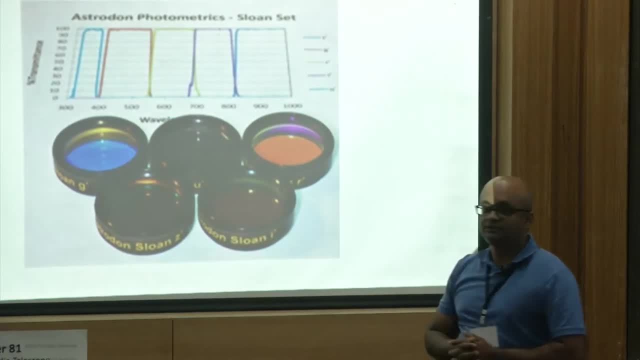 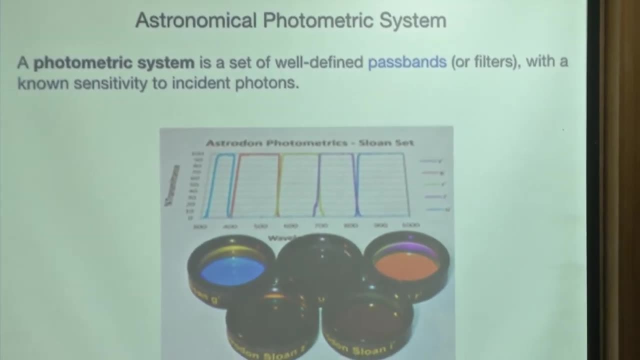 that over a what wavelength range your filter works with, which actually gives you a central wavelength for that band pass. Ok, Ok, So typically these filters or band passes, we divide into three types: broadband, intermediate band and the narrow band. So broadband. basically they have a large wavelength range. 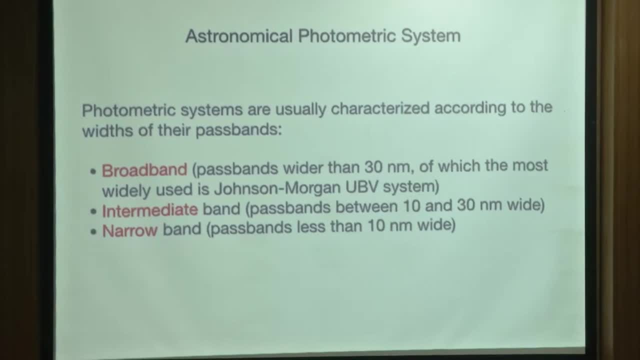 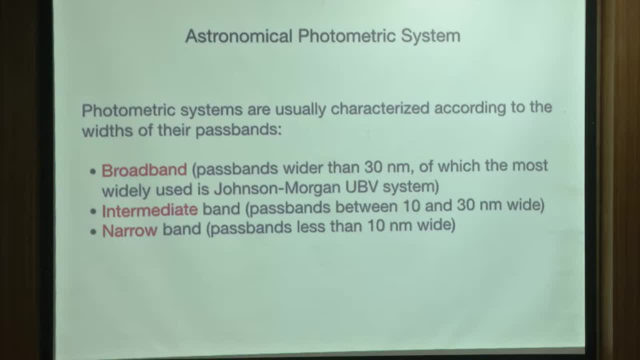 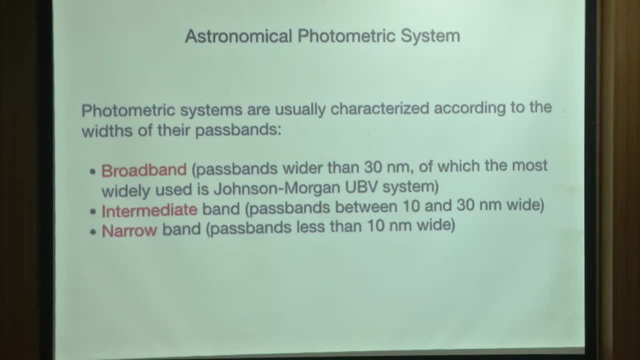 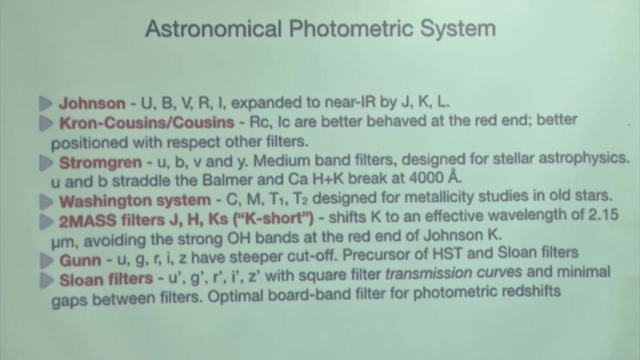 basically, it is specially designed to do some specific types of observation and their wavelength region of wavelength range is very small, around 10 nanometers. So this is just an sort of a photometry metric system available all over the observatories that we use and, as I said, normally nowadays. 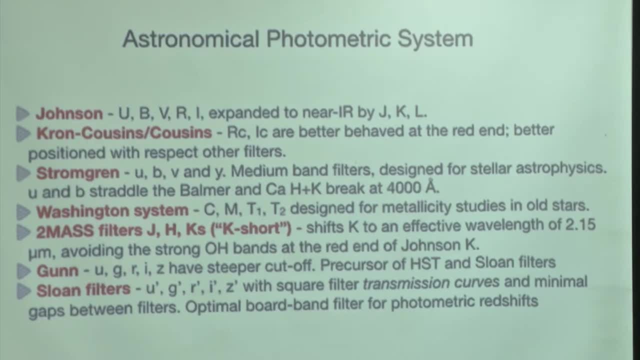 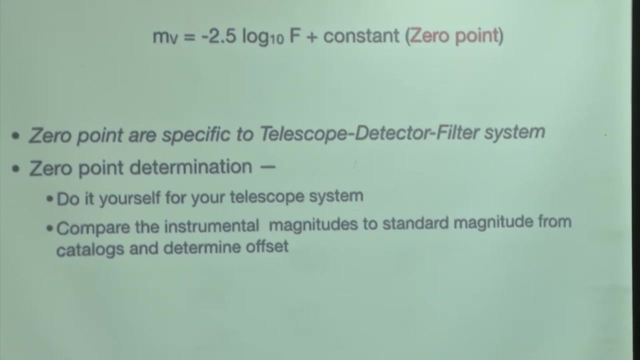 we use a Sloan standard filters when we do the the optical astrophotography. ok, So so now we know that how we can basically convert our fluxes into magnitudes and in which specific band we are we are measuring our magnitudes, So we just try to see what. 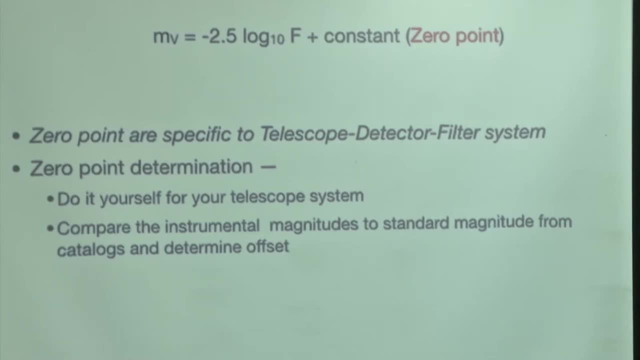 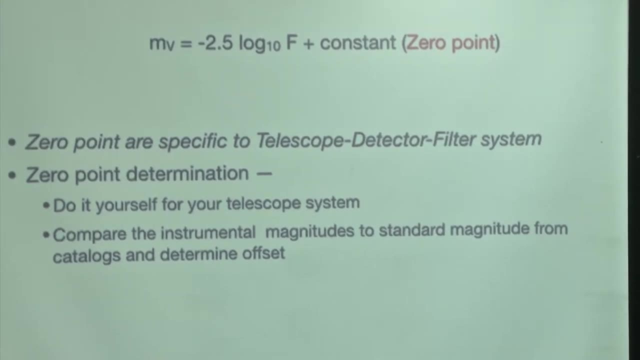 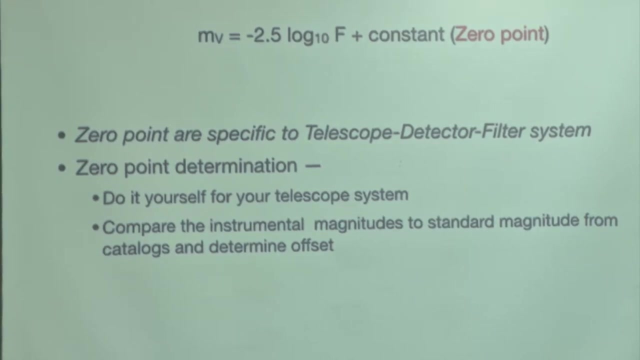 that constant is, which basically we call in many of our conversations or, as you will see in the tutorial notebook, zero point. ok, So what zero point is? So this zero point is basically specific to a telescope detector And a filter system and how basically you determine this. So either you do it by yourself, 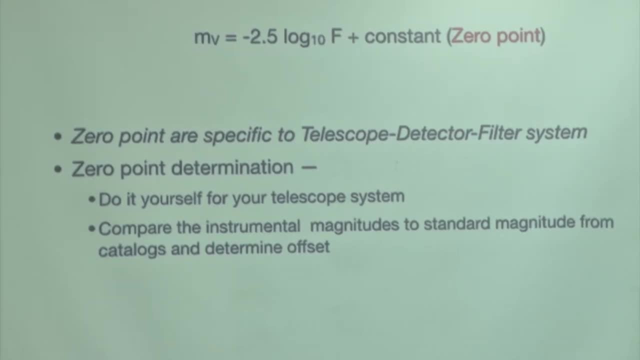 for your telescope system in, in this case, growth, or what we can do is that once we have a instrumental magnitude, that is the first part of of the the this equation, and we actually then compare this magnitudes to the standard magnitudes from the catalog and determine. 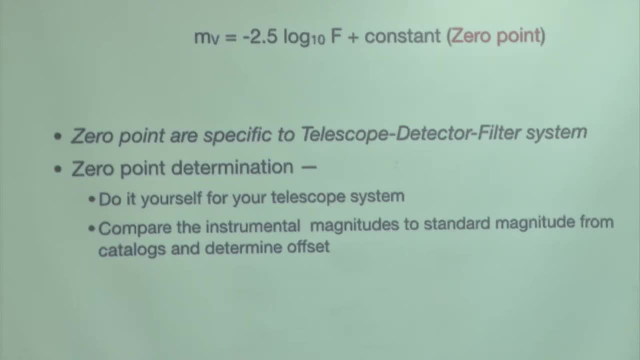 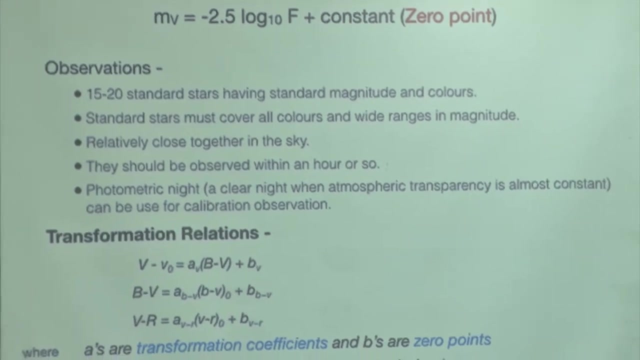 the scaling factor, And that is what I guess we will do in in the tutorial. ok, So, so that will basically give us an idea that how far our, how far away our system is from the standard system. This slide just basically gives you an old way to measure this zero point. So what, basically? 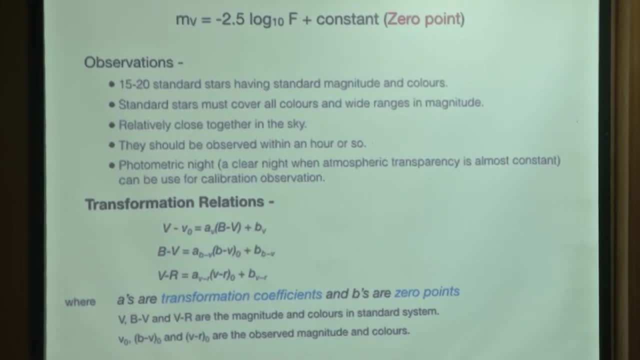 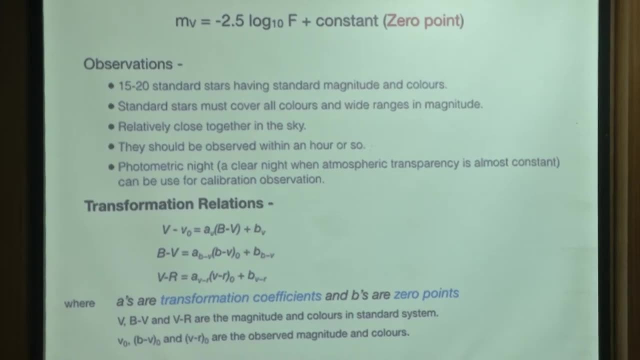 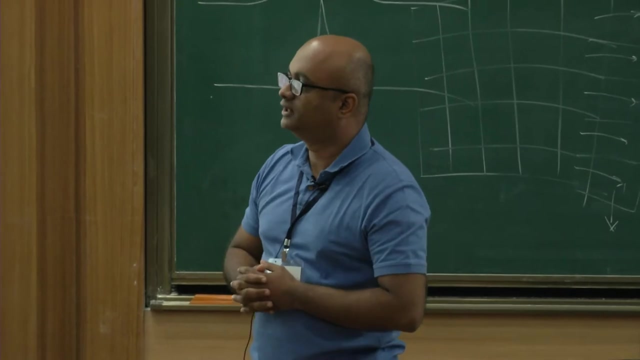 we do is that, observationally, we basically observe many standard stars which we already know what their standard magnitudes are And colors are, and they should be all over the sky, not all over the place, And sorry they should. they should relatively close together in the sky, but they should have all color. 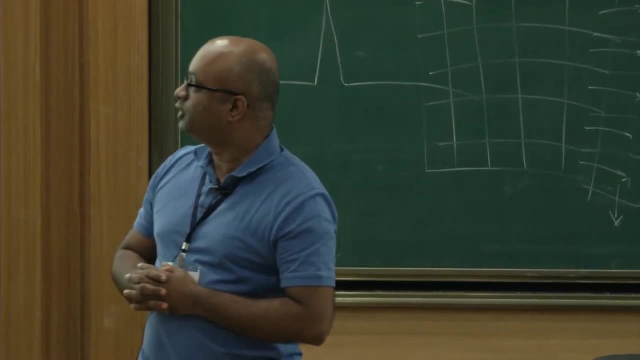 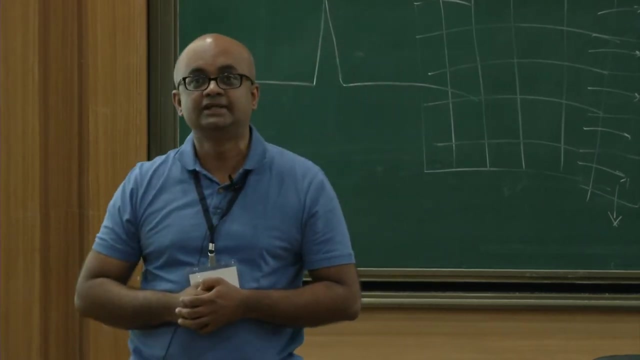 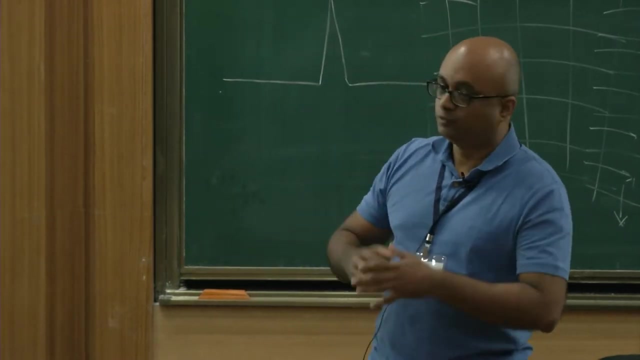 and wide range of magnitudes And they should be observed very quickly, because what we do is that when you want to determine this constant or a zero point precisely, you should worry about the sky condition And your The sky condition should not change over observing time. So generally, what we look for is a photometric 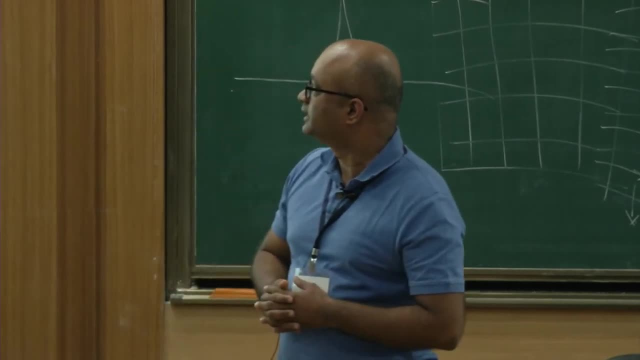 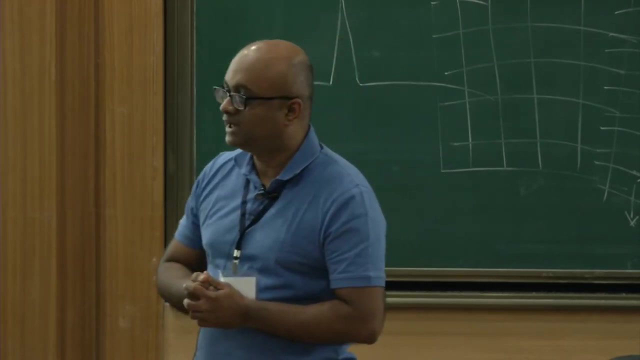 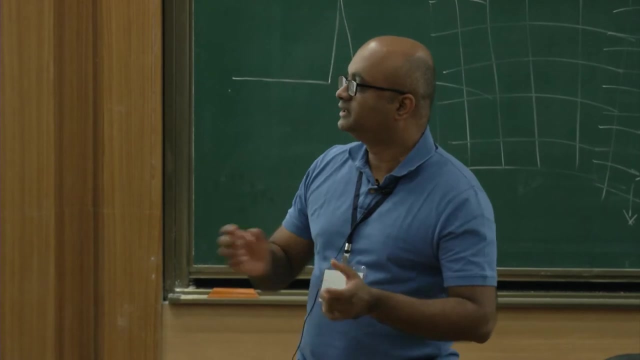 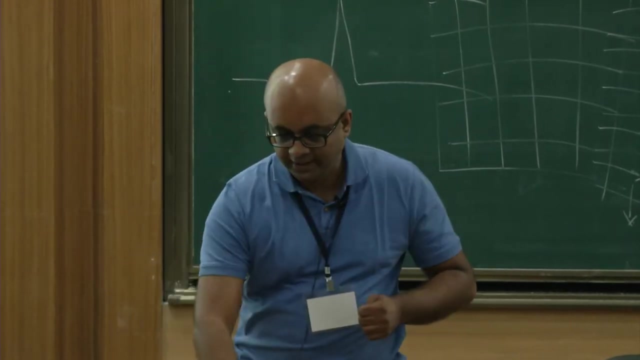 night, which means that a clear night when the atmospheric transparency is almost constant, And at that time we would observe these stars quickly. and we basically then have these kind of transformation relations where we compare the instrumental magnitude and our what we call Standard magnitudes and we basically get the the sort of zero point. So zero point in. 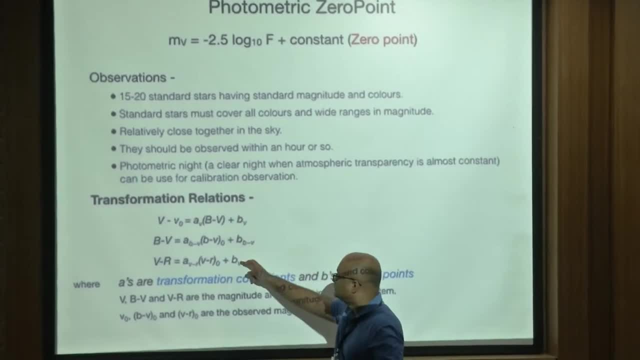 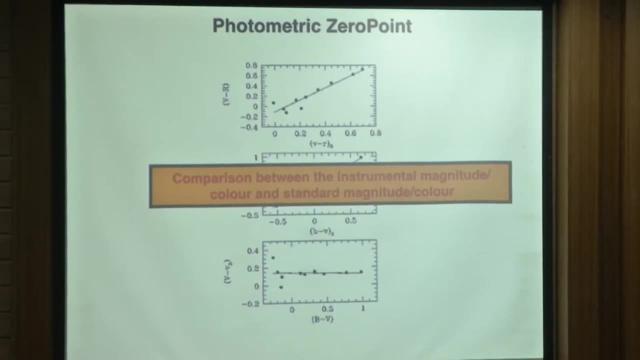 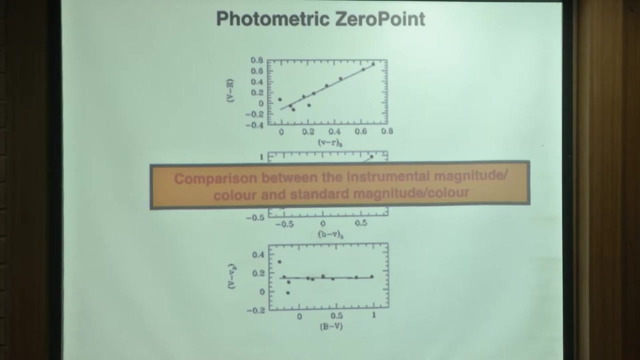 this equation is: is this for a various pass bands? ok, So, so that is, that is how we basically determine the zero point And nowadays since, as you can see from the the relative procedure, it is very expensive or time consuming to wait, So if we can observe for these standard, so we normally compare it with already, ah, ah. 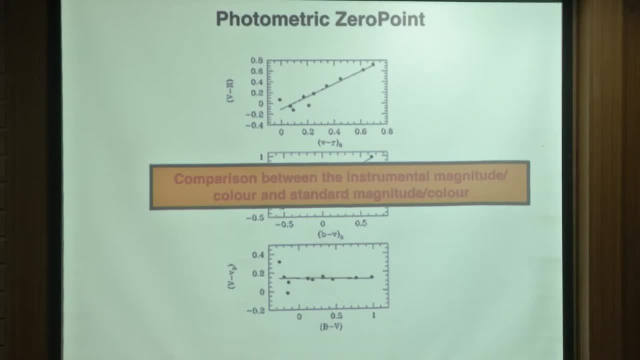 Well, ah sort of a catalogs which have done this already, and then we try to find the offsets ah between ah our magnitudes and the ah the catalogue magnitude and that we use as a zero point. ok, So now, having all these ah techniques and tools with us, ah the thing that we have to. do is to measure the fluxes, ok, So the thing that we have to do is to measure the fluxes, ok? So now we can see that we have got a very large mass here. So you can see that this is a very large mass, which is a. 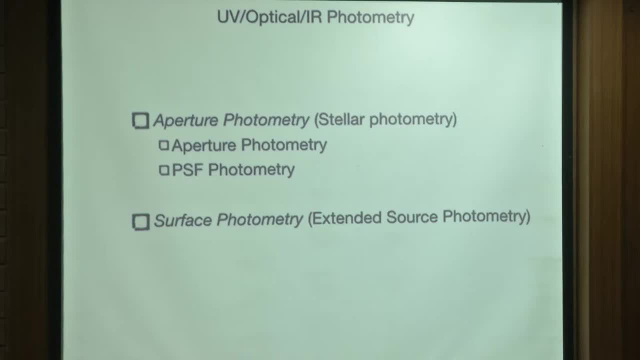 and how we do that. So we actually use this technique called the aperture photometry, which is widely used in the scalar photometry. Most of the time when we actually measure the fluxes from the stellar photometry, we use this technique. This has a two component where we do 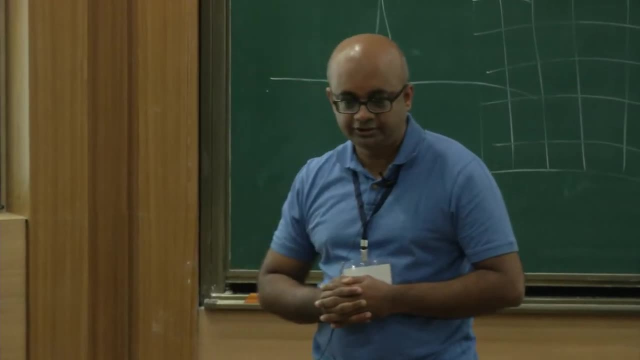 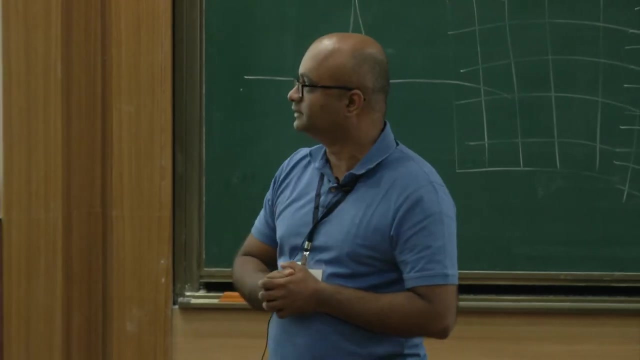 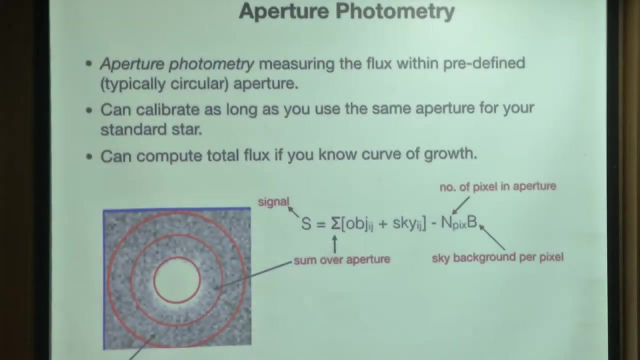 a simple aperture photometry or we do a PSF photometry and then, for extended object, we call it a surface photometry, and obviously this is not the the part of today's topic. So how we do this aperture photometry, So simply what we do. We have a object which is a star and we actually 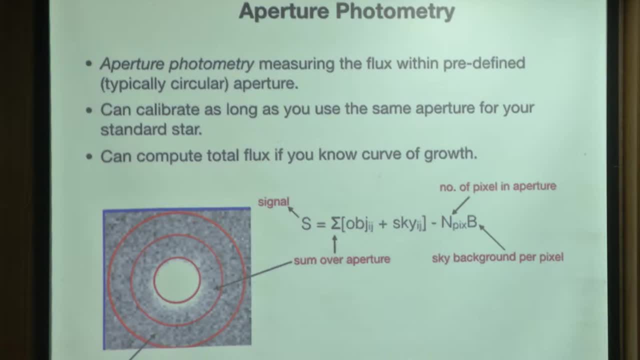 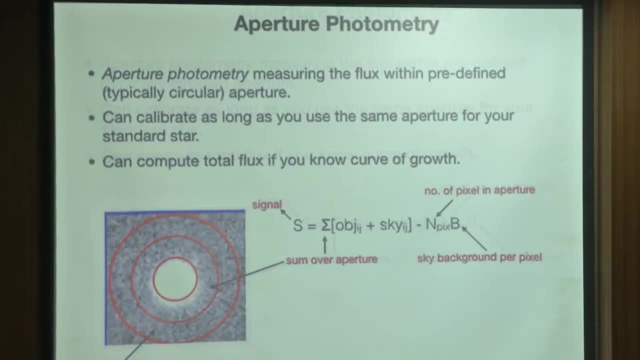 put a lot of apertures and we actually measure the fluxes within this predefined typically circular apertures. ok, So so this is a sort of a flux we want to measure. So you measure the fluxes, for example, in this or this annulus and whatever. 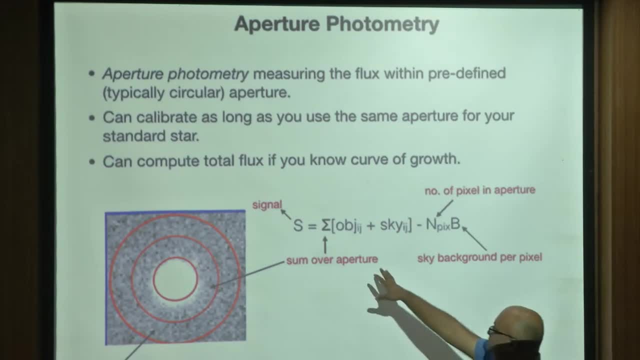 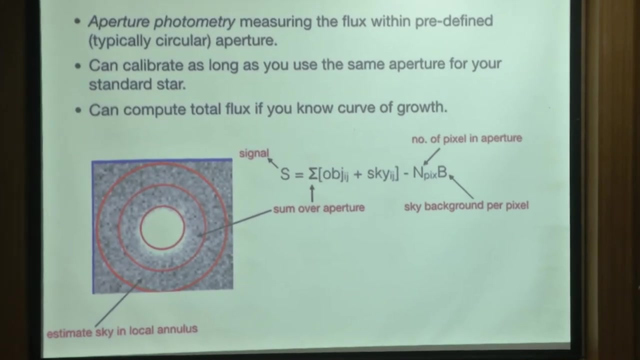 the fluxes you will have. you will sum it over, all the fluxes, and this will contain the flux from the, the object, plus the flux from the background sky. ok, But what you need to do is that you need to remove the contribution from background, and so so you need to measure the flux. 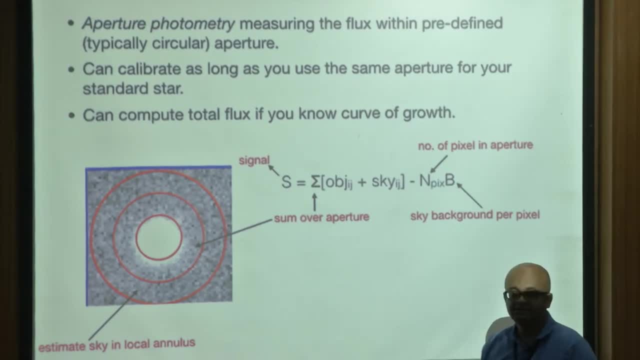 to estimate this sky in another adjacent local annulus and then you subtract it from from this object plus sky, and then you will have a flux from object itself. ok, So, so that is, that is way in, in sort of very naive way. your aperture photometry works. Of course it is not, as 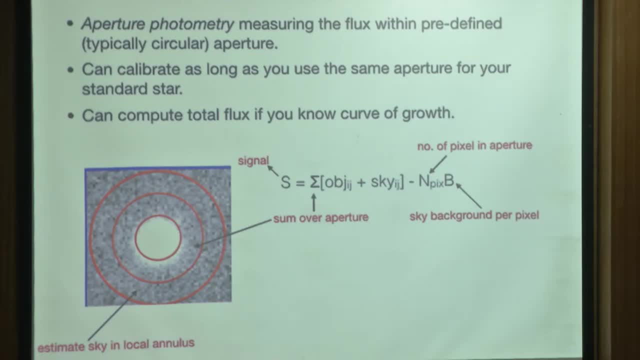 simple as when you go to the actual measurement. So the idea is that you measure the flux in one annulus or one aperture and then subtract whatever the, the sky that is around your object, from from whatever the flux measurement you've done, and you have the fluxes, integrated fluxes with, for. 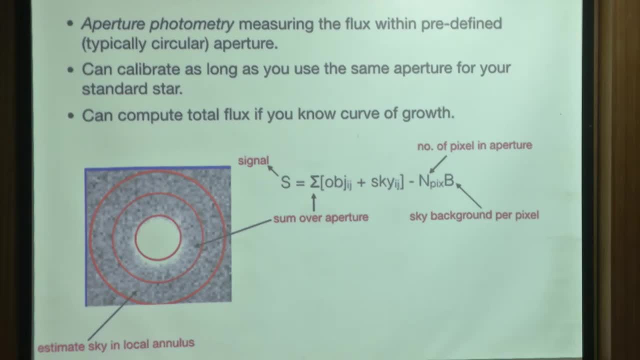 that object, then you get the magnitude, and then you proceed forward. ok, So so what? what? what I mean by proceed further is that then you calibrate your fluxes using the equation I showed in a previous slide, and then, So this flux that you measure is actually a function. 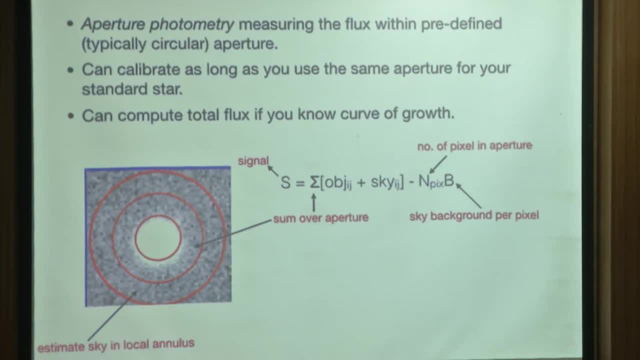 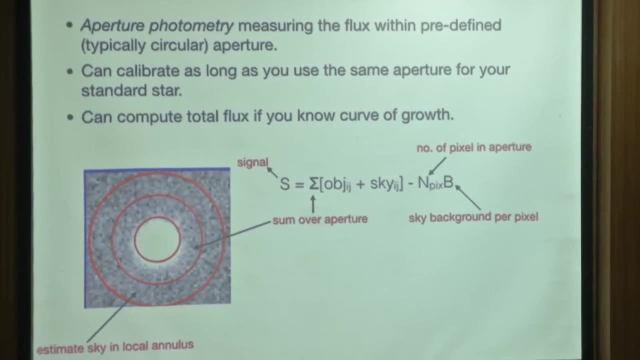 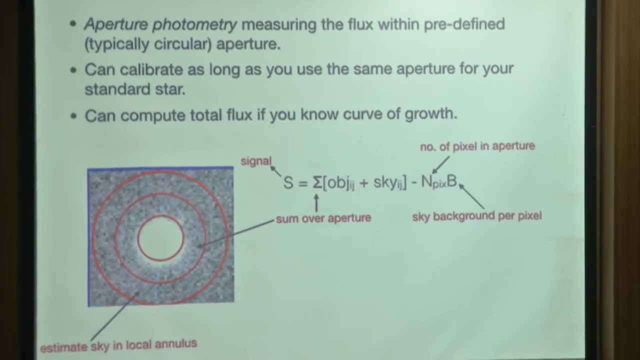 of a aperture. So you need to mention that at what aperture you are measuring this flux. but then you can measure the total fluxes, as long as you know how to measure the total fluxes, and for that you basically plot the curve of growth. So this is, this is what 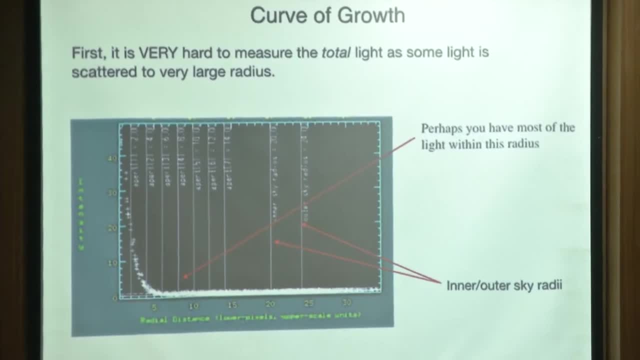 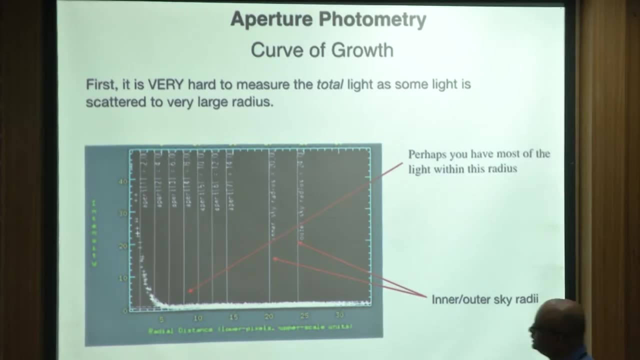 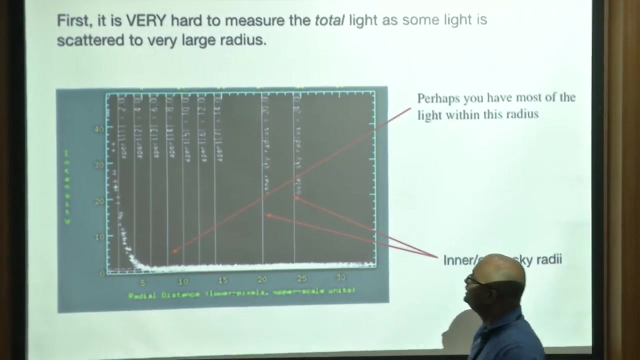 I mean by curve of growth. So what does we do here is that we actually measure the magnitude in concentric apertures and at some point you will see that the magnitude almost has settled in, or the fluxes have settled in at the aperture, and we take that as our aperture. 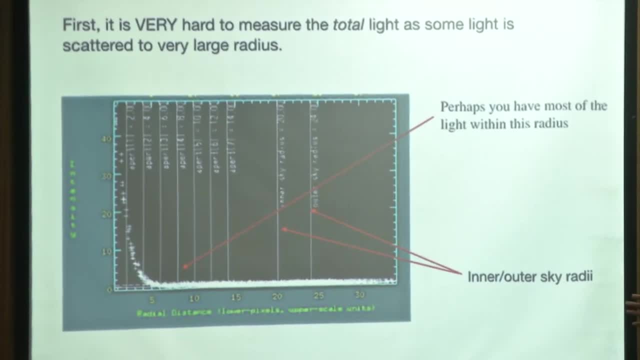 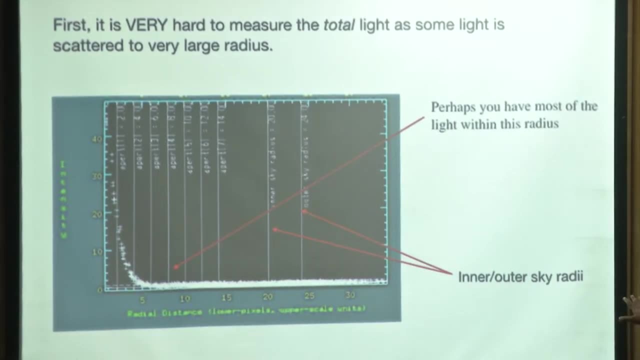 where? So the light within this aperture is? you think that you have the most of the light from that source and then, obviously, there is outer annulus where you can measure the sky and that, basically, will give you the total fluxes from that object and that you can take. 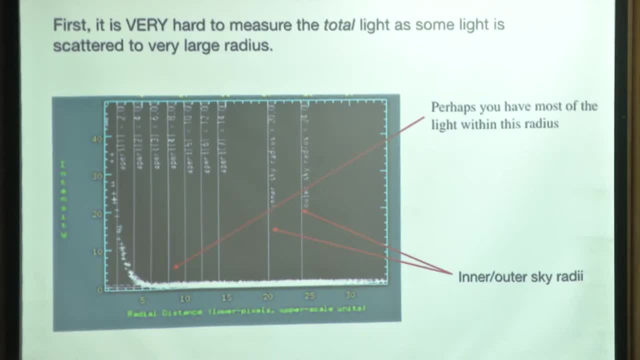 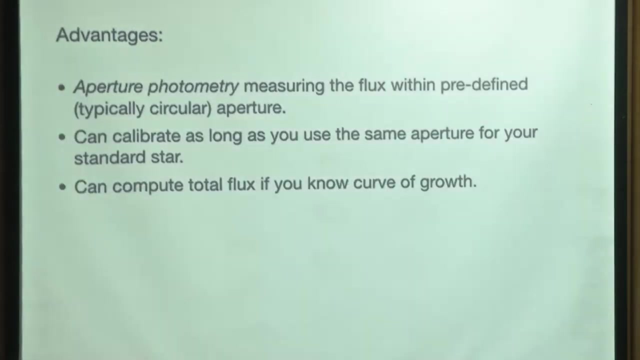 as a total magnitude for a particular target. So this is, this is what we call the curve of growth, where you just plotthe intensity versus aperture radiusthat you have measured in the various apertures. So what are the the advantage? basicallyyou are measuringthe 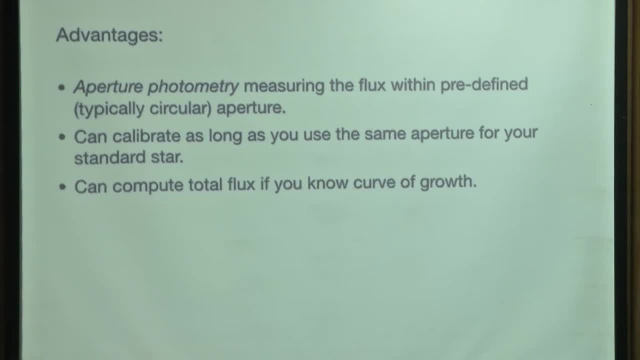 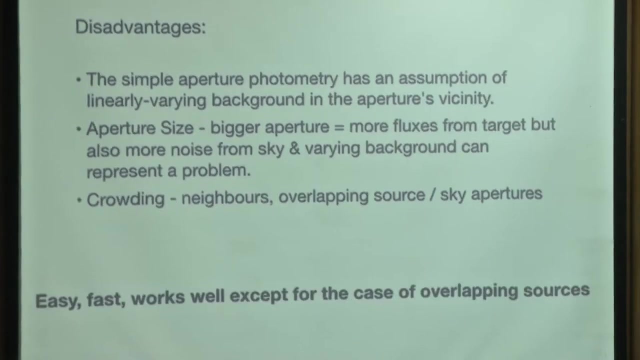 fluxes in a predefined apertureyou can actually calibrate your magnitude, as long as you use the same aperturefor your standard star, and you can compute the total fluxes, if you able able to plot this curve of growth and what are the disadvantages. So here we actually simply. 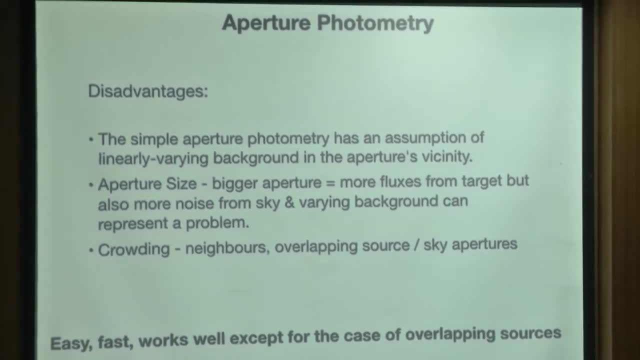 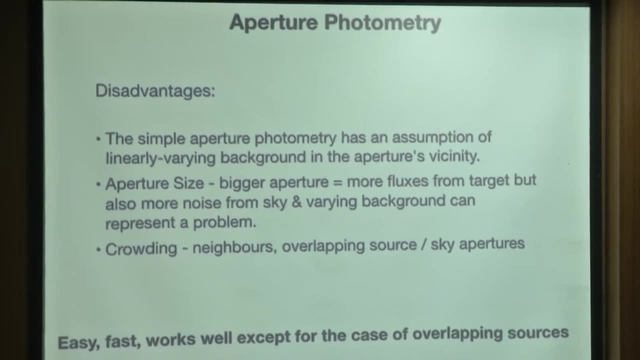 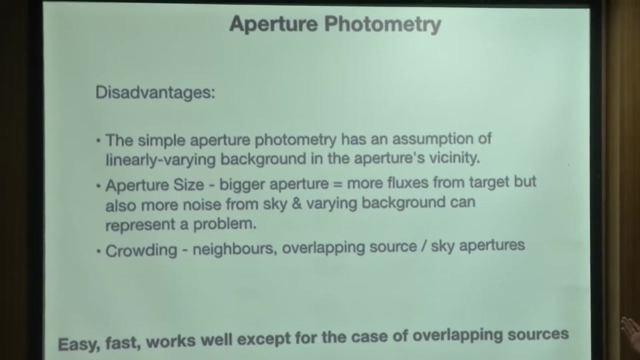 assume that our background is linearly varying in the apertures with vicinity, which might not be the case, and then the biggest disadvantage is the aperture size. So bigger aperture means more flexes from the target, but also the more noise from the sky and the varying background which 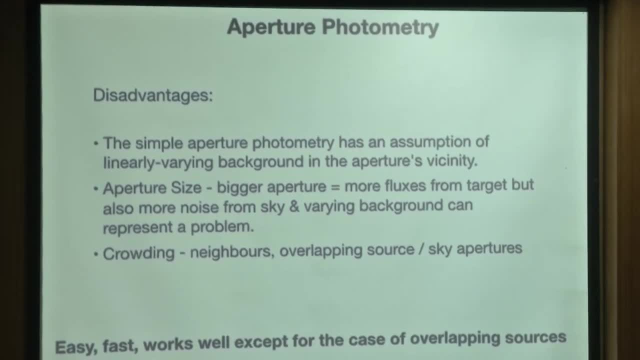 might add a more noise into your flux measurement. and also it does not work when your field is crowded. Crowded means there are a lot of stars and overlapping sources where measuring the sky would be an issue. even the fluxes would be an issue. So this is relatively easy, fast way where you are measuring the fluxes from isolated sources. 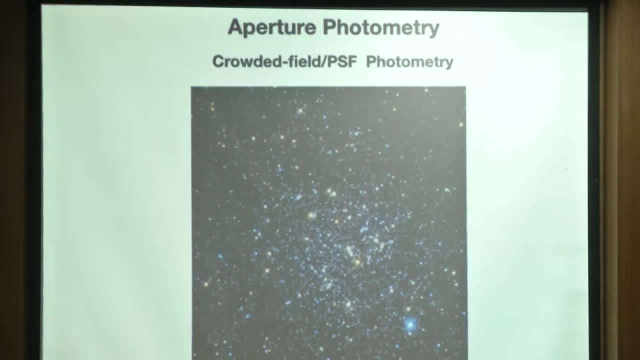 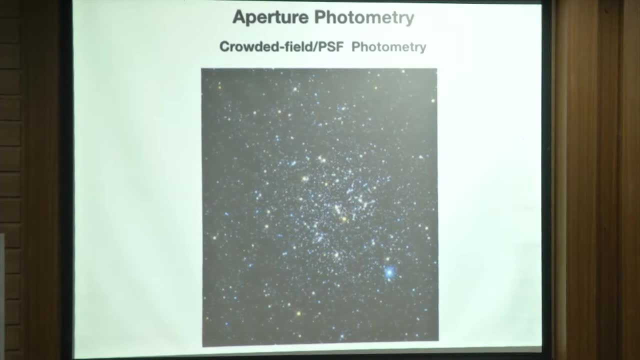 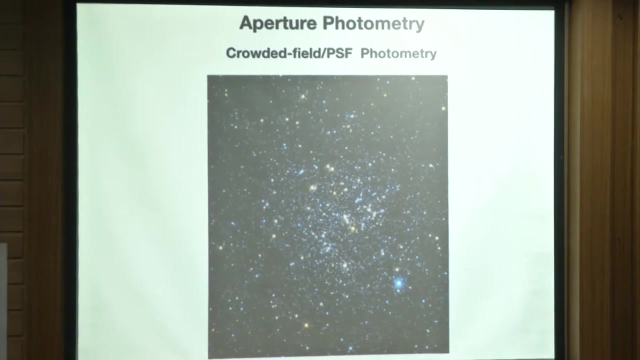 But what happens when you actually go to this kind of image where there are a lot of objects in your frame and you want to measure the fluxes in this crowded field? ok, So what we do here is that, basically, we use a technique called a PSF photometry. ok, So now, as we have discussed, 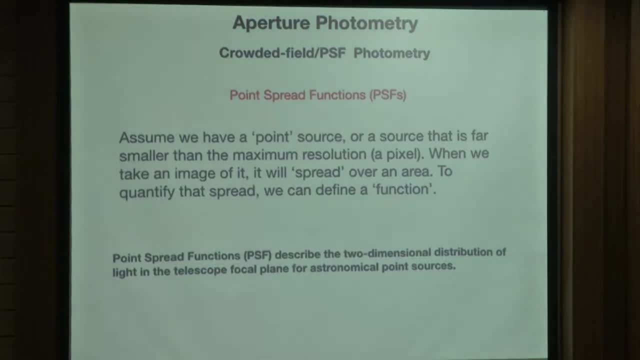 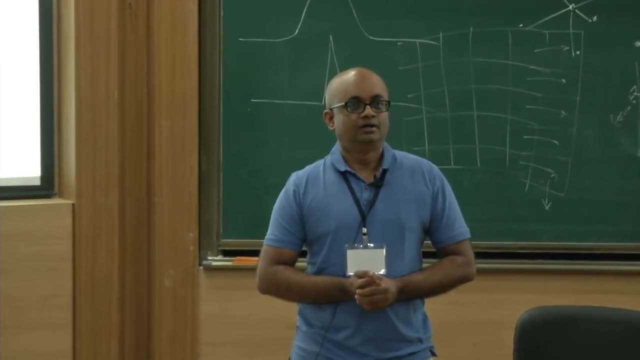 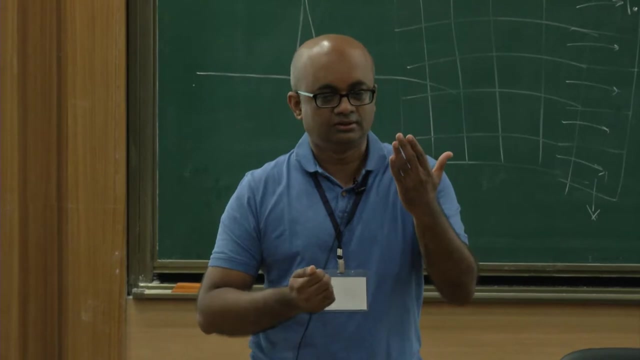 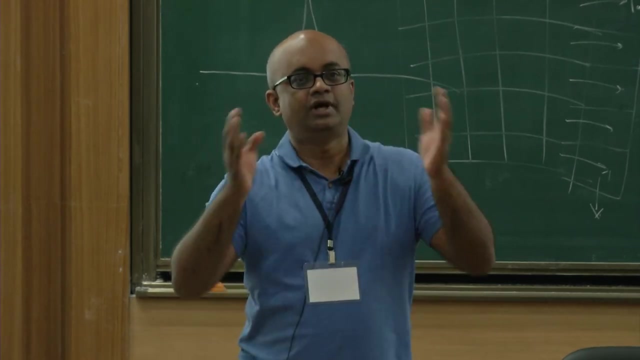 several times and we have used these terms over this. ok, So that actually depends on on your target. ok, So what sort of the image you are seeing at the star is on your image? ok, So if your star PSF is bigger, you have, you have to take a bigger aperture if it is small. 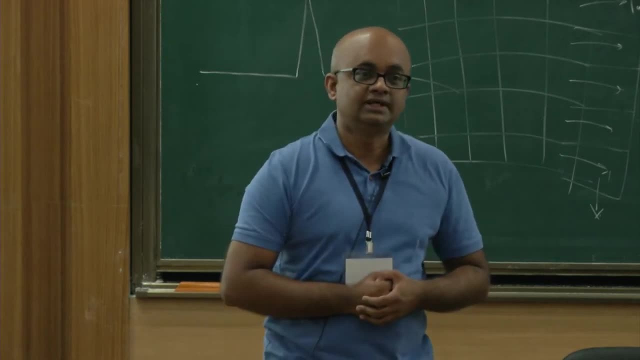 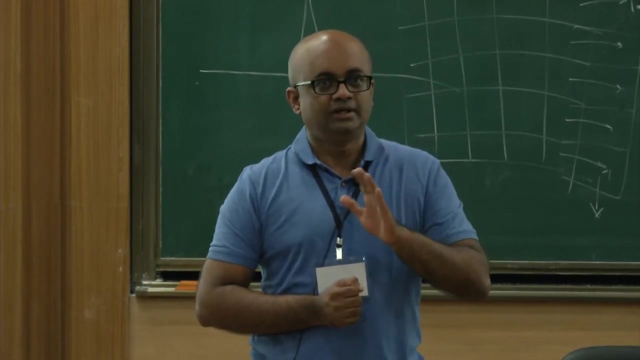 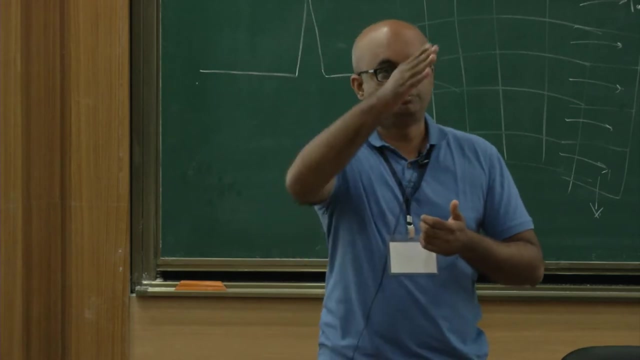 you should take a small aperture. So that is one of the disadvantage of the aperture photometer, Where you need to basically spend some time to decide which aperture you should take. ok, So that is why the curve of growth is helpful, where you plot. 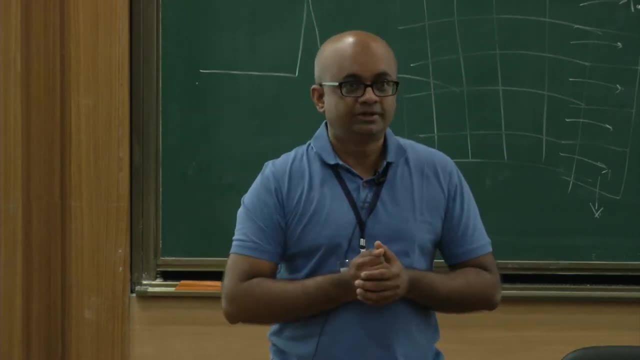 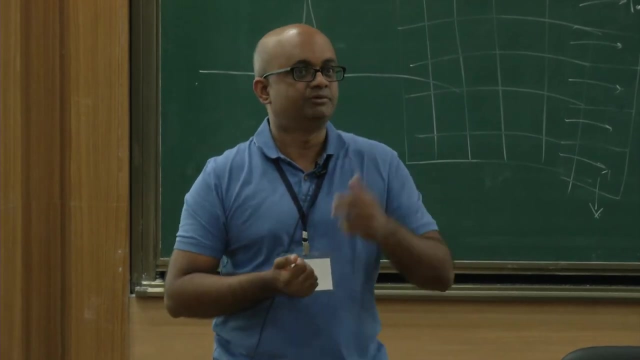 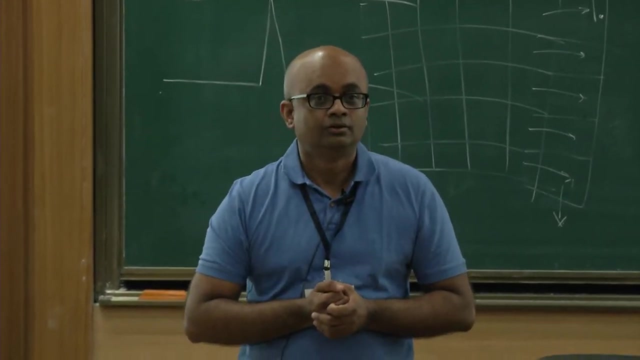 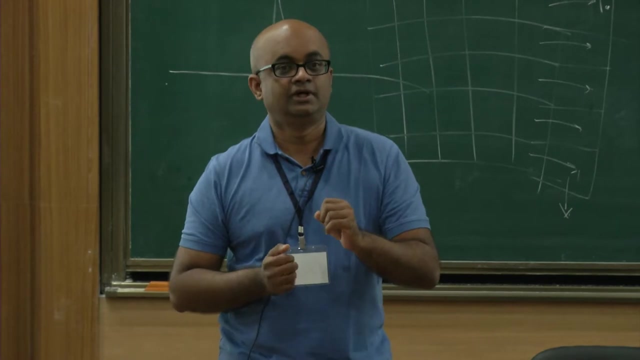 these fluxes at various apertures and then decide: ok, at this point you think that your star contains all the fluxes and that aperture you can take. ok, Sorry, Aperture, Aperture, Aperture. No, So it is a object specific. ok, So it is not about the image. So, for example, if your 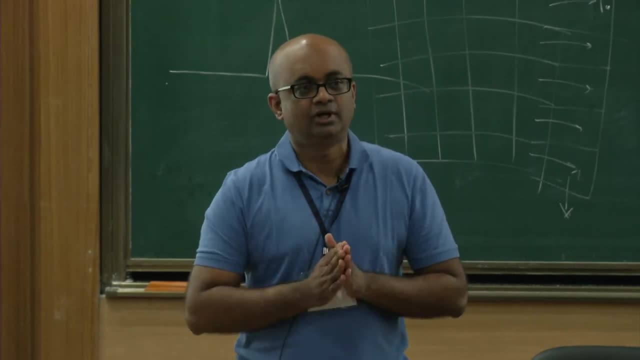 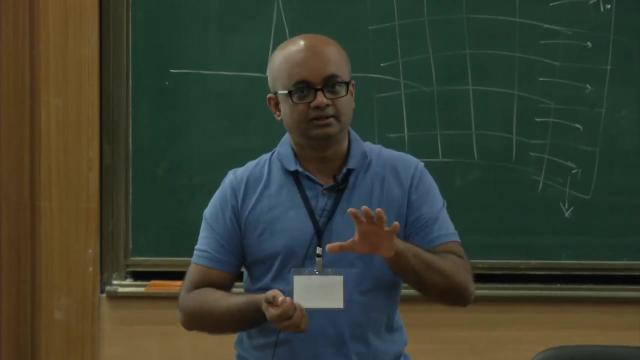 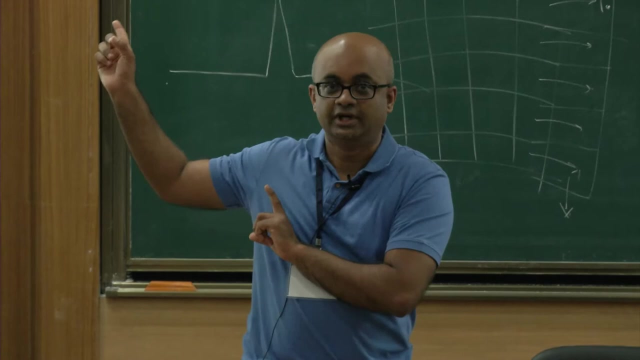 image contains few isolated stars and it depends on how your star, whether it is bright or pink, ok, So, so, so that is where you need to basically decide. it is how and which aperture you can use. So that is another disadvantage, ok, So that is why we actually, most of the time, 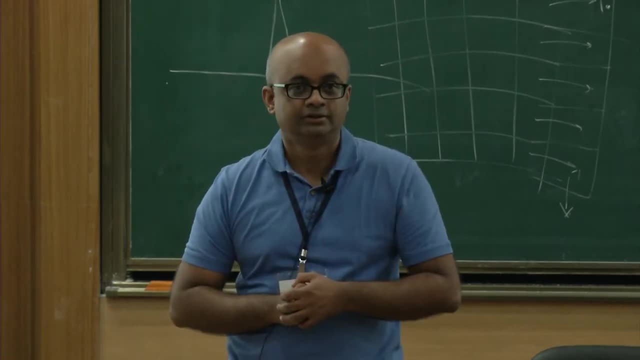 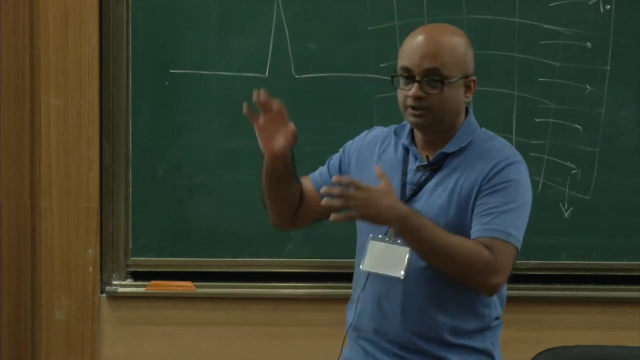 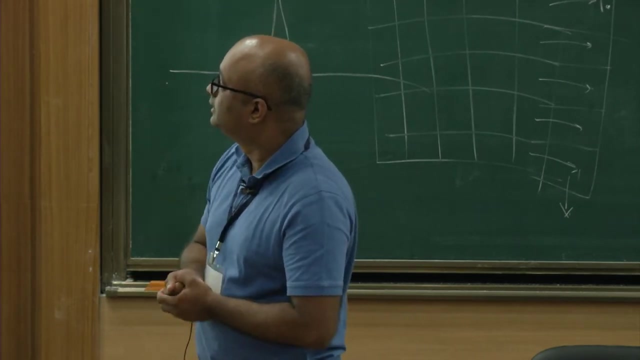 end up using a PSF photometer. So so so you basically know what, what, why we actually talk about the PSF. ok, So you know that at at a telescope focal plane, your point source, like a stars, they are not exactly a point source. 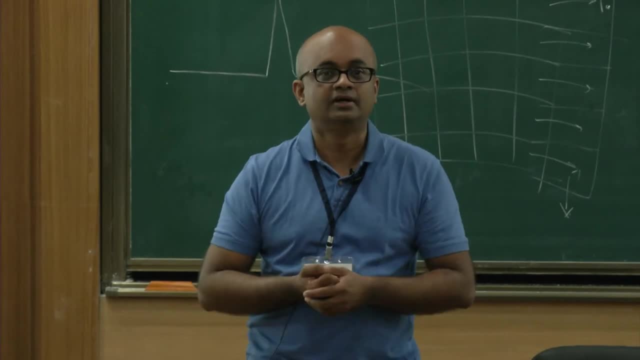 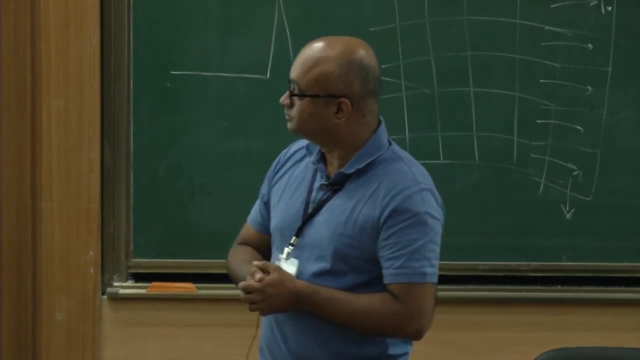 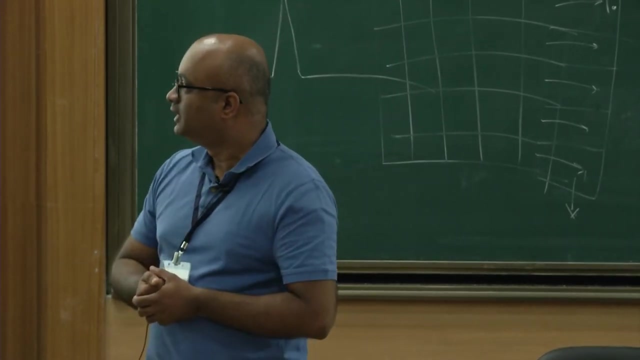 So they appear as a, as a circular disc. ok, And that is that is what ah, that is what we called ah of PSF, and we use obviously some mathematical functions to define this two dimensional distribution, ah of of this, this ah spread of light and 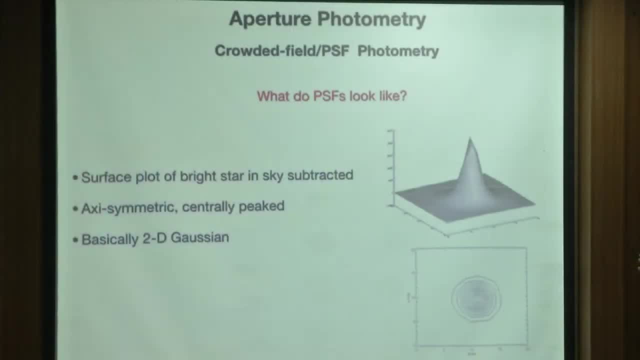 that is what we called the point spread function. So typically, when you ah, do some sort of image examination, ah, you can plot these kind of a surface plot ah, where the x, ah and y is your, the plane, ah, and then then the z axis, you can see the, the intensity and, as you can. 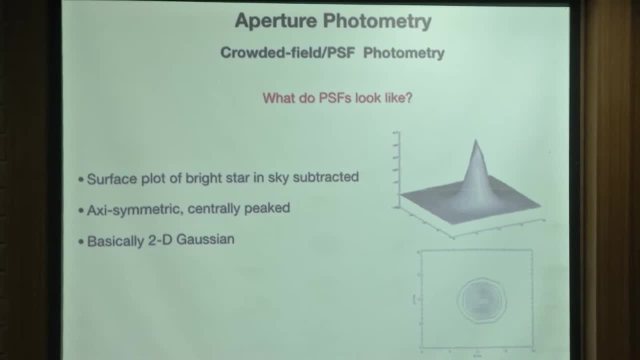 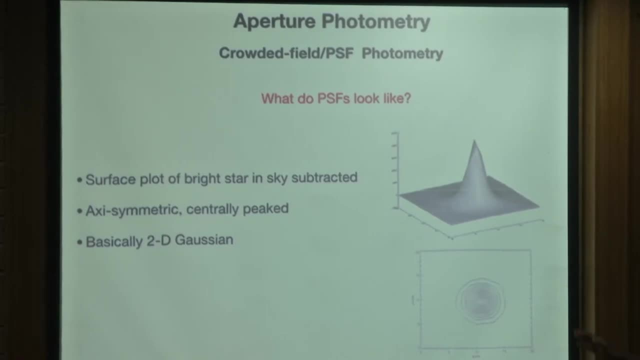 see that, ah, this ah spread, ah, it is. you can well, ah well, ah, represent this by ah, very, ah, very ah, easily by ah two, ah, dimension, ah, Gaussian function, ok, ah, So so this is, this is for ah, ah, ah, the typical PSF that look like for a, for a star, ah and ah generally. 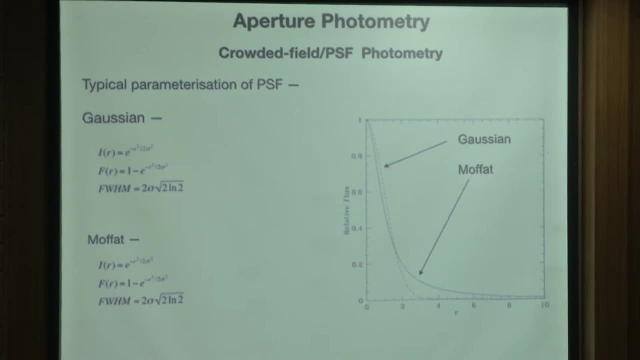 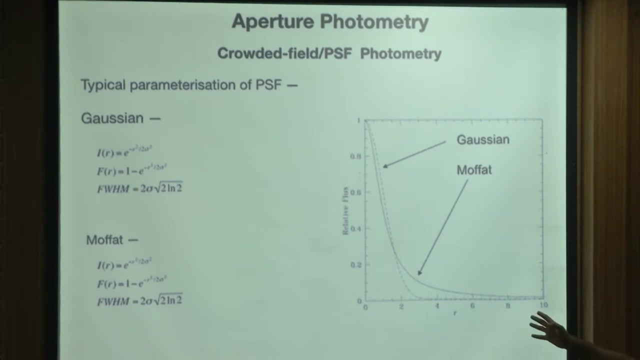 in estrus, So in astronomy, we use ah, ah these two functions, ah to parameterize, ah the PSF, ah, So ah, in most of the cases we use Gaussian ah, which ah the parameters. you can define the using these formulations. or, in many ah cases, ah, we also use the Moffett function and these 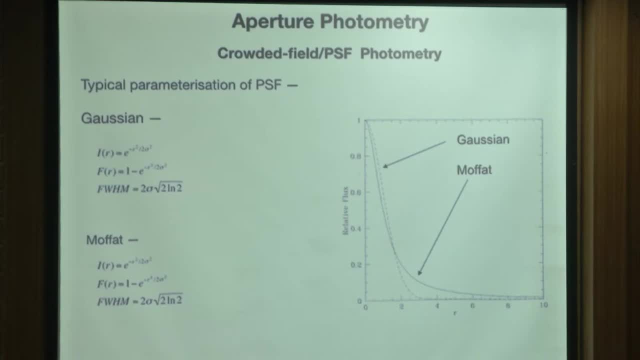 are the typical ah ah way that you can represent, ah, these functions. oh, ok, sorry, I will change this. So this, probably I have used the same image, ah, so these are the image. ah, ah, ah, sorry about this. So, ah, will show at some point what the Moffett function is. ok. 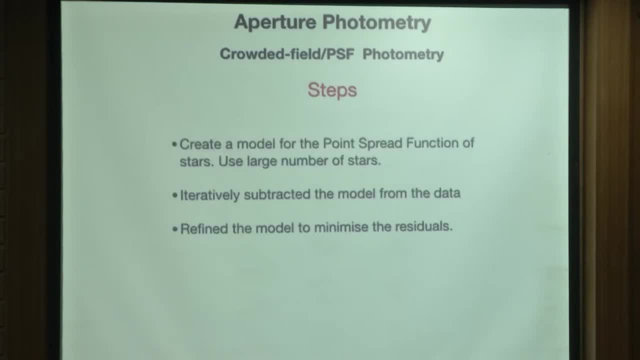 So what basically? we do, ah, in this PSF photometry. so we basically create a model for a point spread function of a star, ok, Ah. and then, ah, to do, ah, get good model. we use a large number of stars, Ah, Ok. 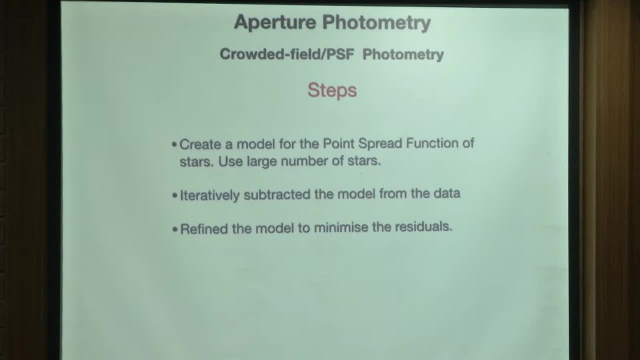 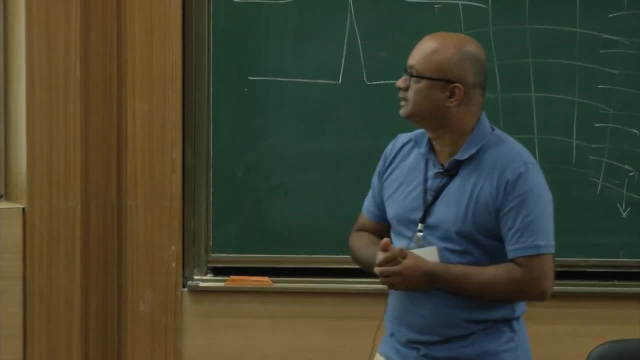 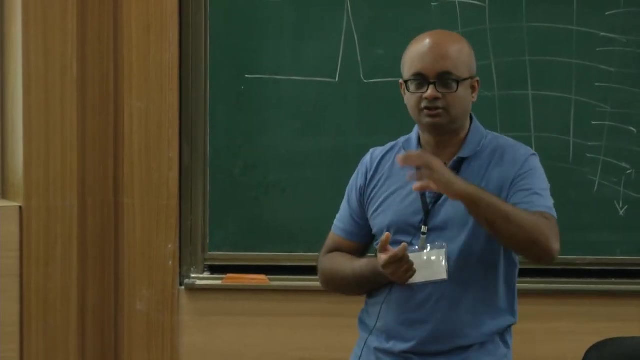 and then we iteratively subtract the models from the data that we have in form of stars, and then we actually again redefine the models to minimize the residuals. So what happens is that when you do it iteratively, you will have for each of your object a PSF. 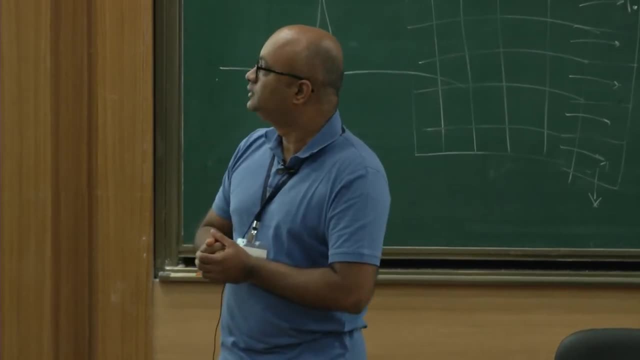 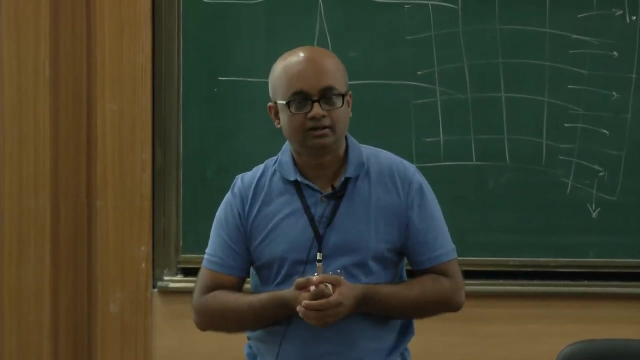 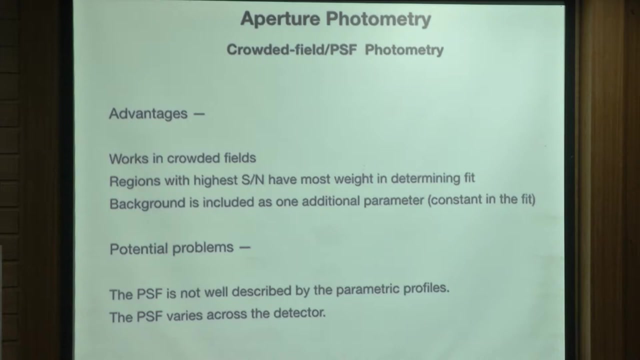 and that you can define in terms of sigma and some radius, and then you can use that radius to get to define as aperture and get the flux in that aperture. ok, So this is: this works very well in crowded fields and it also uses a sort of a weighting. 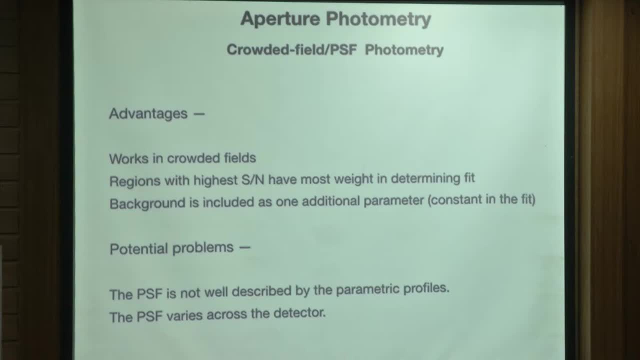 scheme where the regions with the highest signal to noise ratio have get the most weight, and then you can also include the background in this fit so that you do not need to worry about the background. But there are some potential features Issues with that. when your PSF is not well defined, then obviously you have to be bit. 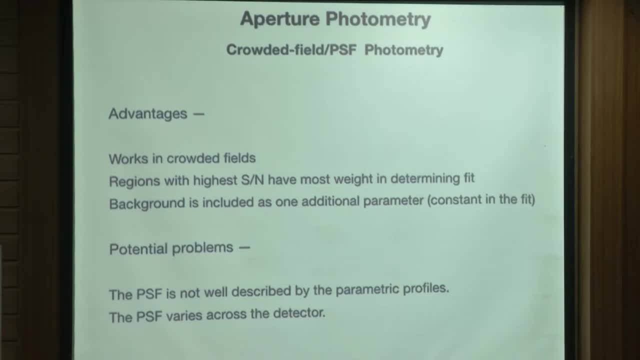 careful and then in some cases, when we typically talk about the large field, your PSF can vary across the detector, So you need to also take care of that and how, basically, you are going to use the PSF photometry. Ok, And I will just end this. 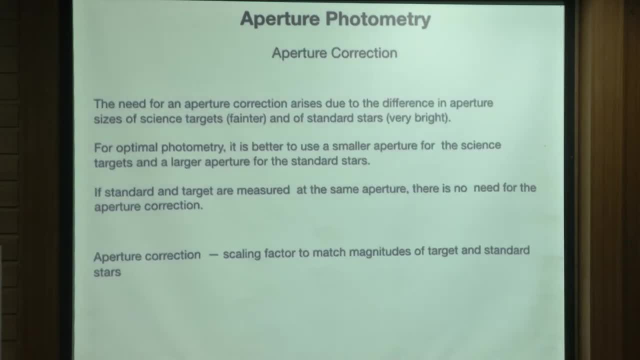 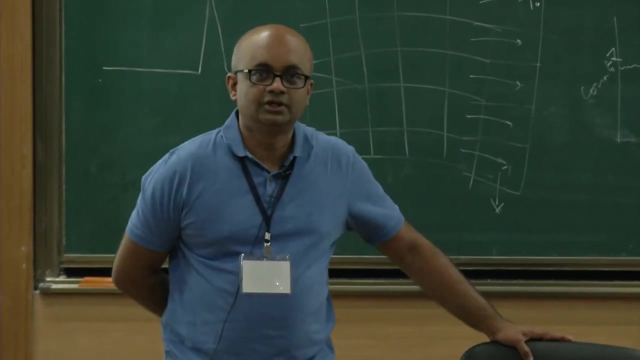 Ok, So let us start with one thing, which we normally call the aperture correction. ok, So what the aperture correction is? it is basically a scaling factor to match the magnitudes of a target and the standard stars. ok, So what happens is that sometimes you do not know what apertures has been used to measure. 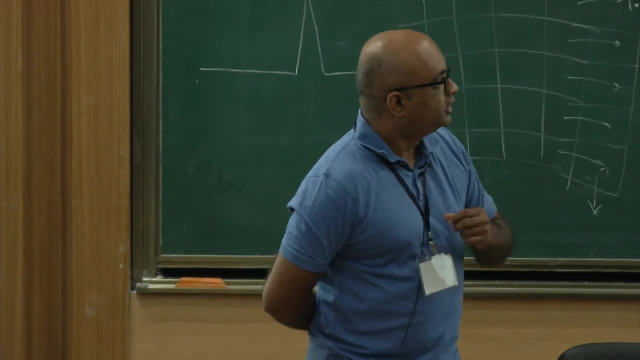 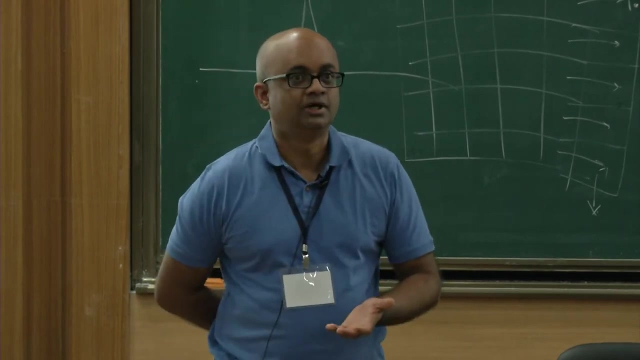 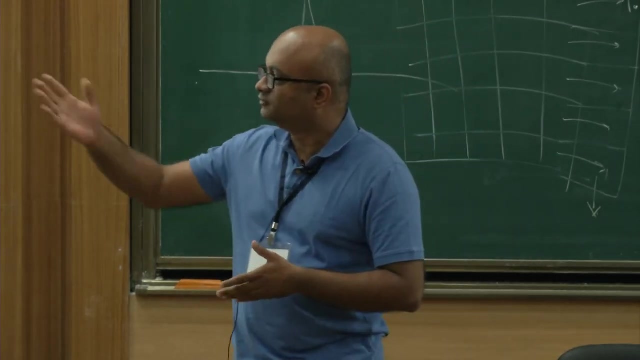 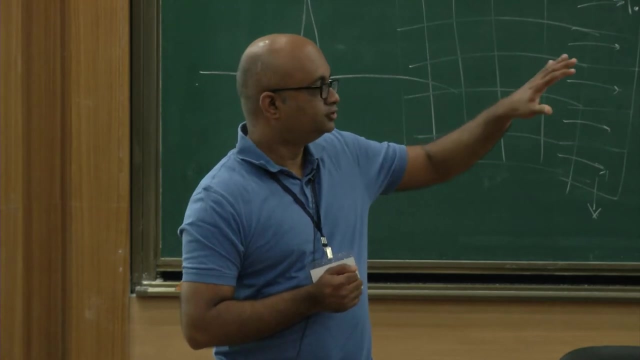 the magnitudes of your standard stars, but you definitely know that, what sort of apertures you are using in in your, Ok, Your image for your stars. So, basically, then, you need to actually use a technique which we call aperture, aperture corrections, to match these magnitudes and find out the scaling factor so that you can. 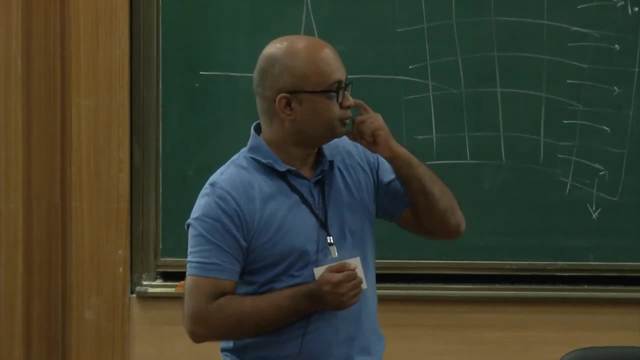 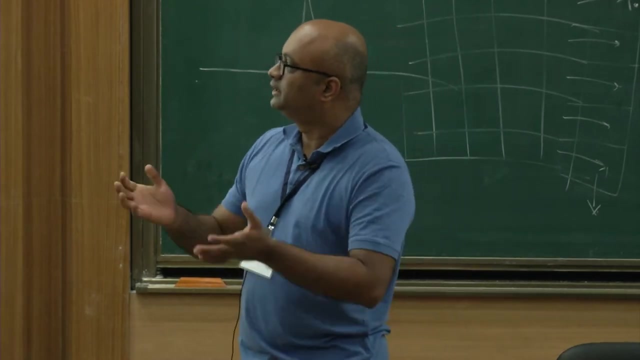 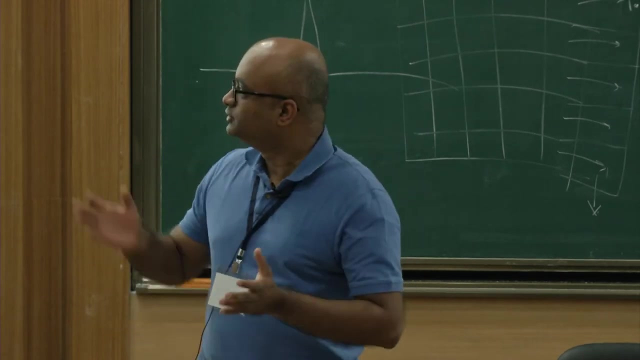 apply that scaling factor to the magnitude in addition to a zero points. But if you have a sort of a, you measure the, you know that your standard stars and the targeted stars, So you can use the same apertures to measure the, the fluxes and its magnitude. 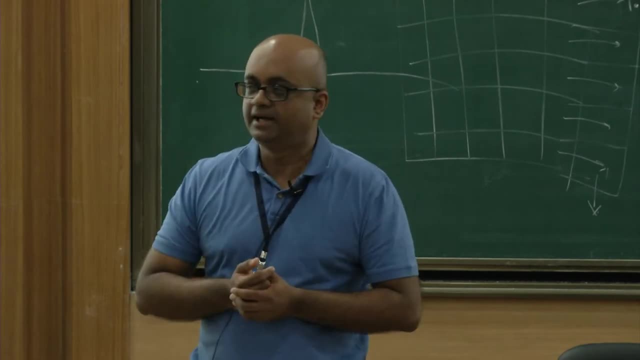 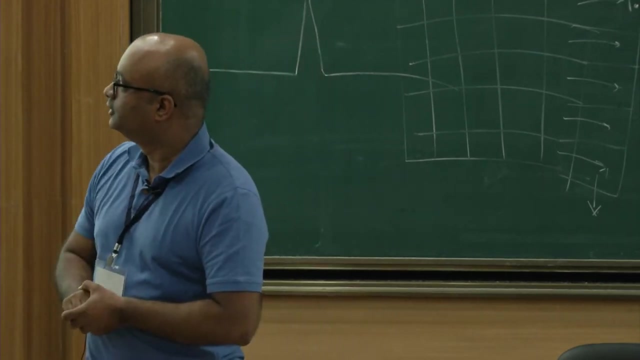 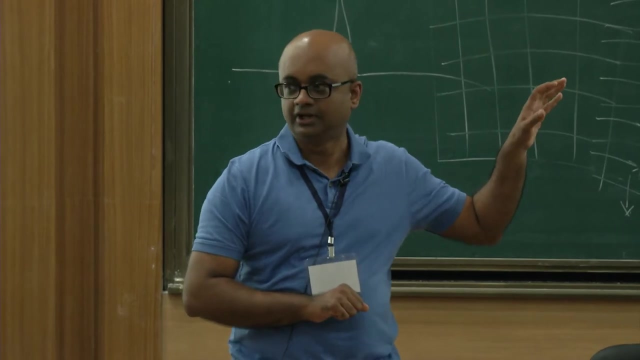 So you do not need to basically do this and you can apply the same magnitude which we basically use as a zero point for for getting your your targets magnitude, and then you do not need to apply the aperture correction. ok, So you will get to know about all this terms when you actually follow various steps of 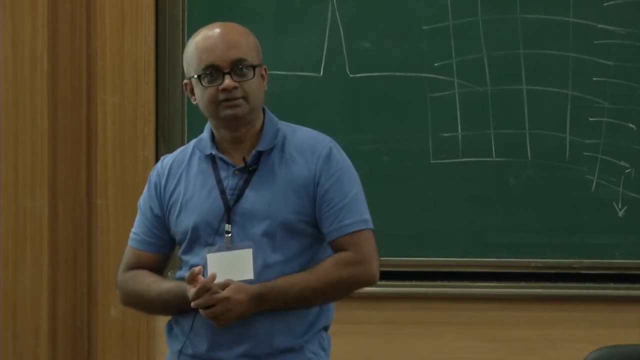 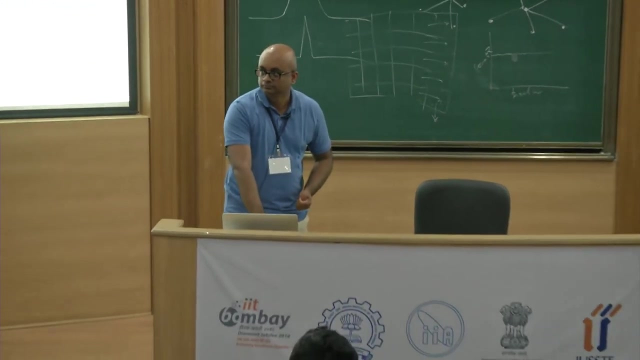 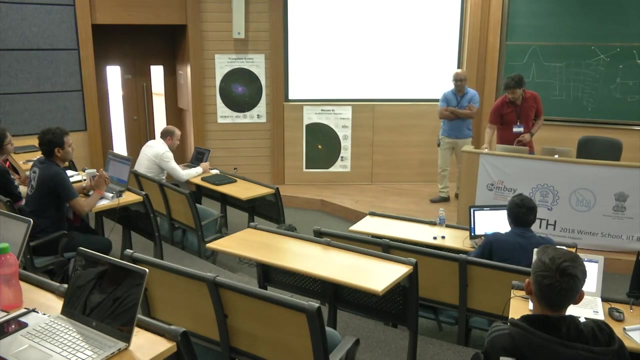 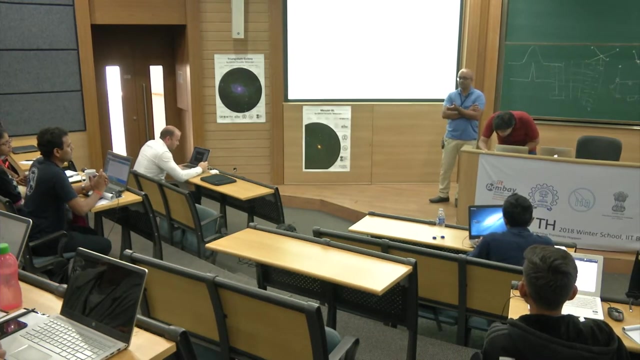 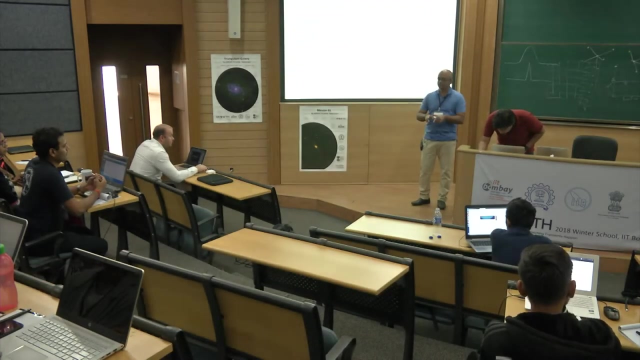 the tutorials that we will discuss. Ok, So we will stop here. Question: Well, what happens normally is that that that is why you use a, a large number of stars. ok, So so to actually get to know that threshold. ok, So what you should get is that a, a sort of a PSF model which exactly represents the whatever. 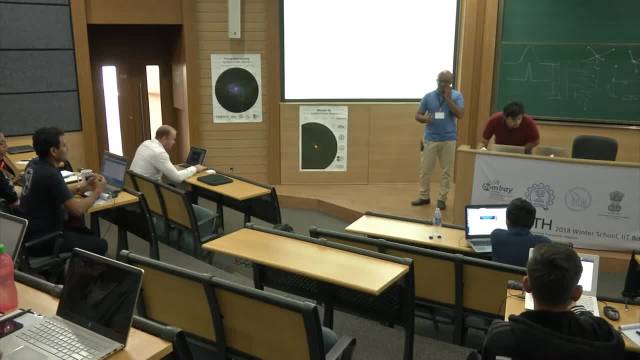 sort of a sources are there in your images. okay, So idea is that to use a large number of stars to get to know which model exactly works best, for both brighter and the presenter sources, Of course, when your star is either much brighter or much fainter. so that thing. 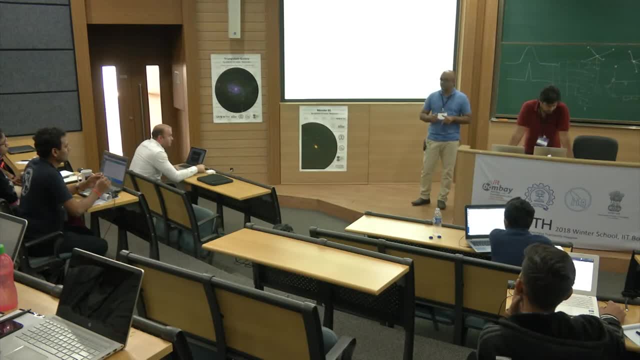 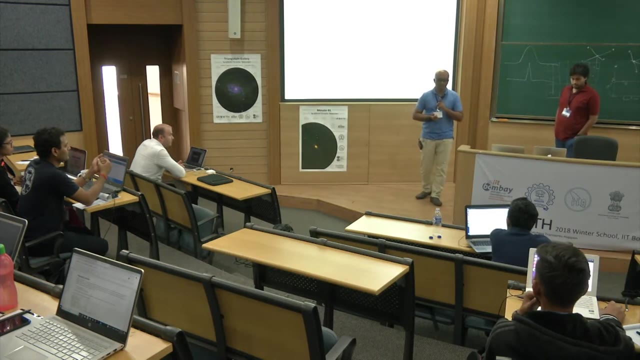 will fail. okay, But it will. it generally works well for a well defined well where you can able to avoid all these extreme points. basically, yeah, I guess that I exactly don't know, I haven't worked on the the very extensively on the. 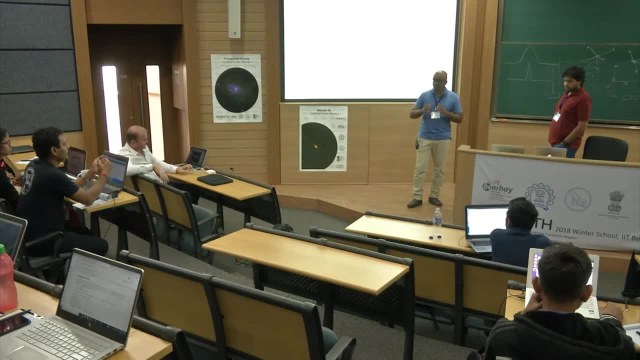 global clusters actually. So obviously again, I said that you need to basically worry about what sort of a PSF you have for your in the field of where the global clusters are, So what the globular cluster is okay, And then then you need to compute the model according. 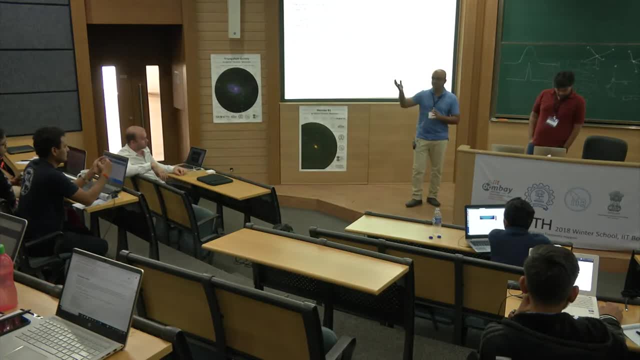 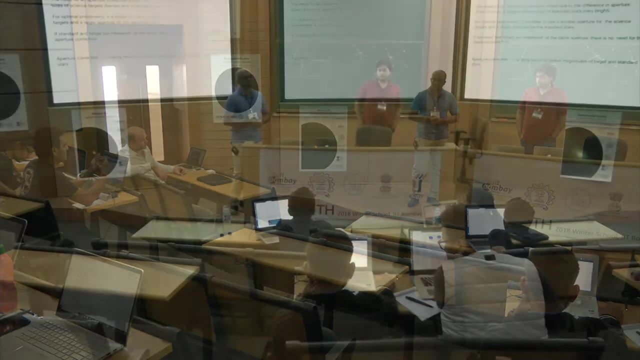 to that, okay. So if your standard star, which is far away, is much brighter, obviously you cannot use that, okay. So giving some number is obviously a bit difficult. You have to work out when you see the image, which you will do in the tutorial. Do we use photometry? to measure a redshift. It is possible in some very special cases. yes, It is possible in some very special cases for really high redshift. Yes, there is a technique known as the Lyman break. The idea is that if you have very strong absorption, short words of some wavelength. 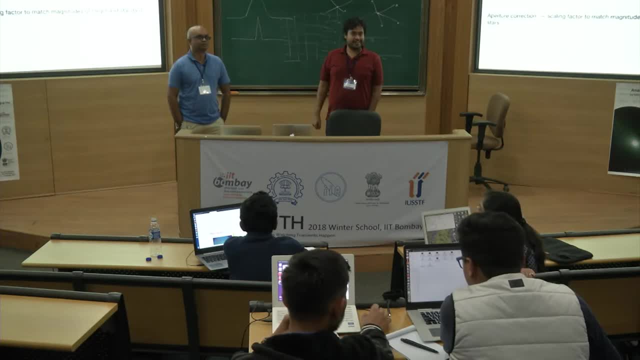 you would see the photometric flux cut off And that gives you some handle of the redshift, but it's still not. it's not as good as a spectroscopic redshift that we have, So it's basically not a good way to measure a redshift. 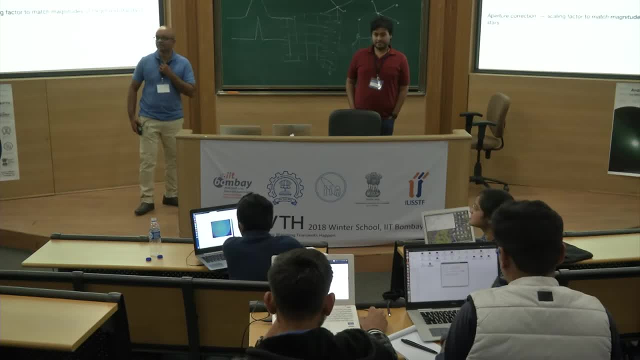 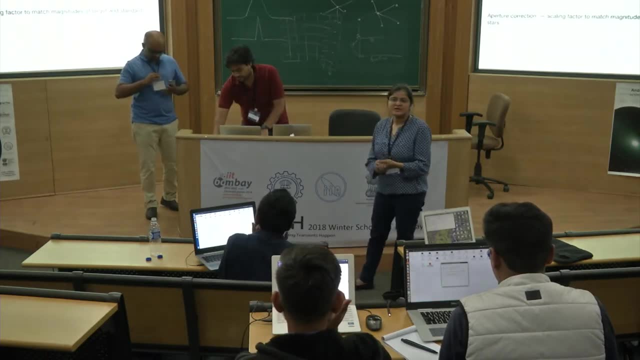 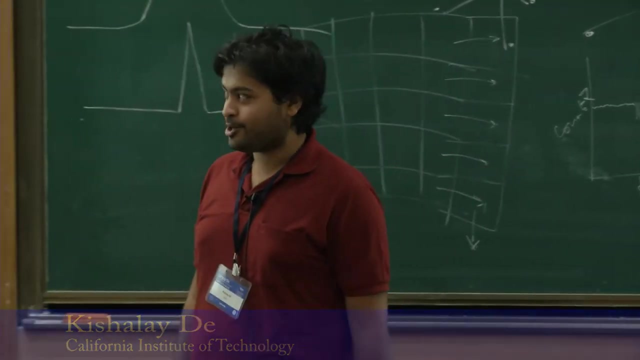 Or no way to measure a redshift. okay, Can talk Right. So, as you already heard in the lecture, there are two ways of doing photometry. One is aperture photometry, the other is PSF photometry. We will be only doing point sources today. 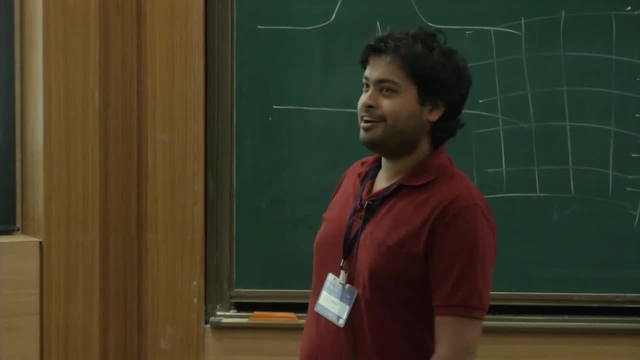 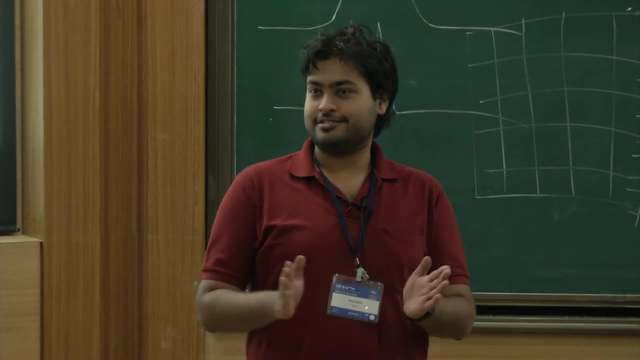 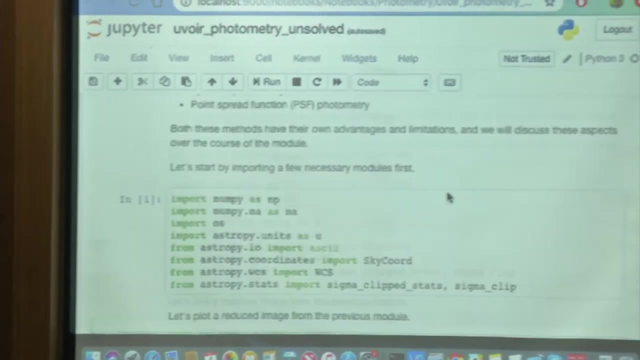 Galaxies and extended sources are totally different. lecture in itself, Right. So if okay, how many of you have the notebook up and open? Okay, That looks reasonable. Okay, Perfect, Okay, Right, So we can start walking through the steps. So, as before, just. 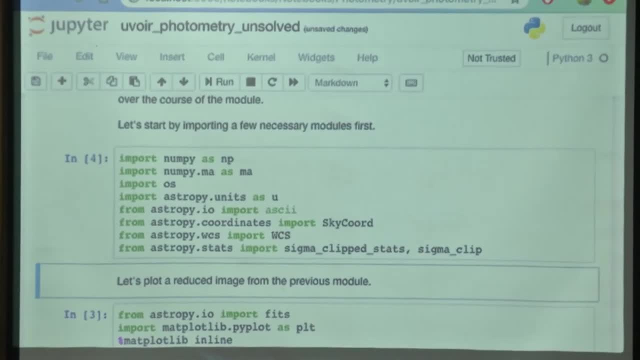 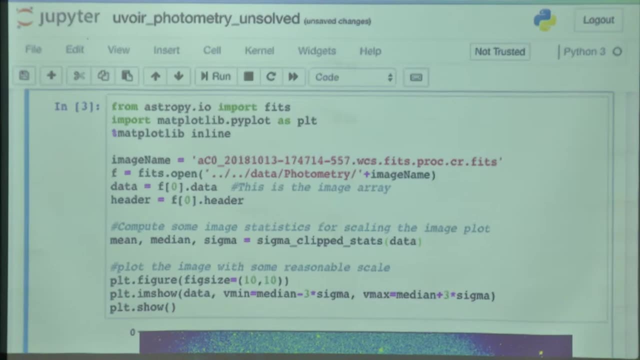 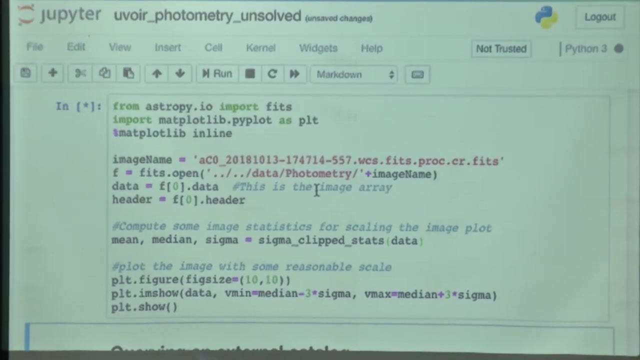 import a few modules that we need. Okay, And I wanted to start with just just one single reduced image that we created in the last module. So if you just run this cell, you should see an image come up. Oh, you don't Just add it? I mean, I don't think it makes a difference, but we'll add. 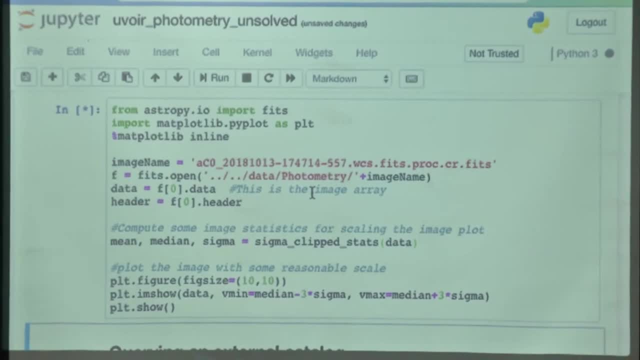 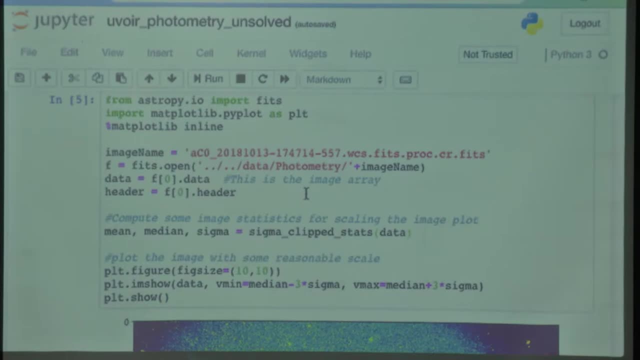 it here And I think for this notebook, the if you are using the Docker, No, it's, it's fixed on the detector coordinates, It's not on the sky. So, Yes, Yes, You've shifted the detector a bit. with respect to the sky, Then, 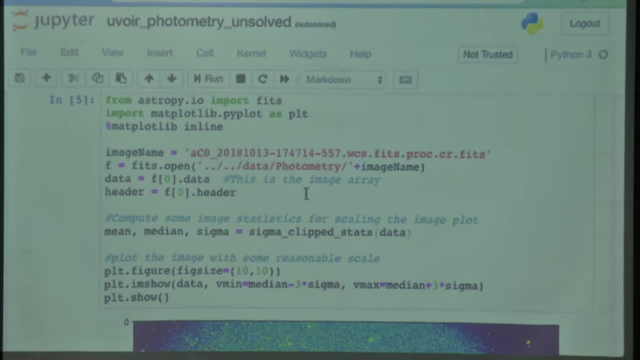 Yes, Yes, You're doing that. Yes, Yes, Oh, It's like a little bit, then. and if you stack them, then, because the bad column is falling on different locations in the sky, everything gets lost. that is the way you would want to do this. ok, ok, ok, perfect. 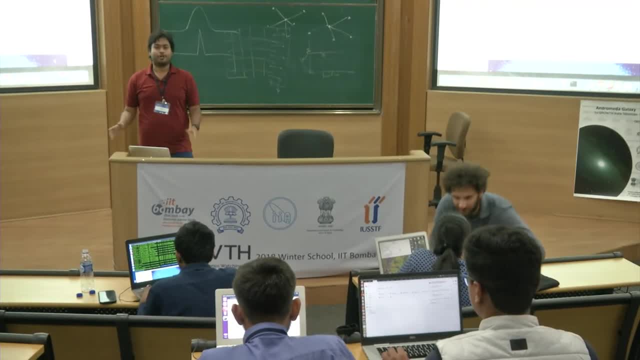 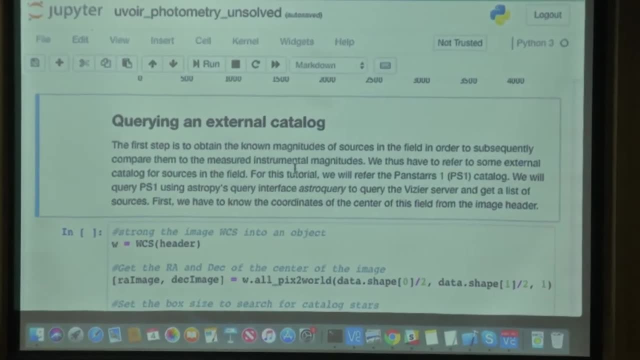 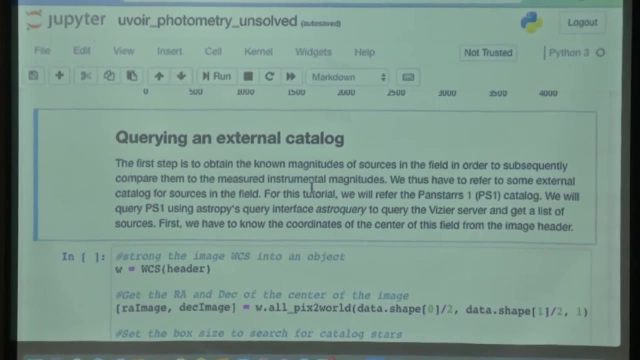 So this is a reduced image from the previous module and we will be doing photometry on this image. ok, So the general procedure in photometry is to is to query an external catalog. So the idea is that, you know, today there are sky surveys that have actually derived magnitudes. 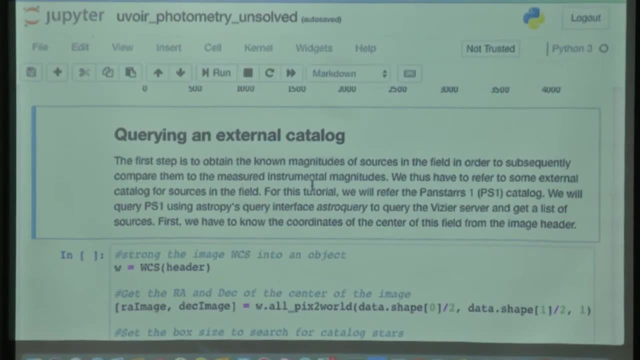 for most of the sky, and the idea is that you query an external catalog. you ask the question: these are the stars inside my field and what are the magnitudes of the stars that are there inside the field? You want to compare those external catalog magnitudes to the magnitudes. 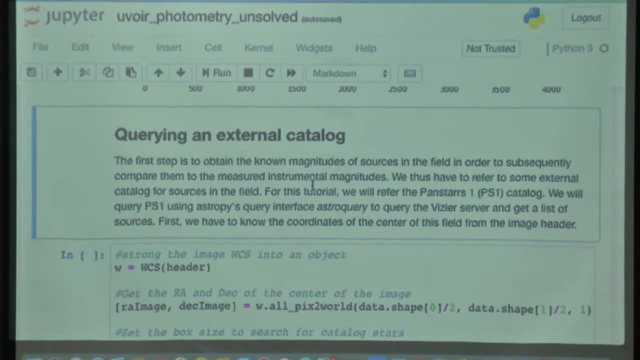 that you actually measure from the image, and that is basically what you will do here. So the first step in that is active is actually to query an external catalog. Ok, In this case, for this field, we'll be querying: what is a catalog from the Pan-STARRS survey? 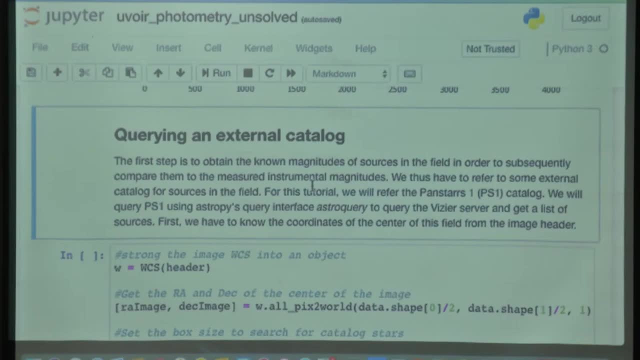 So the Pan-STARRS is an all-sky, Is it all-sky, Mansi? Is Pan-STARRS all-sky? Yeah, Yeah, So it's almost all-sky. It's an all-sky survey that has. 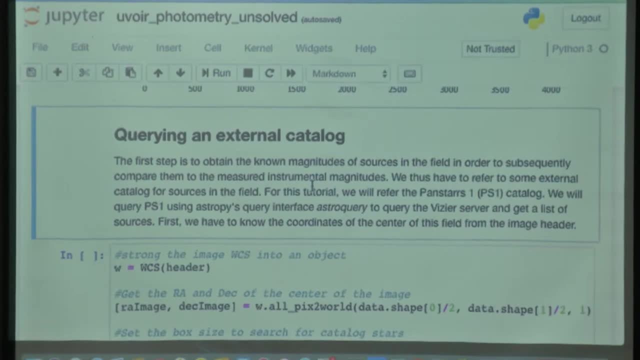 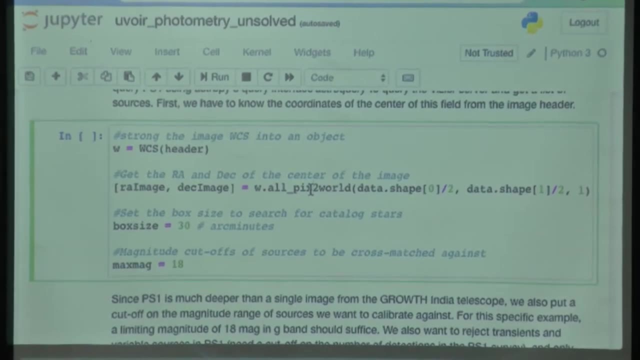 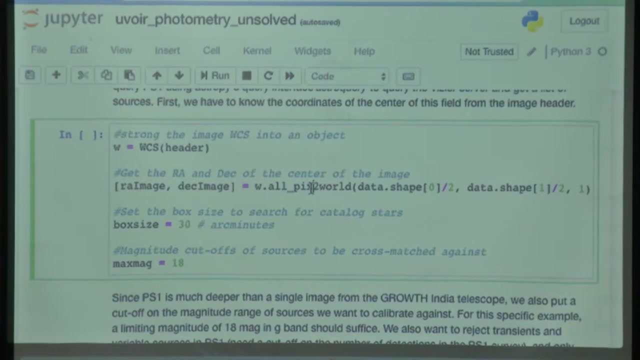 well-calibrated magnitudes for stars in most part of the sky, And what we'll do here is first, so the image that we have here already has the astrometry derived on it, And in order to download an external catalog, you have to tell Pan-STARRS that I. 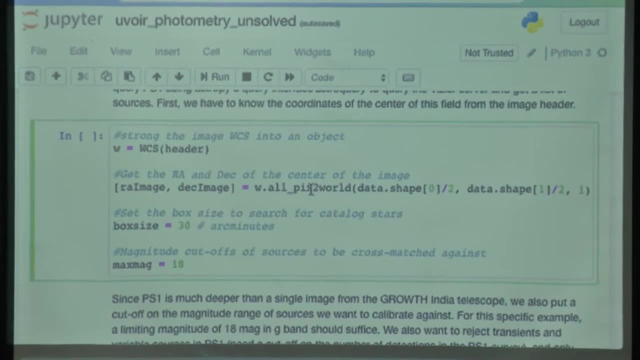 want stars that are within some radius of my field, And that's why we will first read in what is the location of the image. So this is what WCS is. So WCS stands for World Coordinate System. It's a term that you'll come across very frequently in image reduction. 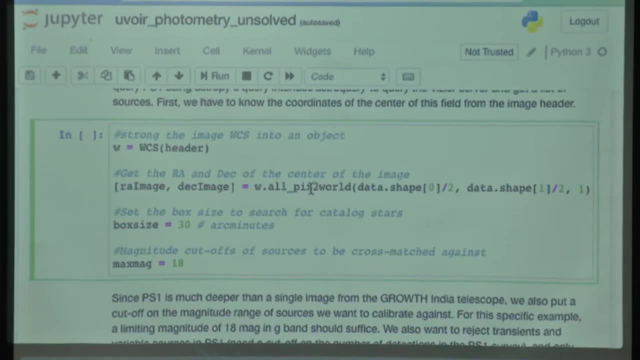 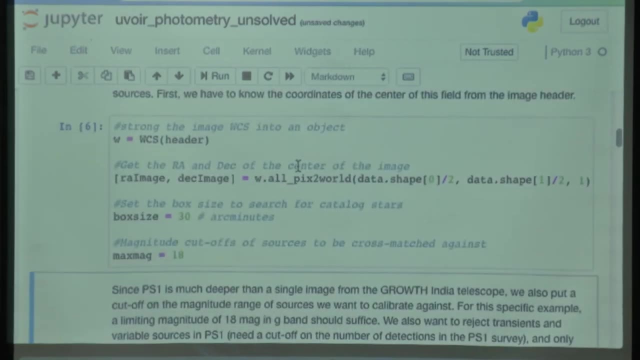 WCS effectively tells you what is the location of the image in the sky. So if you just go ahead and run that, what we're doing here is that we are reading the center coordinates of the image, So we are reading the WCS of the image. 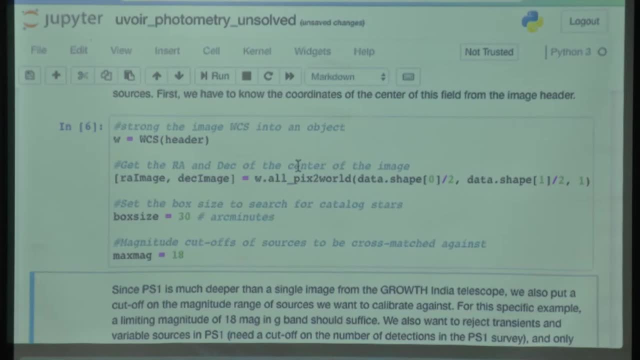 reading what is the center coordinate of the image, and we are setting the size of the radius, So we are querying all stars that are within 30 arc minutes of the center of the image, And then we are also setting what is the maximum magnitude. 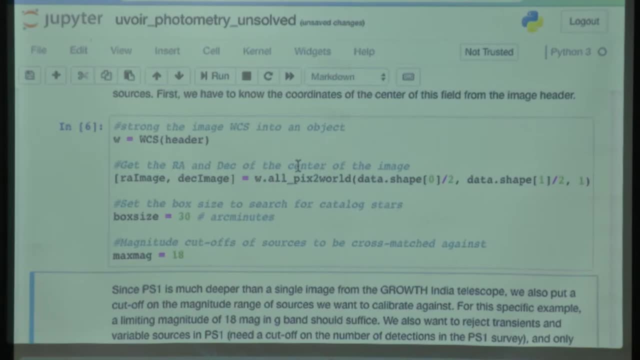 So recall that the larger the magnitude, the fainter the source. So what we're doing here is that we're asking to return stars which are brighter than 18th magnitude, because that's about the typical sensitivity you get in a short exposure. 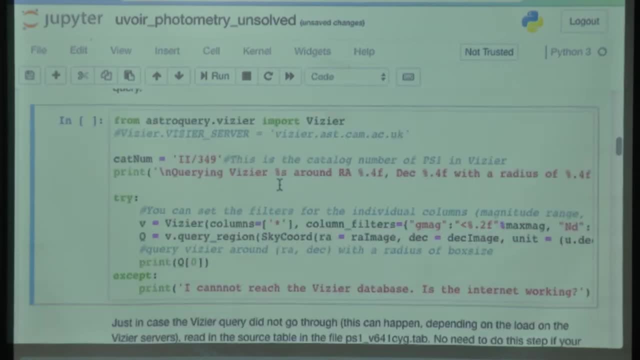 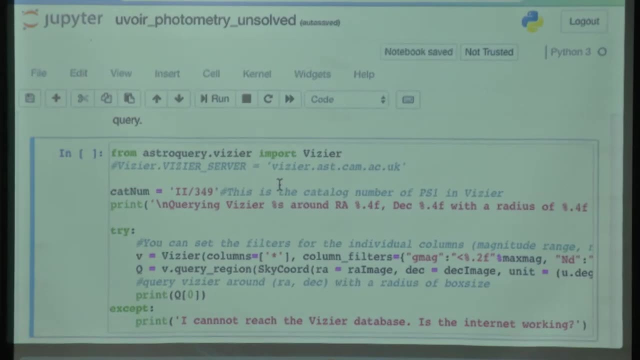 So let's see. Okay, So the next step is to use the AstroPies interface for querying. It's called AstroQuery And this is where we'll be querying the Vizier catalog. So the Vizier is again you can look up. 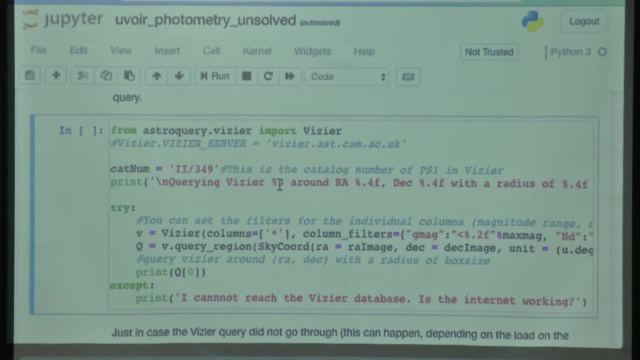 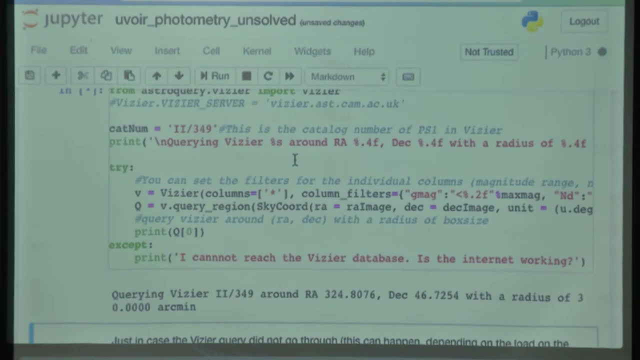 Google Vizier. It's just a database of lots of different surveys. It has catalog magnitudes for all different kinds of objects that are recorded by surveys. So you just run this shell. can take a bit of time because it's actually downloading a fair bit of data. 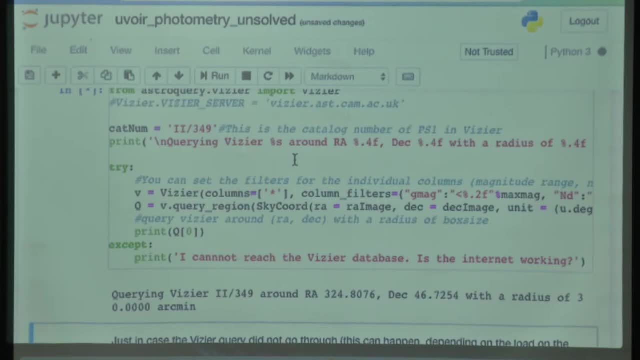 So what you're doing here is that we are querying pan-stars around a right ascension of this declination of this, with a radius of- so sorry, right ascension declination and radius of 30 arcminutes. This is V641 signi, which I think is a Cepheid Cepheid variable. 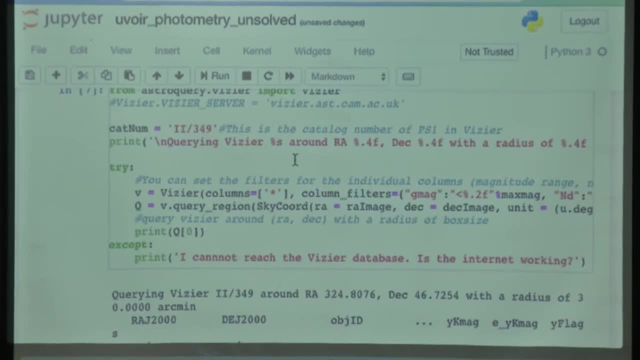 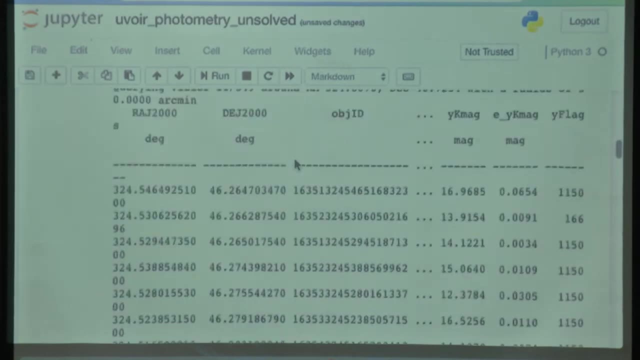 Yeah, so this is the source that you will be working on in the light curve module. It's just a field that has an interesting variable star in it. Okay, so if that query worked, you should see a list of stars being displayed. You'll have the RA of the stars, you'll have the deck of the stars and 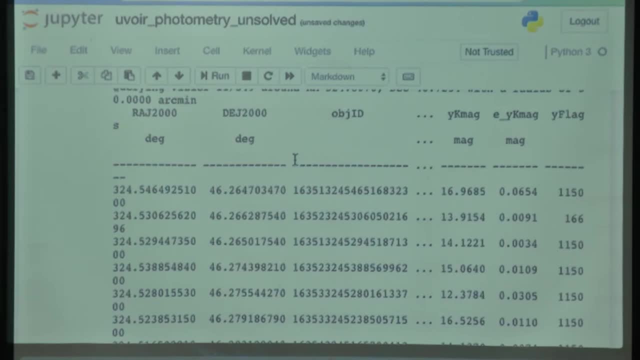 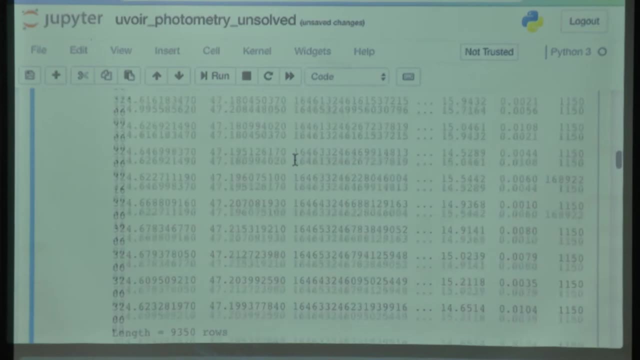 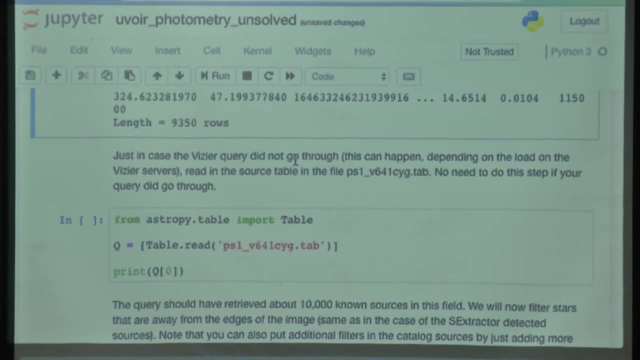 all sorts of magnitudes That are returned. Okay, perfect, Yes, okay, Right, So I had. I just had this in case the internet did not work, but it looks like it worked, So you don't need to. don't don't run this cell. do not run this cell. 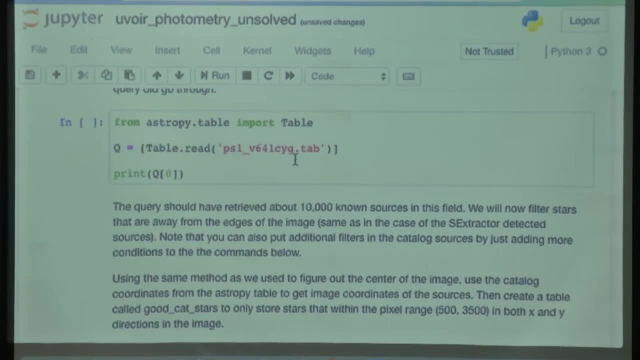 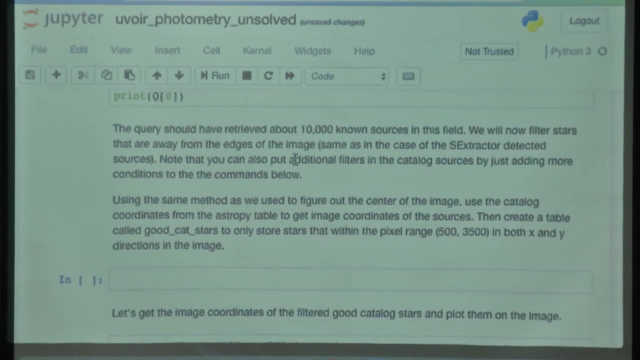 Because you'll get an error and that might scare you. so, yes, yes, Yes, it will Right. what do I have? Yes, so let's see. the next step is to so this. what this catalog returned is a list of stars within 30 arcminutes of the center of the image. 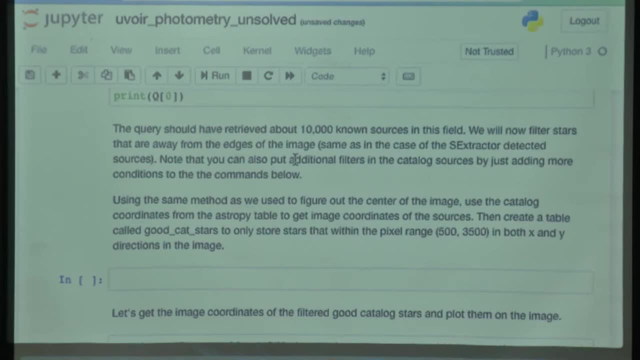 For photometric calibrations, you only want to select stars that are within some region of the center of the image, Where the idea is that you don't want to select stars that are in the wing netted region, because the sensitivity is really weird over there. So 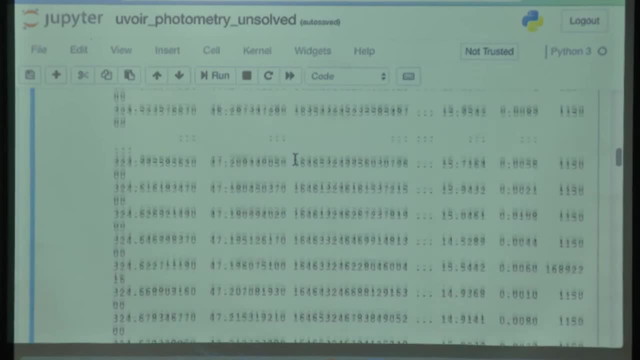 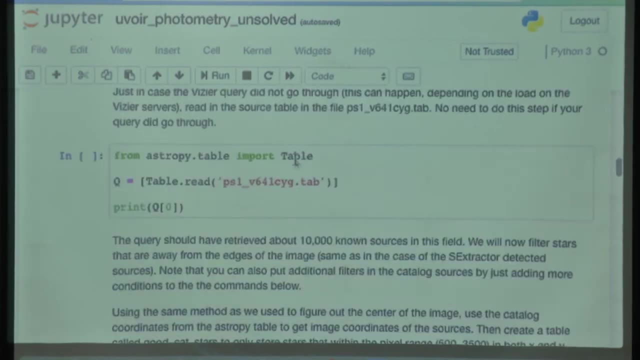 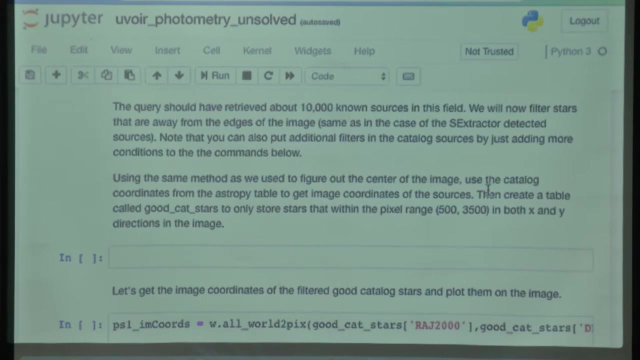 this is an exercise for you. So what you what? what the query returned is an AstroPy table, and you can filter on the AstroPy table to select stars that are only within within pixel coordinates of about 500 to 3500, with that is about the center of the image. 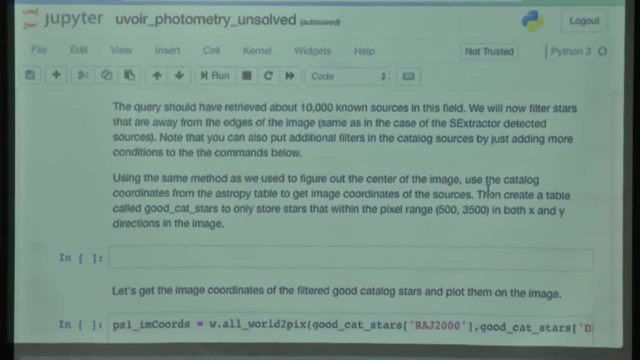 So you can give it a try. I'll wait for a moment, but I'll show you the solution eventually. So the idea is to you have the coordinates of the stars that were returned from the catalog, And then you want to only select stars that are within the center. 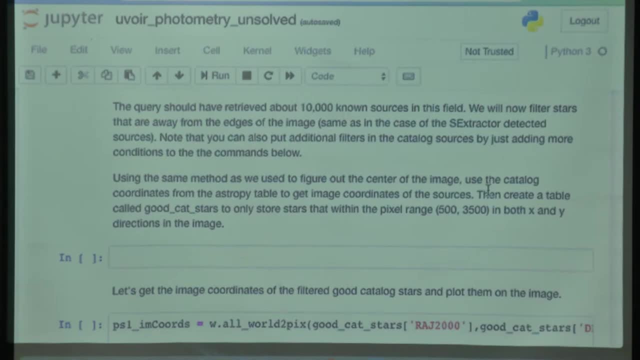 some central box of the image, Because we only want to do photometric calibration with those stars. So give it a shot. Yeah, we'll continue after a moment. So what you want to do here is get the pixel coordinates for all of the stars that were detected in that were returned by the catalog. 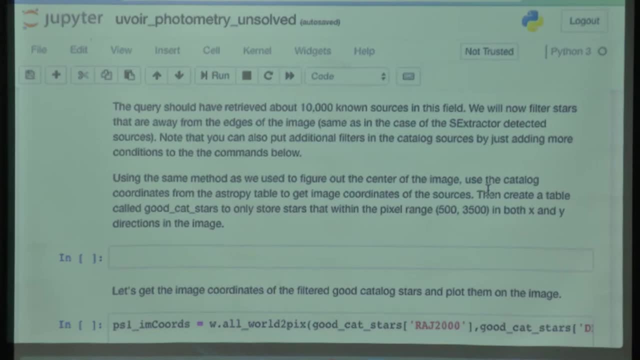 You have to get the pixel coordinates for those stars and then create a list of stars that are inside the central- whatever 3000 pixels of the image. Okay, anybody still having issues with getting the external catalog working? Did everybody get the external catalog print out? 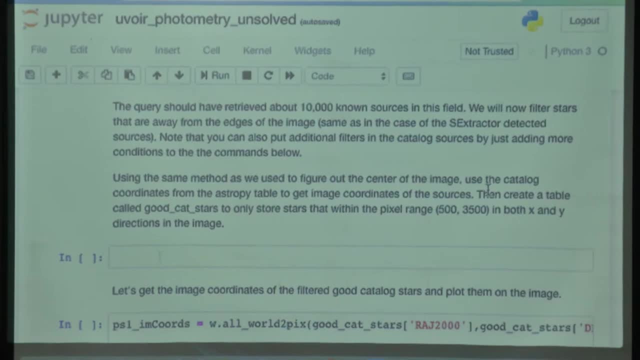 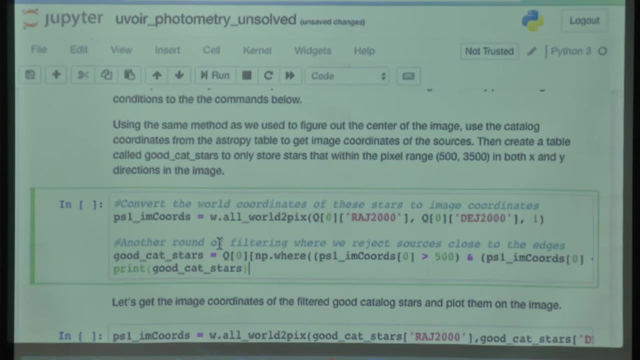 Anybody with still an issue getting the external catalog. Okay, so let's see what we are doing here. So, if you just pay attention to this, So what we're doing here is that. so q is an AstroPy table with the coordinates of the objects, the array and deck for the objects that are within the 30 RQ. 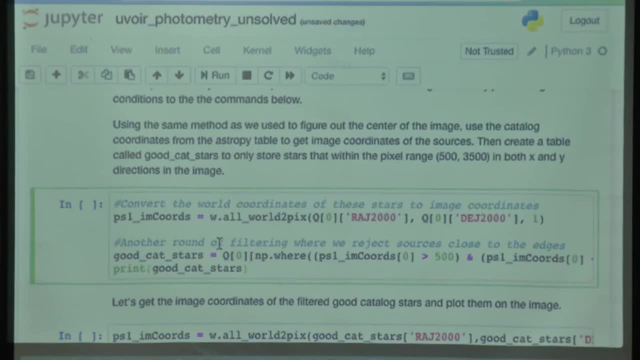 minute radius and I'm using this function, AstroPy function, to. so it says world to pics. world to pics means give, trans, convert the array and deck coordinates of the stars in the image to pixel coordinates based on the WCS of the image that I already know. so W is the WCS of the image that we already. 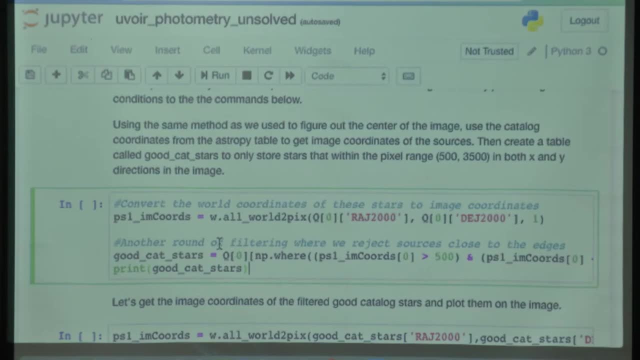 know, I'm asking AstroPy to give me the pixel coordinates for these stars and then, once we have the pixel coordinates, what I'm doing is I'm creating a, an array called good catalog stars or good cat stars, where I'm requiring that the the X coordinate is: is the X coordinate of the star is greater than 500 X. 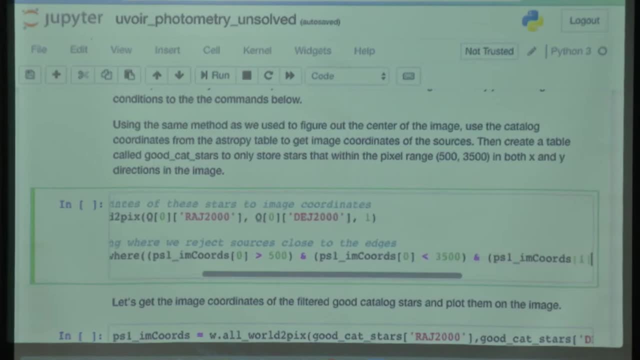 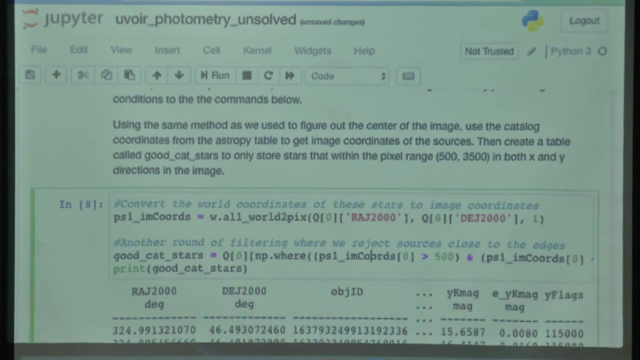 coordinate is also less than 3500, the Y coordinate is also greater than 500 and the Y coordinate is also less than 3500. so I am only selecting stars that have pixel coordinates within some central region of the image. any questions about that? oh, yes, okay, yes. 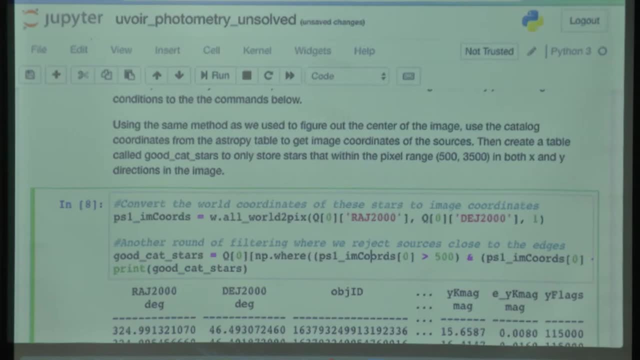 yes, the world to pics function. yes. so the what world to pics does is that if you give it a list of RA and dec coordinates for the stars in the that you expect to see in the image and you say world to pics, what it does is that it converts those world coordinates to pixel coordinates in 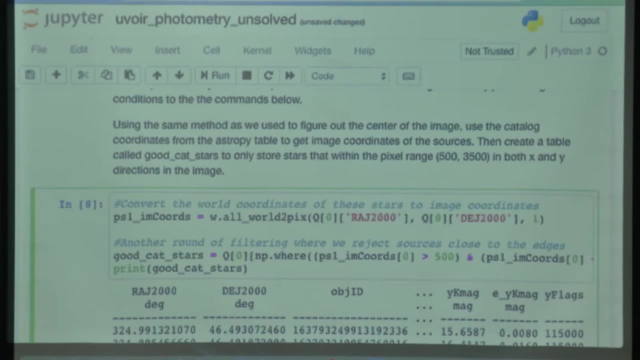 the image and the way it does. that is because I know the position of the image in the sky. so if you give me any given RA and dec, I should be able to tell you what is the pixel coordinate of the image. yes, crop the. okay, you might have an interesting. 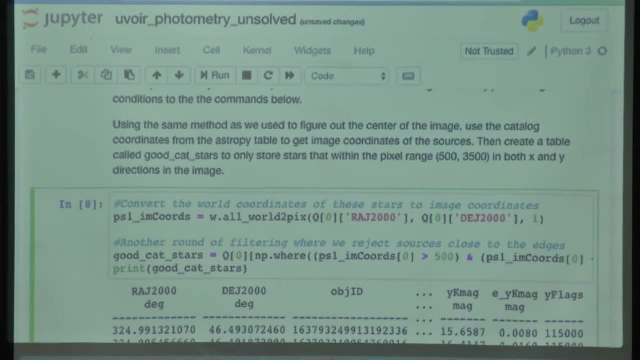 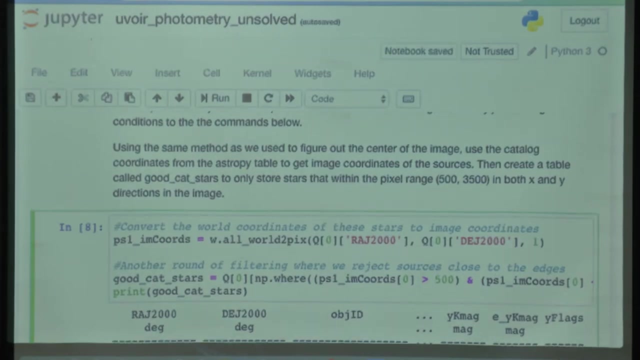 you might have an interesting source at the edge of the field, so might have. so I mean, I mean it's there's no reason to crop the image really. yes, yes, yes, okay, I mean cropping the image would all always mean losing information. I don't think I mean it's just for the photometric calibration that I'm 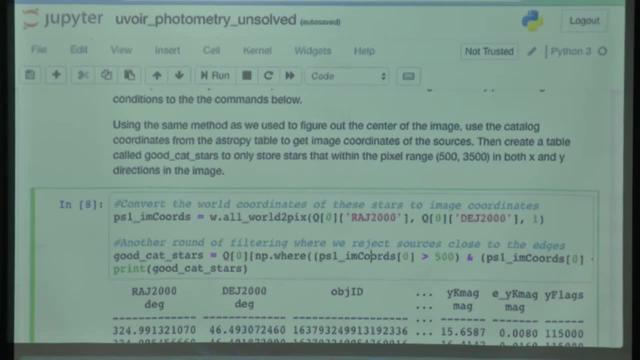 selecting stars within the central region of the image, just for the photometric calibration. yes, okay, so just in case you want to look at this again. so, once you set this up, just create this variable: good, underscore, cat, underscore, stars, where you require the code, the X coordinate. so 0 is X. 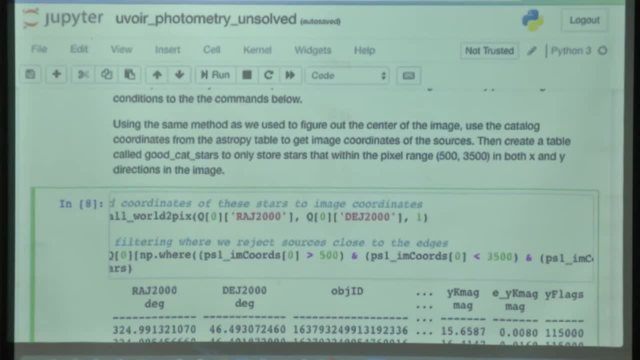 coordinate. the X coordinate should be between 500 and thirty five hundred and the Y coordinate, which is in the in the first axis, you should be again between 500 and thirty five hundred, and just try to print it out. see if you can print it out. okay, if you. if you're still having issues running this step, 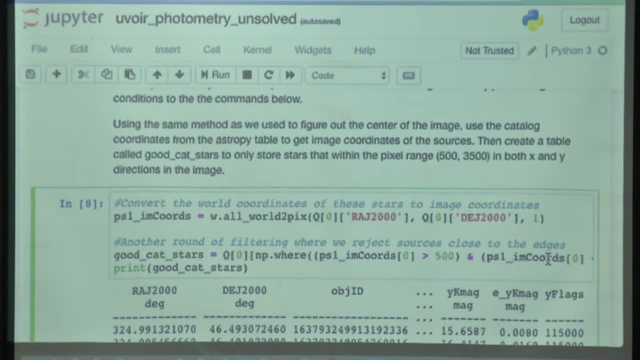 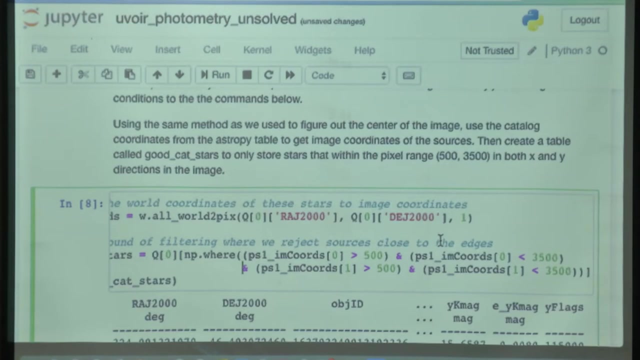 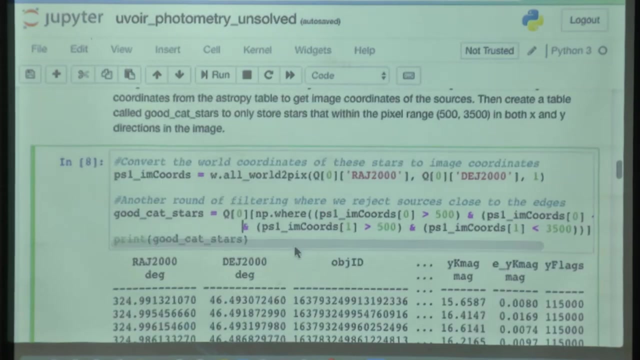 raise your hand. oh okay, I mean, it's just a continuation of this, so what you're doing here is sorry, what? oh, okay, yeah, yes, I hope this is visible. oops, yes, I think I can move on. yes, okay, so I am going to move on to the next slide. 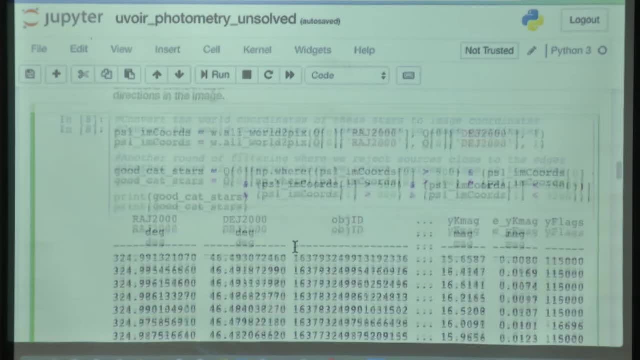 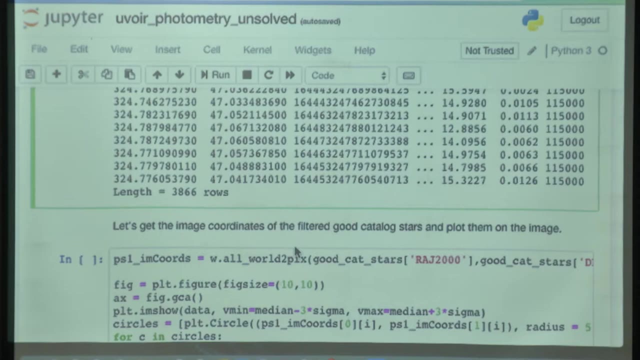 thank you for your patience. good night. next step: So by now you should have the list of x and y coordinates for Panster sources that were detected- sorry, that are inside the field and what. just to make sure that you didn't get anything crazy, you can overlay the locations of those sources inside the image. So that's what. 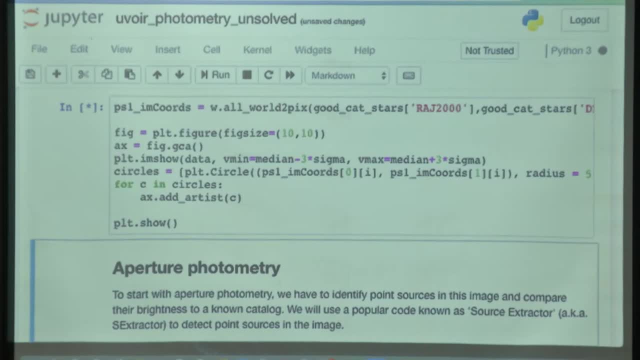 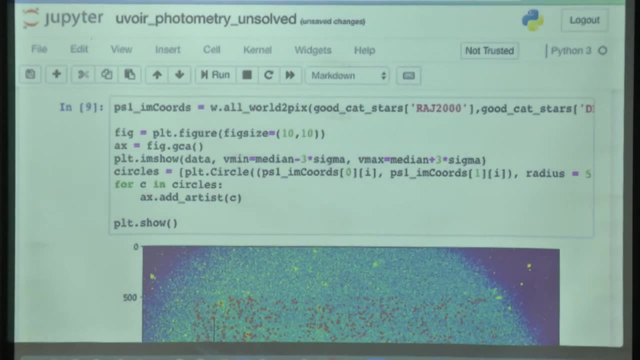 the next step does So. what I'm doing here is I am getting the x and y positions of the source Panster, sources inside the field- and I am overlaying red circles on top of those positions just to see that what we are getting is these are actual sources inside the field that are detected. 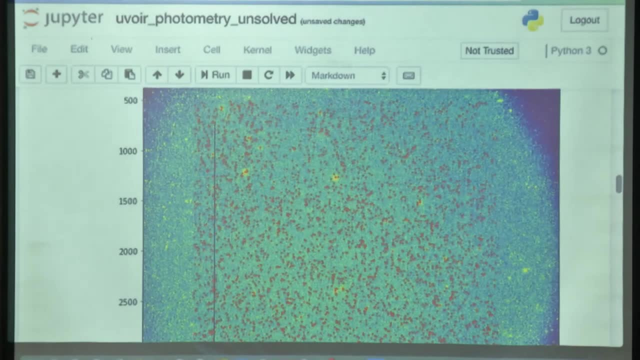 in the image, So you can play around with this. but you see, this is the growth India image and you see there are red dots on the at the locations of the images- sorry, of the stars- and you can play around with this. you can zoom into the center. 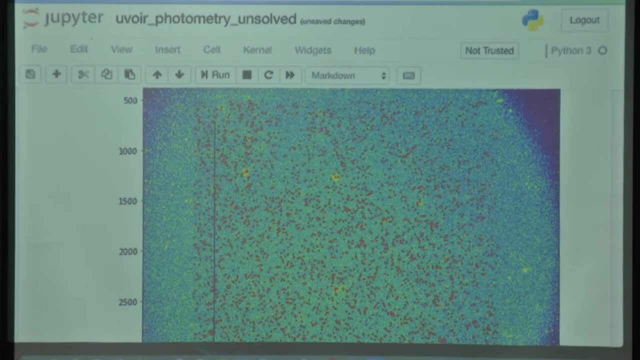 of the image to make sure that what you are actually seeing is those are actually stars. I know it's a bit difficult on this scale, but you should in general see this pattern, which is red circles on the top of those Panster, on top of the detected sources. So what Varun just pointed out? 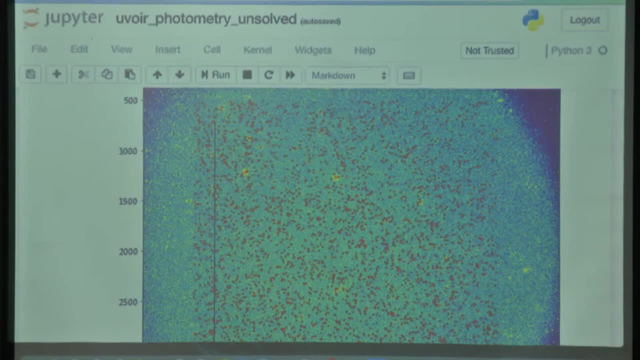 is that that Python has a slightly different convention for the axis when you open load of its image and try to plot it, In the sense that you will see different results if you open up an image in ds9 as well as if you open up an image in ds9 as well as if you open up an image in ds9 as. 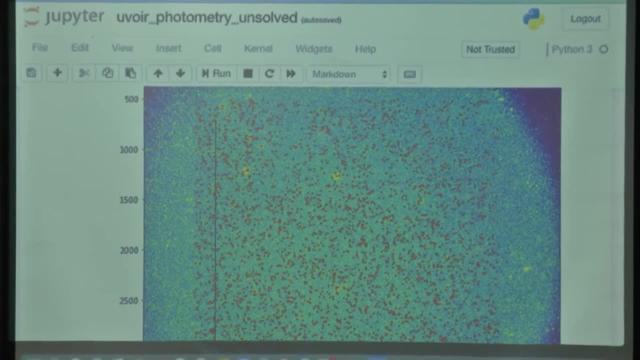 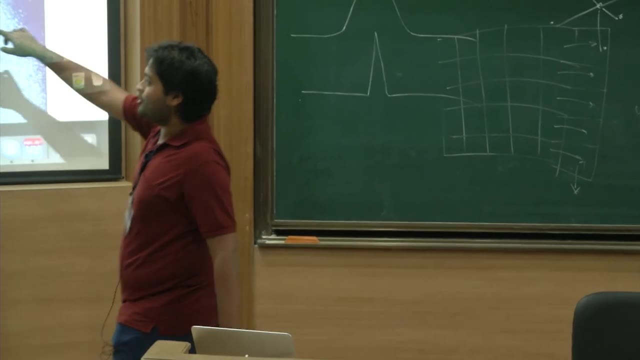 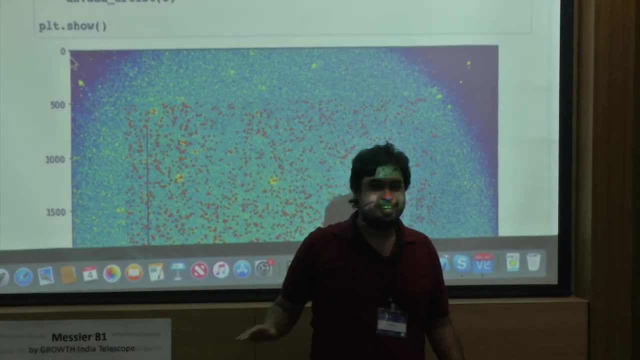 opposed to pointing, sorry, plotting it in Python, where it's because of the choice of the origin. So the in Python, the origin is always this point here. So, and if you plot it in xy coordinates, this is increasing x, increasing y, the ds, ds9 is of opposite. Yes, you can always be, but yes, yes. 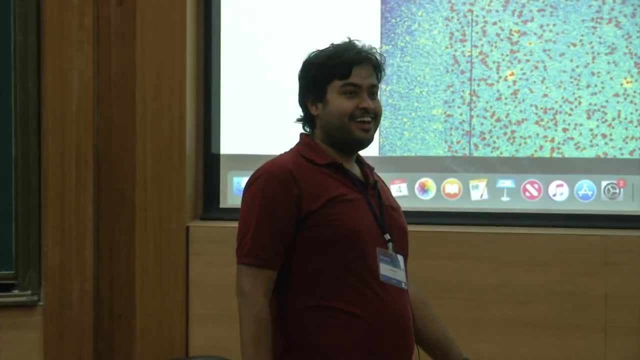 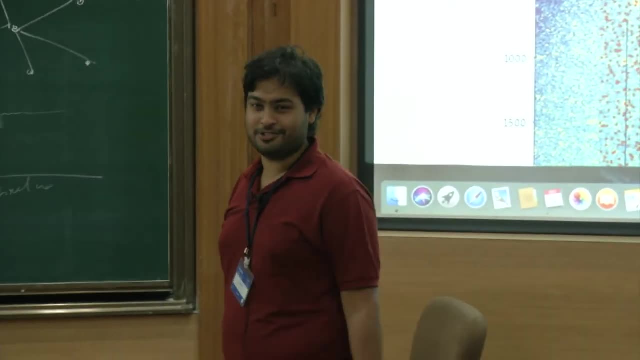 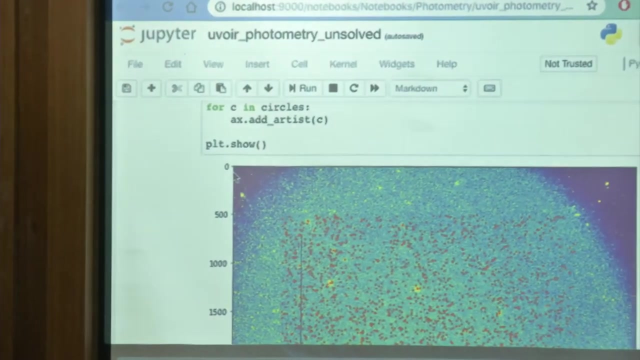 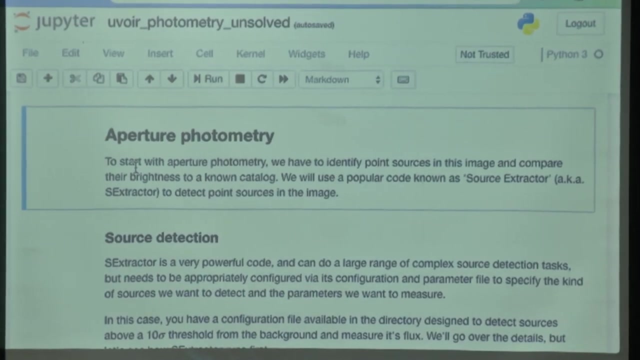 Yeah, yes, I mean just something you should know. I mean it's, it is a common confusion. Okay, how many people were able to display this? Raise your hand, Okay, that's okay, That's good, Okay, Yes, okay. So now is now we actually start the serious business, which is 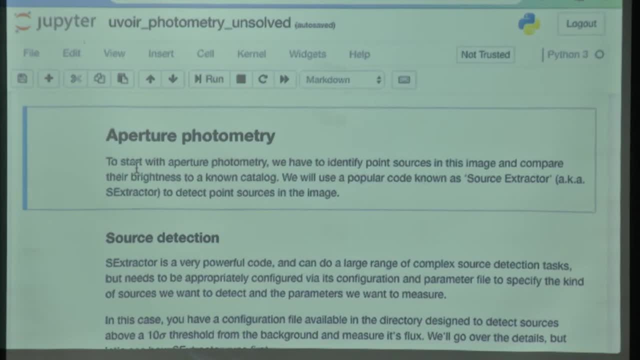 actually doing aperture photometry and so far we have a catalog of sources that we expect to see inside the field. The next step is to actually detect the sources that are seen in the image, and to do this we'll be using this very powerful code known as source. 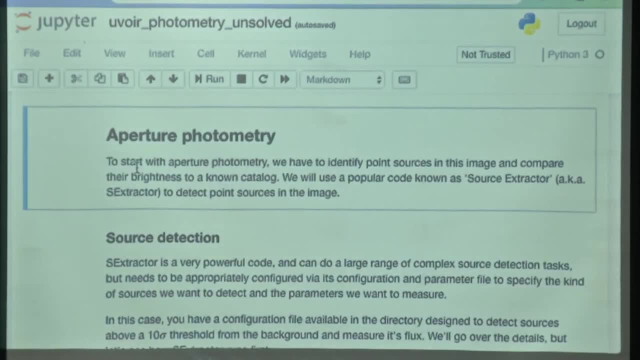 extractor where. so actually we did use source extractor even last time when we were doing the astrometric calibration, but I didn't go into the details there. but the idea is that source extractor is actually a very powerful software that allows you to detect sources inside the field, measure their measure, the amount of flux that you have inside those. 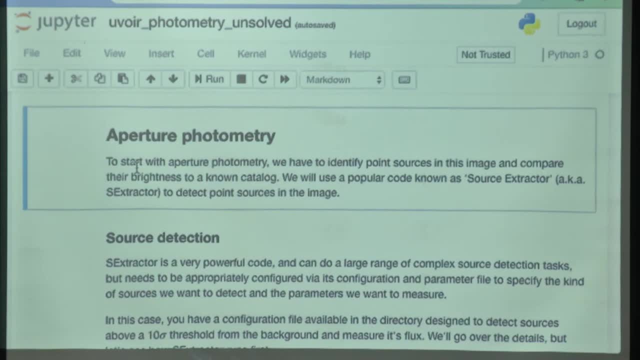 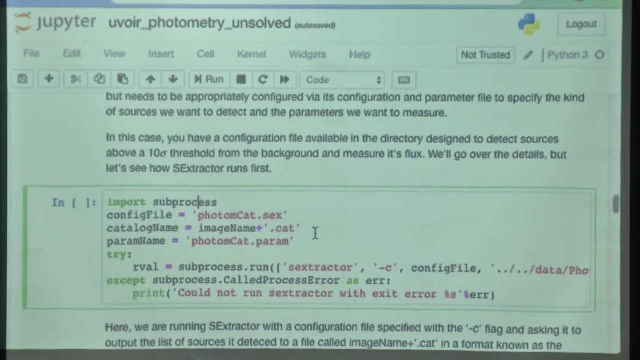 sources to actually do things like photometric calibration. Okay, So what you want to do next is to run source extractor on this image. So what I'm doing here is just a configuration file. So the configuration file is important for source. 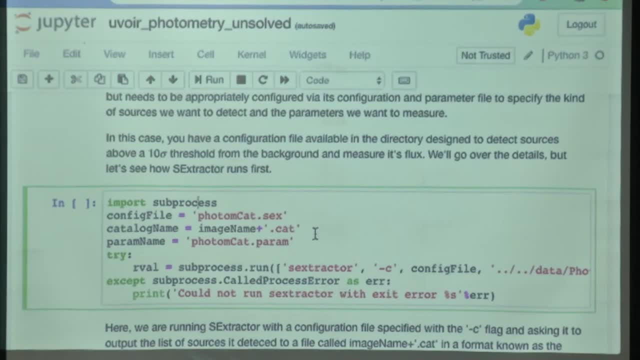 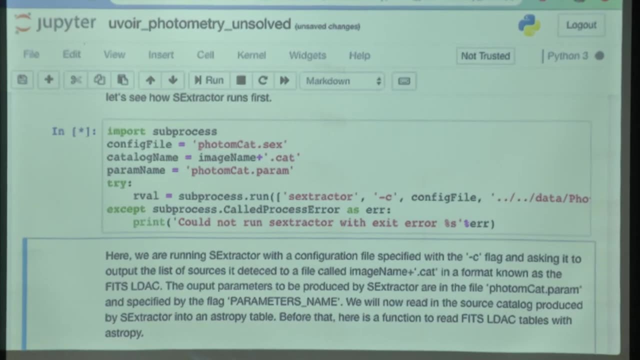 extractor. It actually controls the way source extractor runs. but in this case I've actually already given you what source extractor should do. So what you should do is just go ahead and run this and you can check the terminal. So you see, this is source extractor running. So it detected. 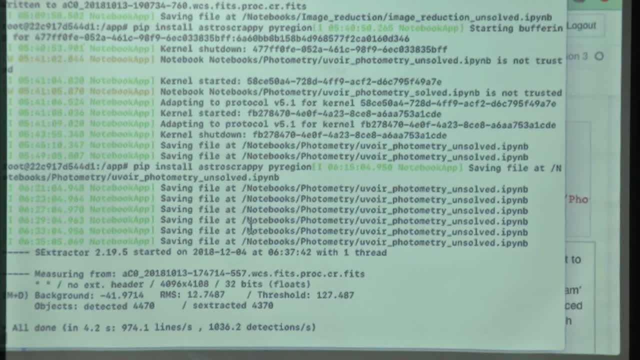 about 4,000 sources in the field. Okay, And while detecting the sources is actually already performed, all of the photometer that we need on those sources, Um, and that's what we'll read eventually to do the photometry on the sources that we want, Okay. 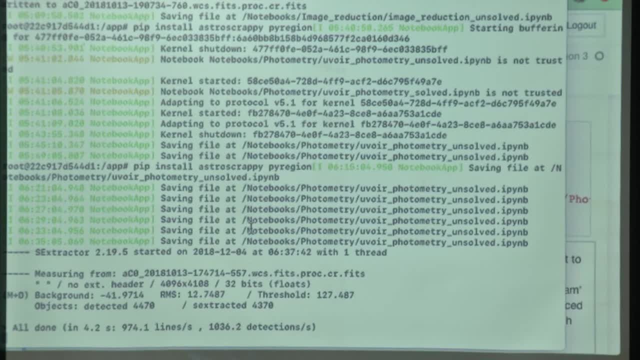 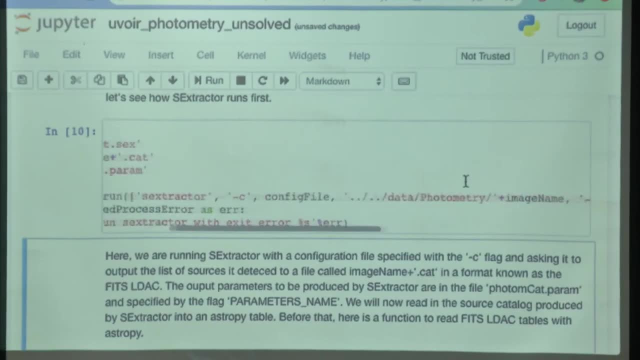 Did this step run? Sorry, What A path per second? Yes, it, oh good. Okay, so this requirements. Okay, We can run this For a particular object: 보�د. Okay, Okay, Um, Yes, uh, The configuration file should be in the same folder as was there in the docker. 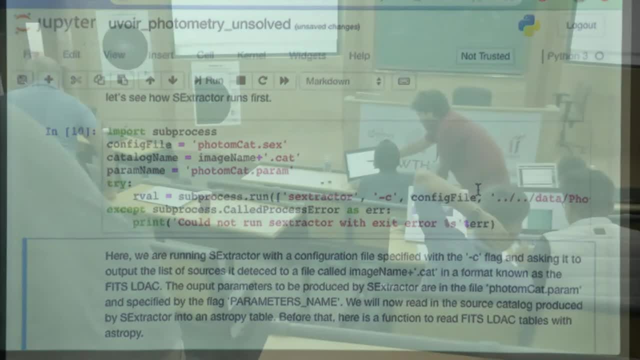 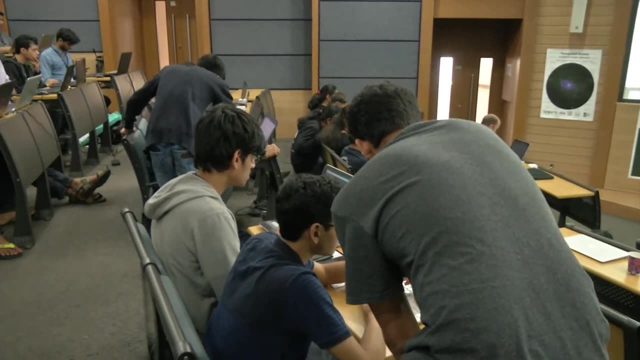 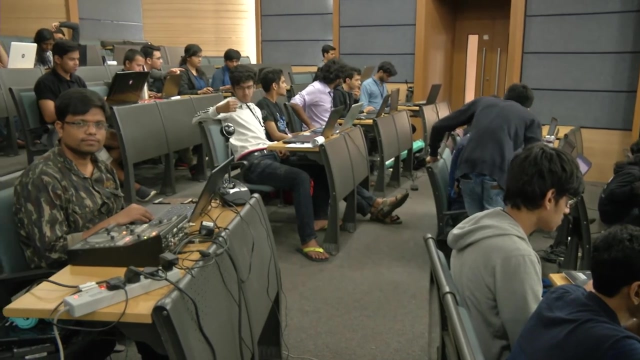 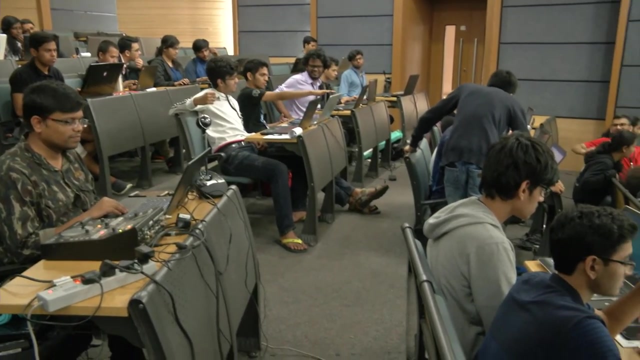 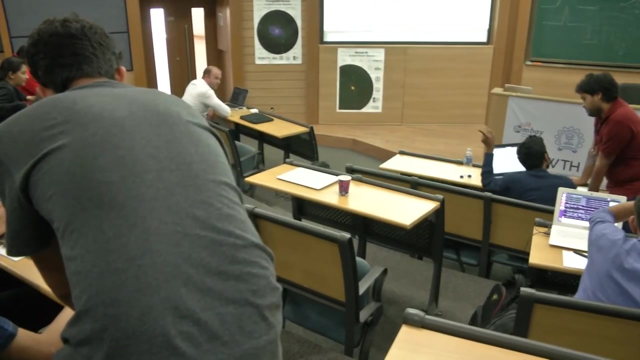 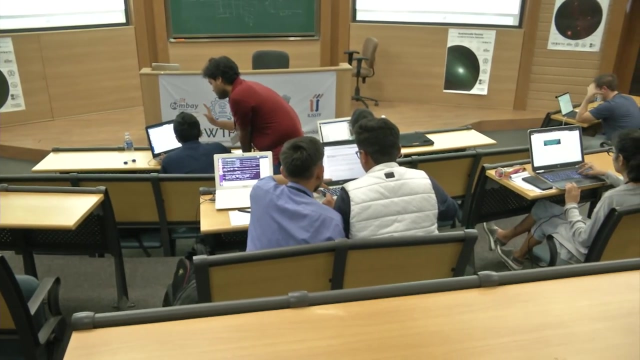 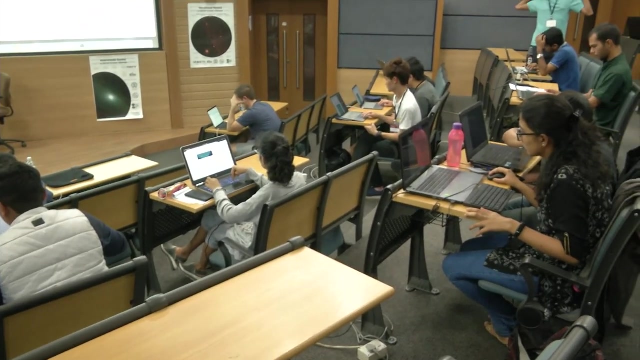 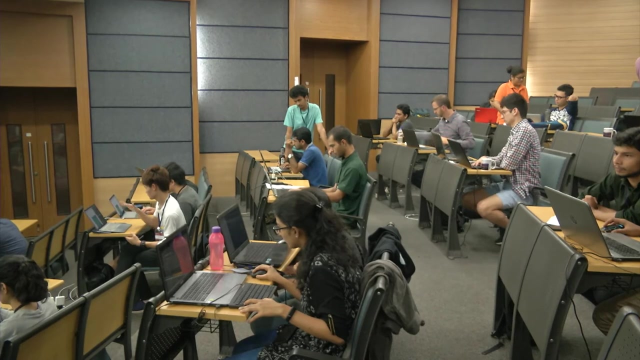 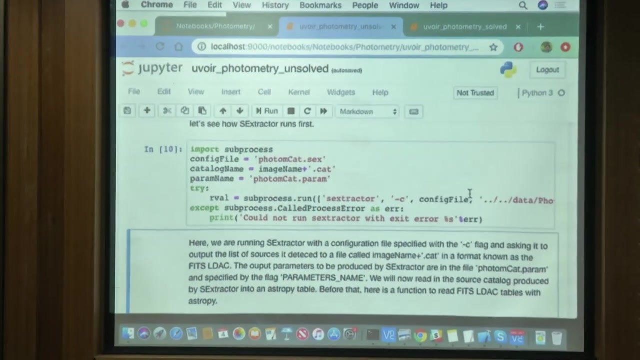 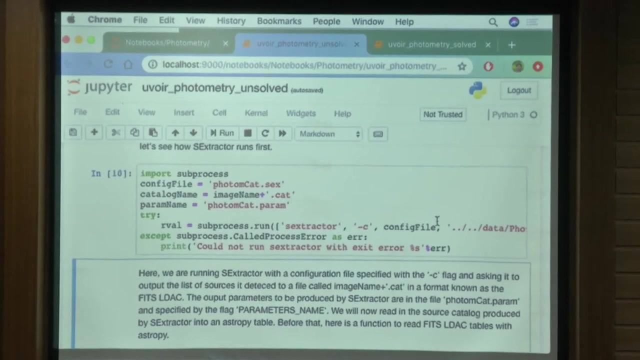 How many people are having issues running this step? The next step is to create a new folder. The folder should be in the same folder as was there in the docker. If you have any questions, please contact us at the chat box. Okay, it is running. yes, ah, LDSE is. I actually do not know the full form of LDSE, it is just. 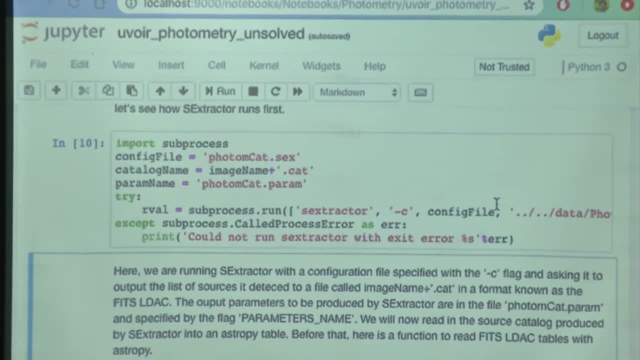 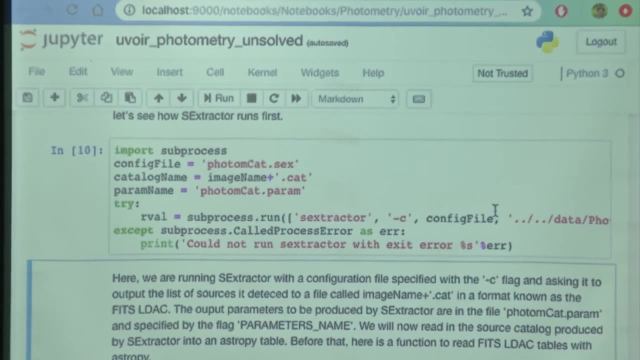 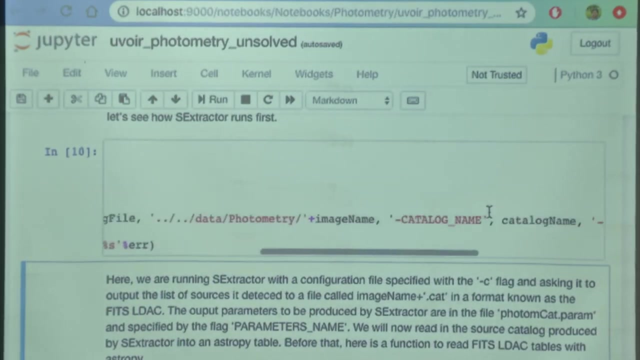 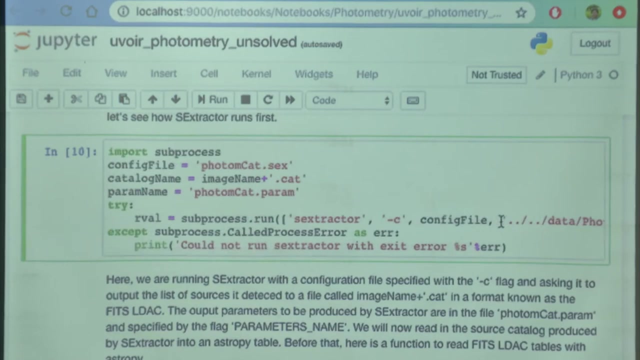 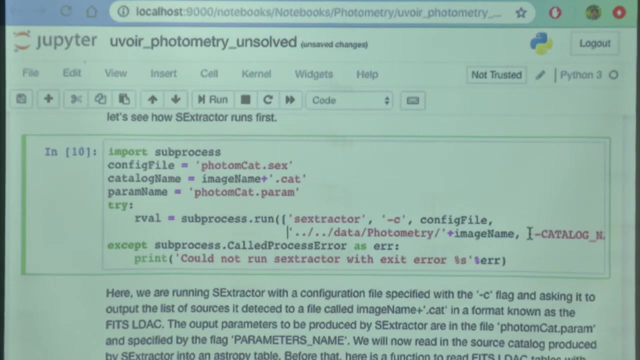 it is a format that source extractor uses to store the catalog of sources, that that it is actually a format that most astromatics software use. It is effectively a table that we will actually read the table eventually when we when we run it. 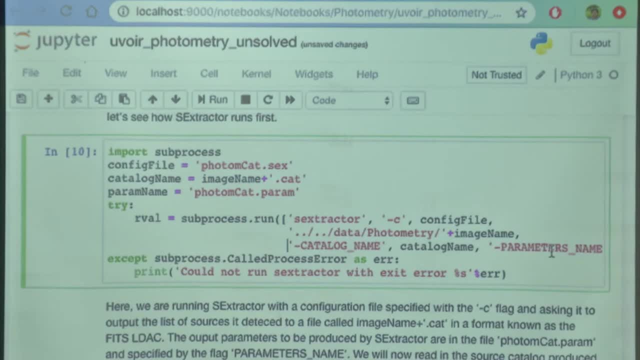 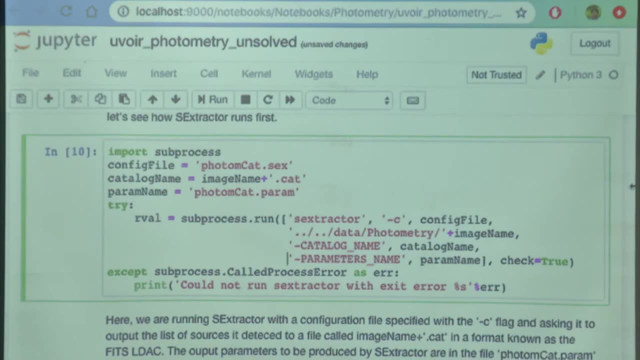 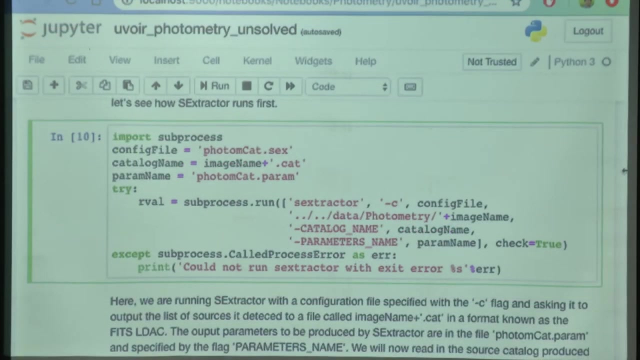 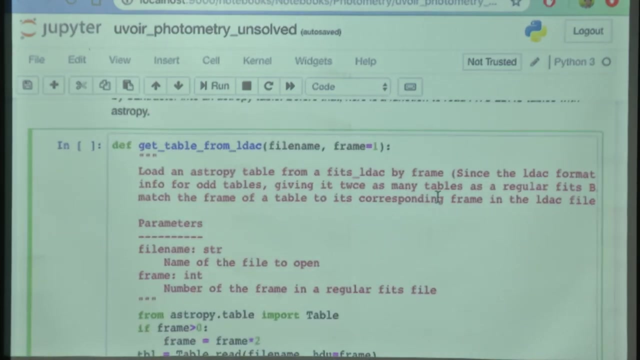 Okay, so I, okay. how many were able to run source extractor? Raise your hands, Yes, Okay. ah, I think we should move on because yeah, okay, okay, okay. So the next cell is actually just a function. it is, it is actually, it is just a function. 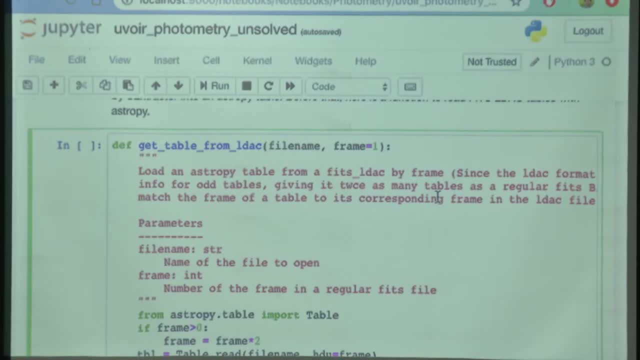 to read a fit. so the output from source extractor is in the format known as it is. it is a fits format and what I have done here is just made- made a wrapper- to read the fits format and read it into an astropy table. 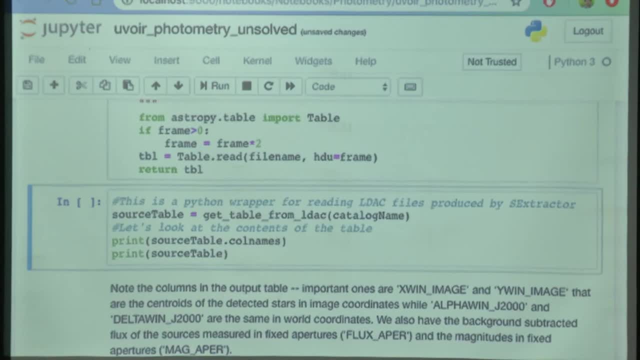 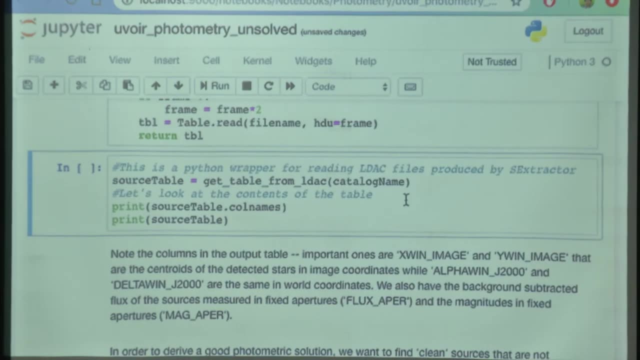 So if you just just just run that cell, there is nothing else. just run that cell, it will define this function and after that you want to. what I am doing here is I am reading the output from source extractor, using this function and printing out the output. 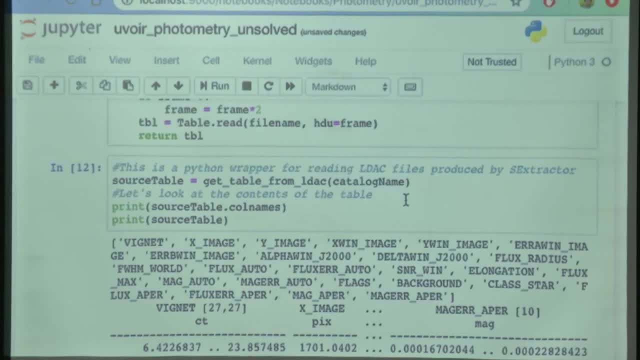 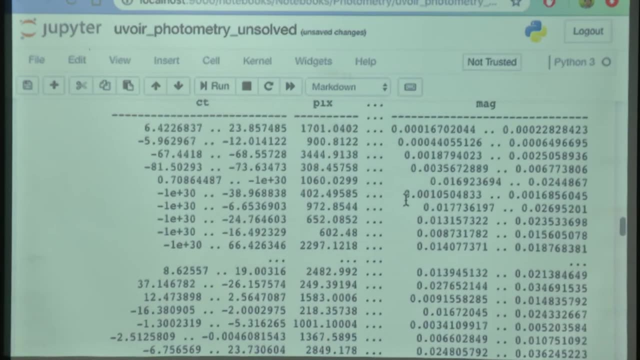 So, if you were able to run this step, what you should see is all of the parameters that were measured by source extractor when it ran and, as well as you know, just a a list of parameters for the really random sources in the field. just make sure you see something. 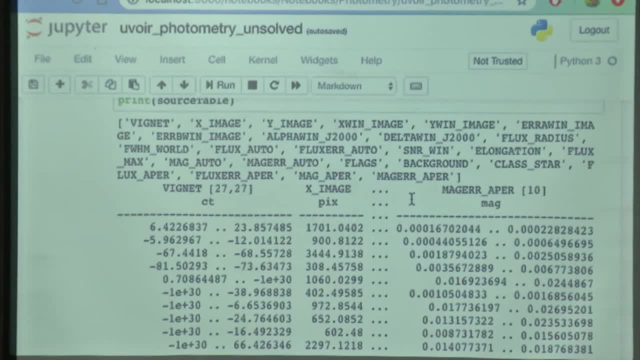 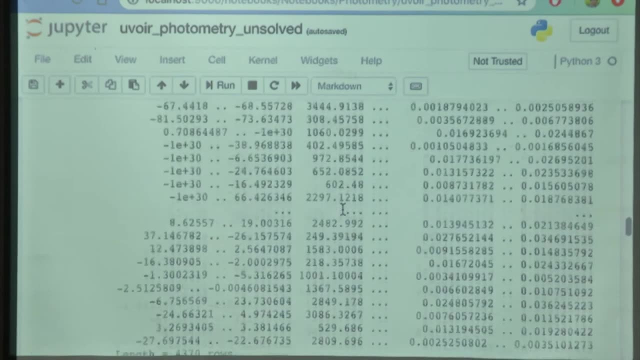 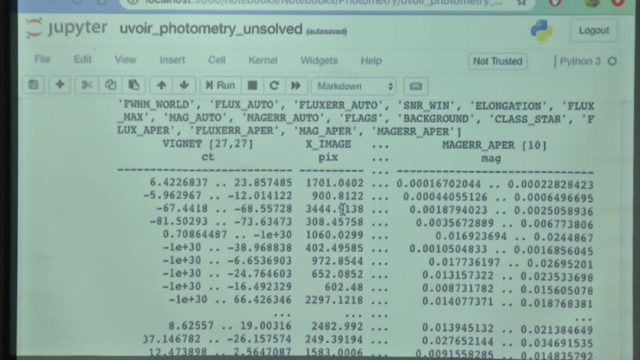 like this: Okay, so how many were able to get print this table? Okay, so what do I have next? So, just just so you know, just note, you know the kind of columns you have. you have the x position of the x position of the source. there is a column that has- sorry, the column. 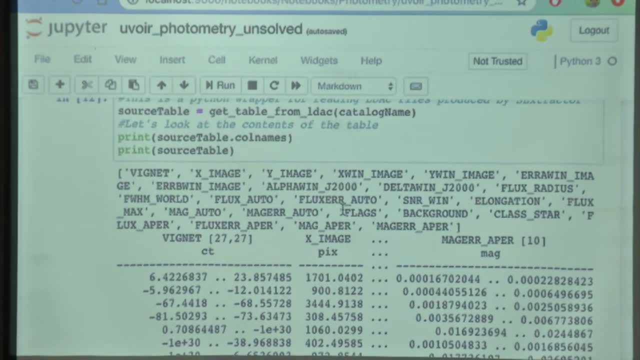 names are displayed. so there is a, there is a x and y position of the source. there is the flux in the source. there is there are actually even aperture based magnitudes in the in the in this table. So if you look at these columns- mag underscore upper, mag error underscore upper- these are all aperture magnitudes that were already measured while source extractor ran. 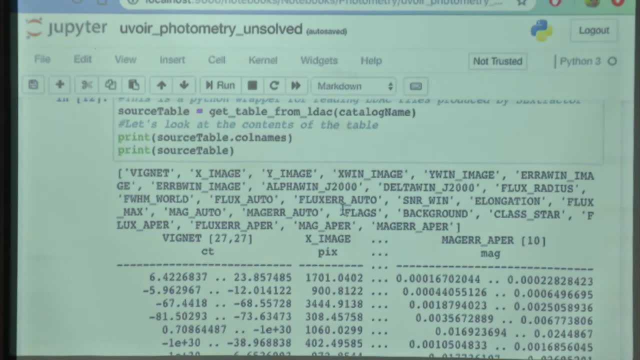 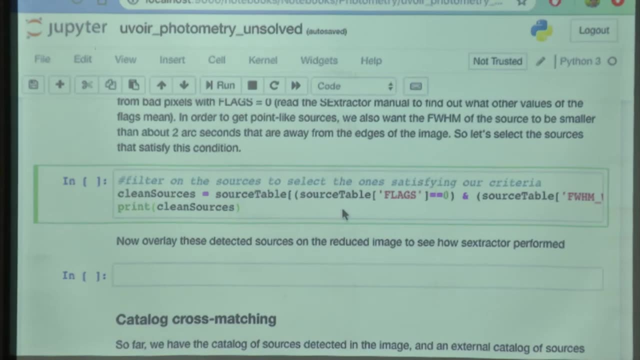 So we, in principle, we actually already have the data that we need to do the photometric calibration. So, if you go further down, so what I am doing here again is selecting a set of clean sources to do the photometric calibration on. 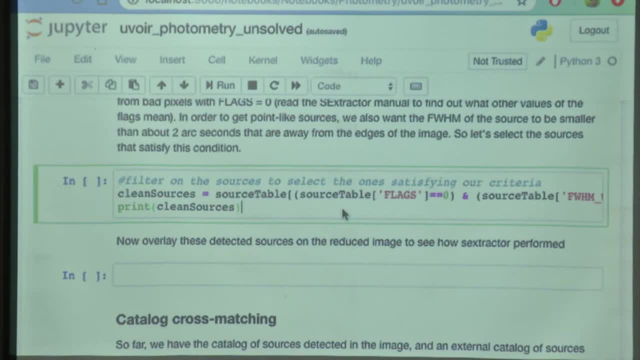 And one of the columns that source extractor does produce is this column called flags, where flags for good sources should be zero If, for example, either the source is saturated or it falls on a bad column or something. So, in particular, we can just make sure that the source is saturated so that we have at least one or two photos and we can then find, you know, the new conditions for those conditions. 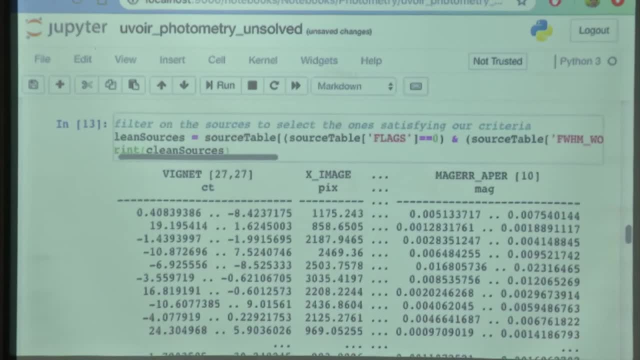 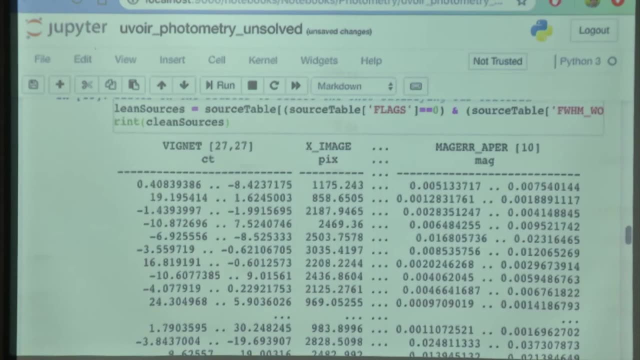 And what I do is I can type this in the input code that I want. so I can type: this is image, and then I type angle, and then I type this in the output code that I want, And then I type what I'm looking for and that's what it is. 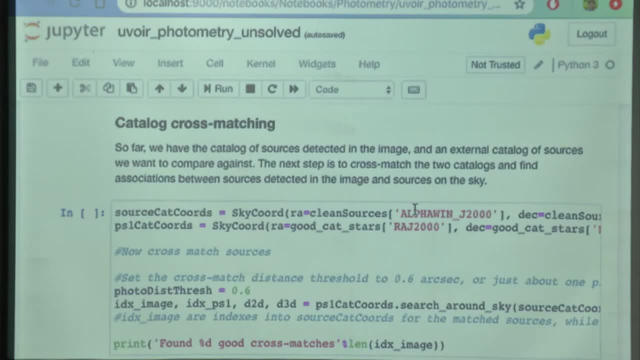 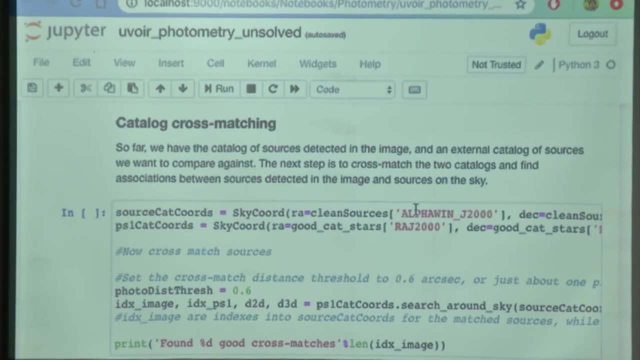 so you now need to figure out a cross match between every given source in the detected image to every source in the PANSAS image, in the PANSAS catalog, and that's what we'll do in this step of catalog cross matching. what we are effectively doing is that 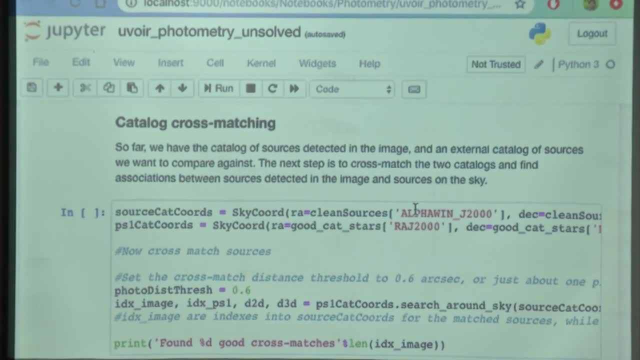 we are taking two catalogs- one is the PANSAS catalog, one is the source catalog- and asking AstroPy to cross match them. cross match all stars that are, in this case, within about 0.6 arc seconds and 0.6 because that's about the pixel size. 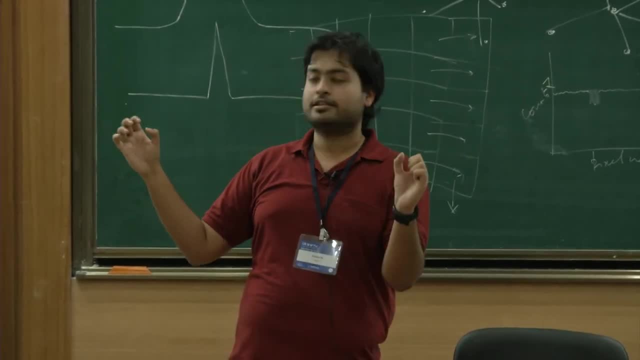 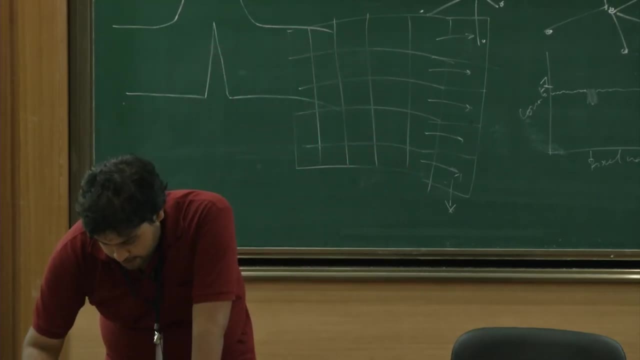 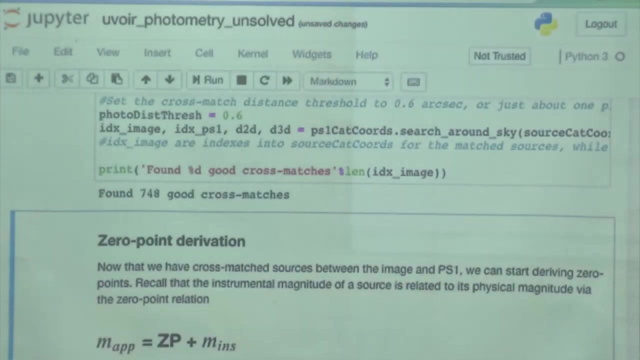 of growth, India. we are cross matching all sources that are within about 0.6 arc seconds of each other, so if you go ahead and run that, it should tell you that it found. so how many cross matches. in this case, it found about 750 sources that were cross matched to each other. 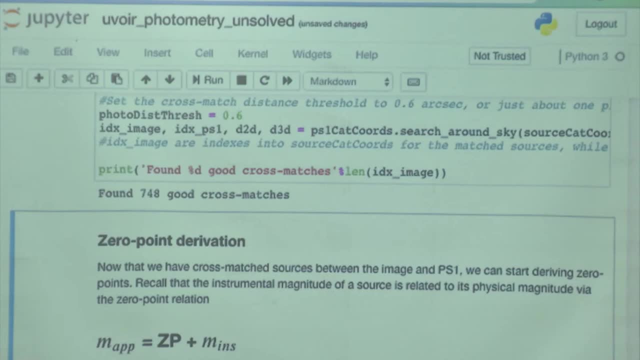 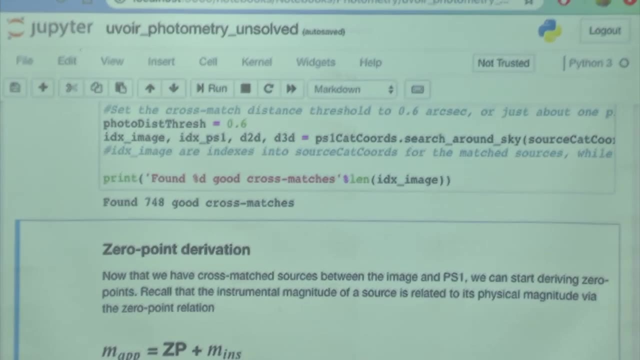 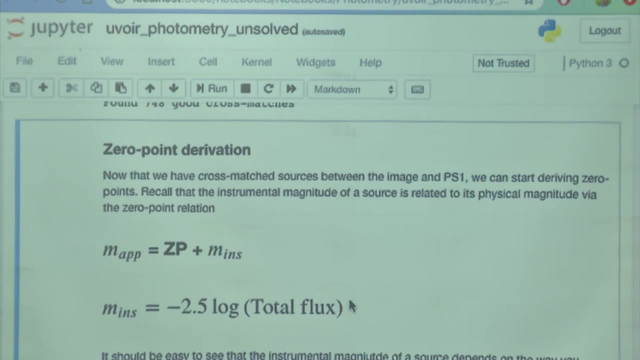 inside the field. no, I mean, it typically should be smaller than a pixel, yes, but I just chose one pixel in this case. so now the actual part of photometry which is deriving a zero point from the image. so, as you heard in the lecture already, the apparent magnitude of a source as 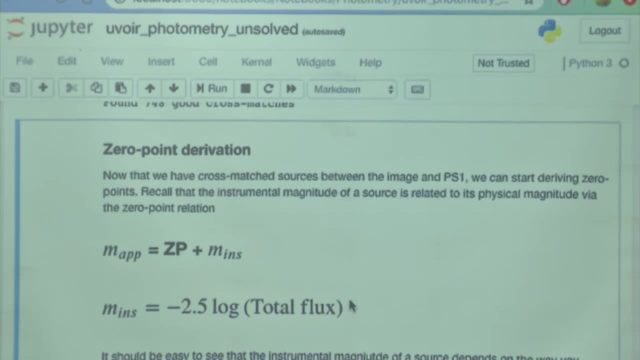 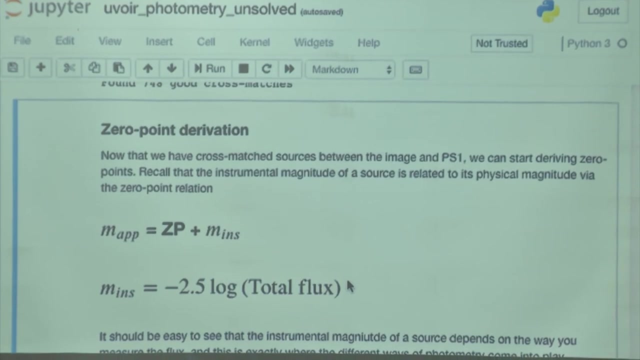 measured should is related to the instrumental magnitude of the source by the zero point, and the instrumental magnitude is just minus two and a half log of the total flux. and because you're measuring a total flux, the flux depends on the size of the aperture that you use. 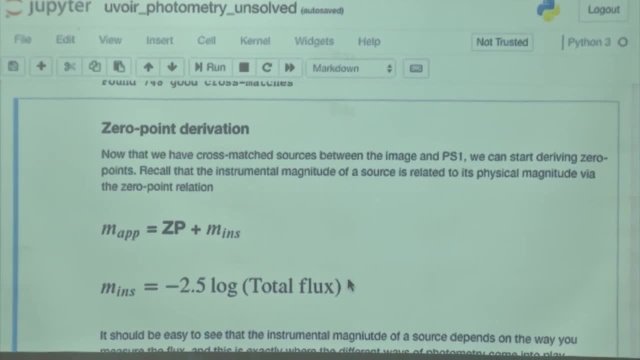 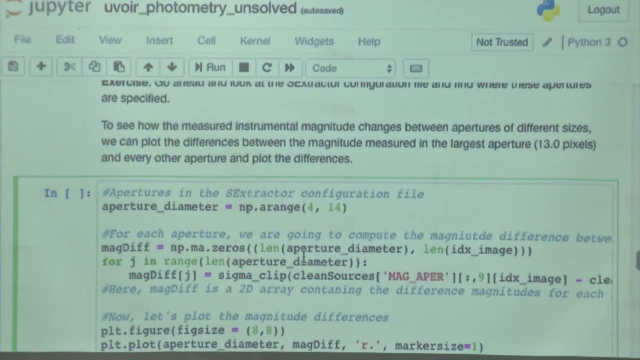 which is exactly where this idea of aperture correction comes in. well, so the idea is that, in order to get consistent magnitude measurements, you should measure the magnitude of your calibration star in the same aperture as that of your science target. and in this case, let's see, yes, and because the larger the size of 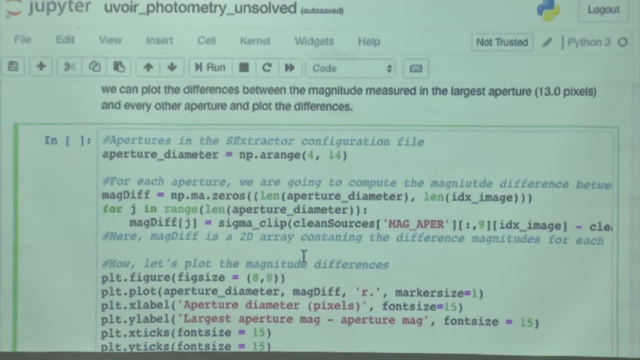 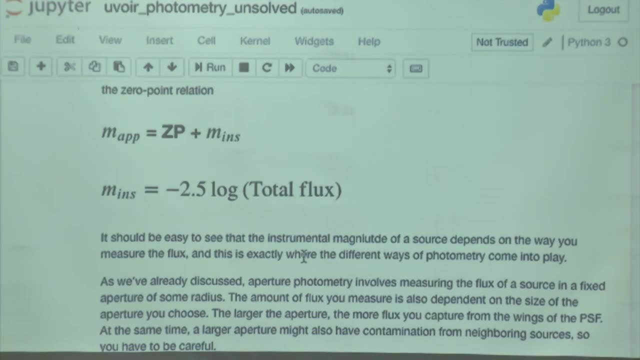 of the aperture, the more flux you're collecting, the magnitudes will become systematically smaller for larger and larger apertures because of this minus sign. So the larger the aperture, the larger the total amount of flux, the smaller is the magnitude. So if you look at your 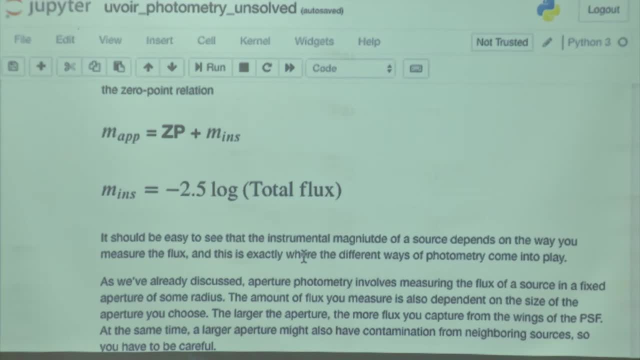 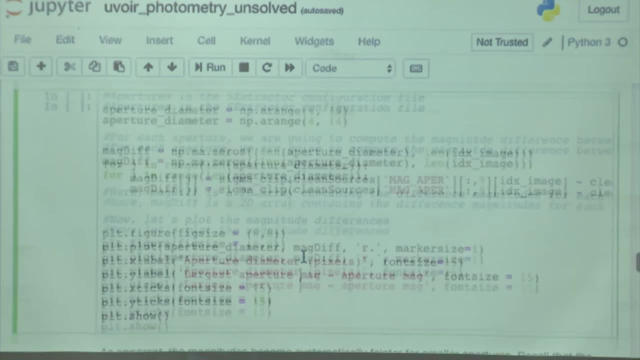 magnitudes as a function of the size of the aperture. you should see a constant trend, which is: you'll get brighter and brighter sources, for well, those are not those brighter and brighter measurements for larger and larger apertures. So this is what I'm. 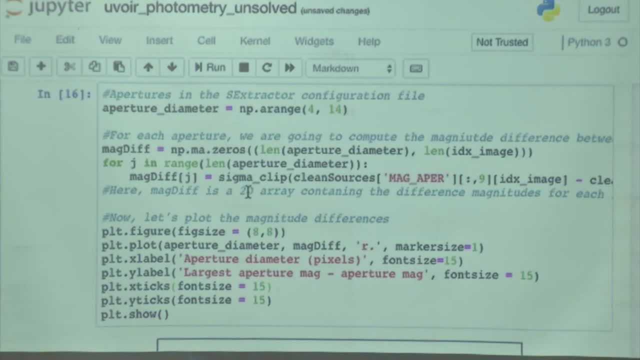 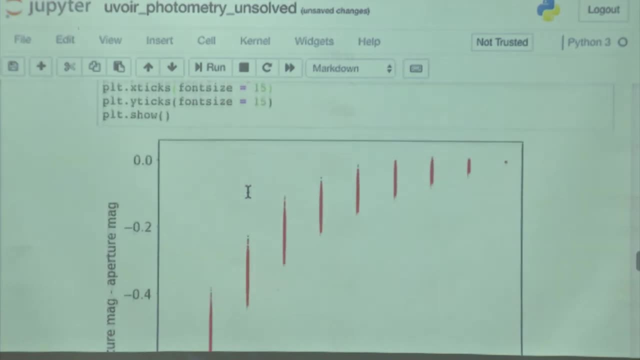 doing here, which is I'm plotting what is effectively what Sudhanshu mentioned as the curve of growth, where the idea is that the bigger the aperture, the more the flux, the smaller the magnitude. So if you're able to run this, you should see something. 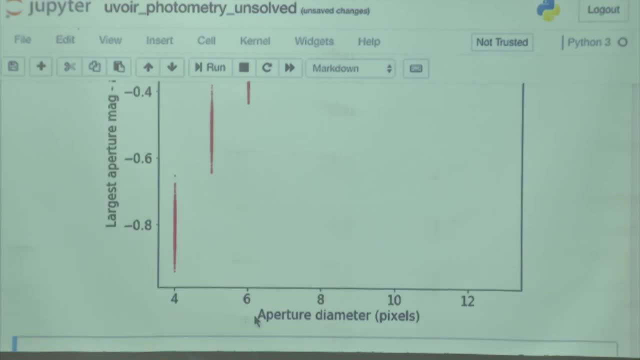 that looks like this. So on the x-axis is the diameter of the aperture and on the y-axis is the magnitude measured with respect to the largest aperture. So you see, it becomes brighter and brighter for larger apertures, and this is what 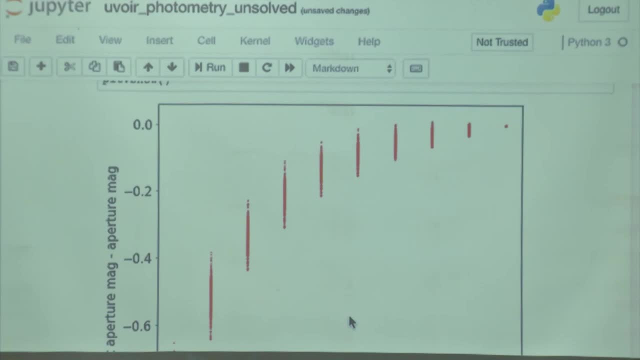 we saw earlier as the curve of growth, and this is from actual data. Yes, Okay, Which formula? Not yet, no, So these are instrumental magnitudes. Yes, these are the magnitudes in this case are still measured with respect to the raw counts in the image. 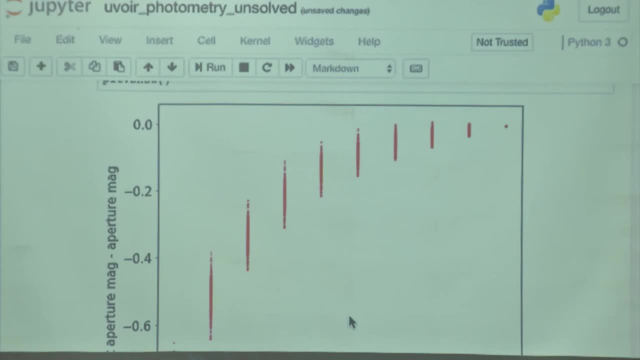 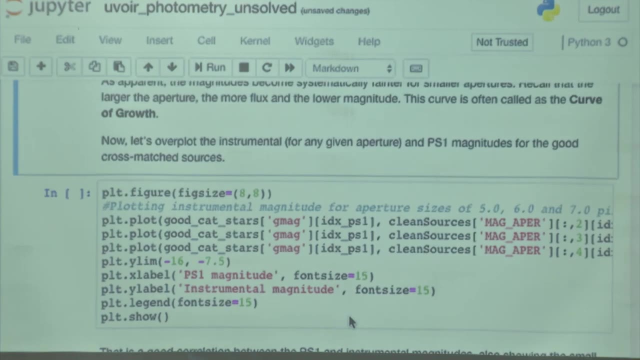 But we will do that as soon as we derive a zero point. So let's see, Okay, So now. so this step is really the deciding step, step to see if you actually got a good cross match, a good calibration, because 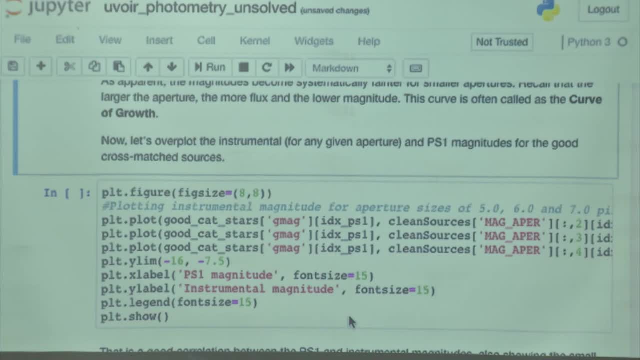 what we will do here is that we will plot the instrumental magnitude of this, of the sources detected in the image, against the known Pan-STARRS magnitudes, and if your instrument is fine, if growth India is fine, then we should see a good correlation between them. okay, so what do you guys have to say about that looks? 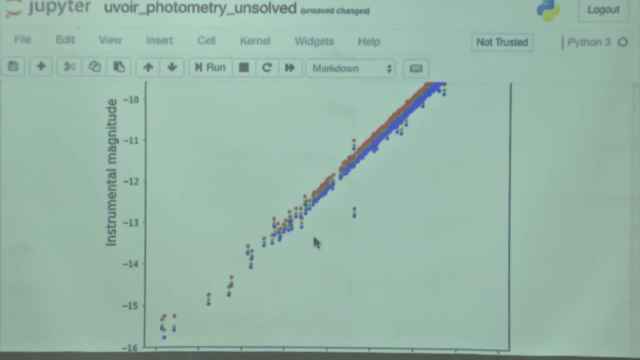 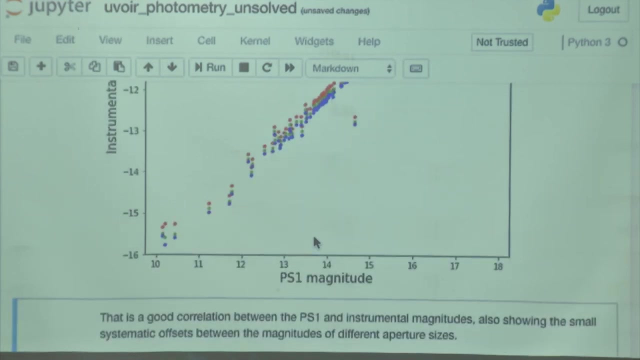 good. so about your question about variable stuff? so you see those outliers, those are variables. so again, this is a plot of. on the y-axis I have the instrumental magnitude, which is related only to the counts detected in the image, and on the x-axis I have the known magnitudes of the stars. so in principle, 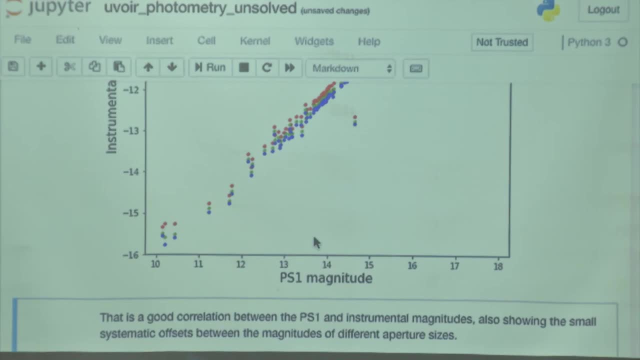 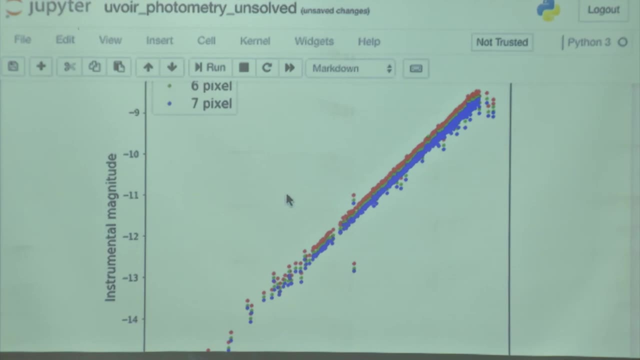 if your instrument is fine, the brighter that. the brighter that known magnitude, the brighter should be the instrument of magnitude. there should be a one-to-one relation and that's what we are seeing here. and these red, green and blue points, these are just magnitudes measured in different apertures, so that the magnitudes are slightly brighter if 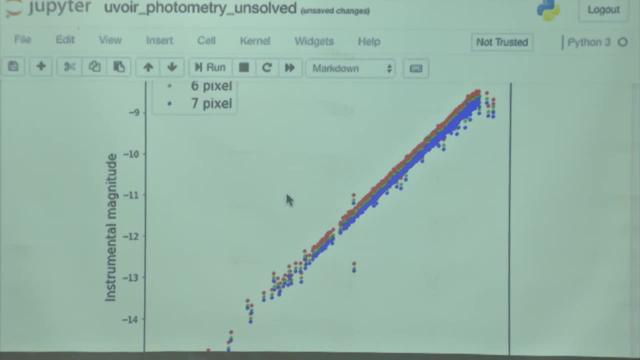 you use a bigger aperture. okay, right, so. so there is some. there are some funny things going on in the towards the ends of the ends of the two, the two ends of the plot where, typically, if you, if your source is really bright, then it is very likely that your CCD is going into the nonlinear regime. in those cases, 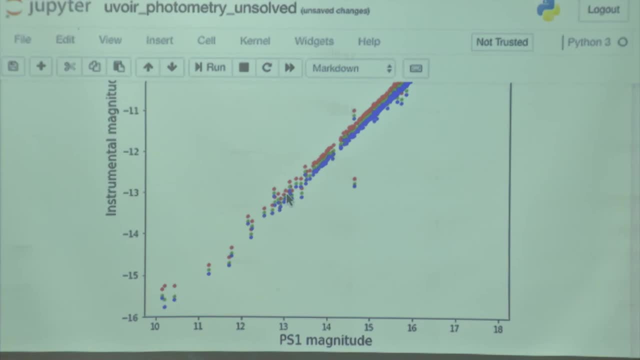 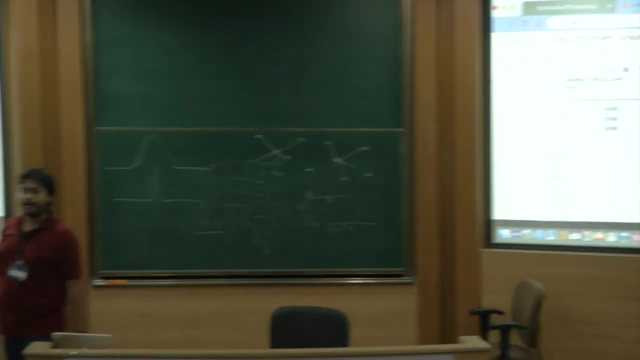 you will see that the magnitudes are not quite where you expect them to be, and you don't want to use those stars for photometric calibration on the faint end. I think it's just a matter of signal to noise, which is if your source is really. 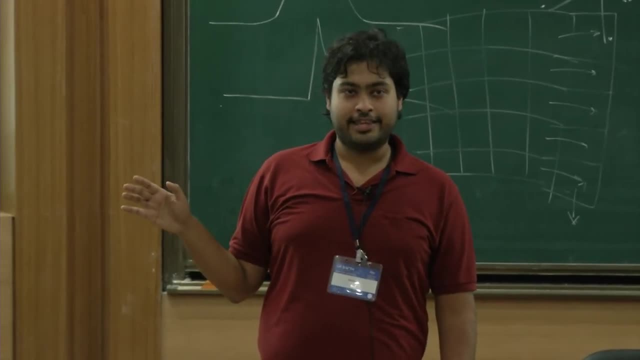 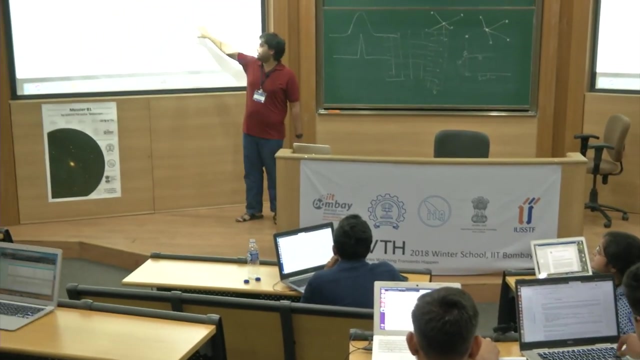 faint, then you do not get enough signal to noise on those targets and then your photometric measurements will not be as accurate. yeah, yeah, so that's the thing. so just note that what I've plotted here is the magnitudes in three different apertures. so this red. 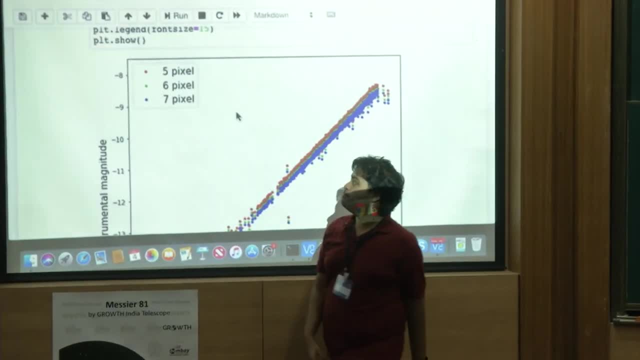 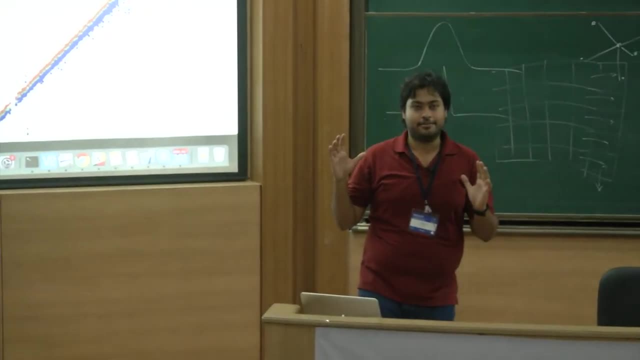 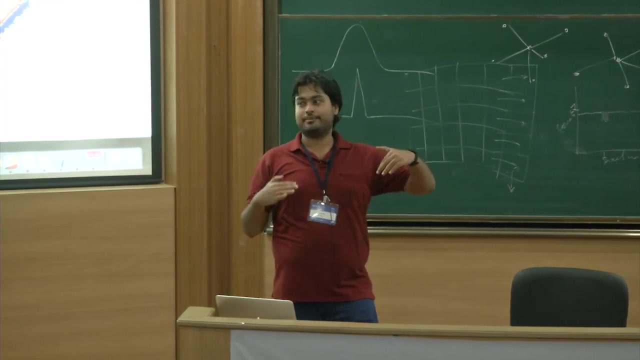 is 5 pixel, 6, green is 6 pixel, blue is 7 pixel, and there is a systematic offset between these two again because, as I said, the larger the aperture, the the more flux you are collecting, the smaller is the magnitude, which is why, even though there is a one-to-one correlation, the correlation is has a systematic. 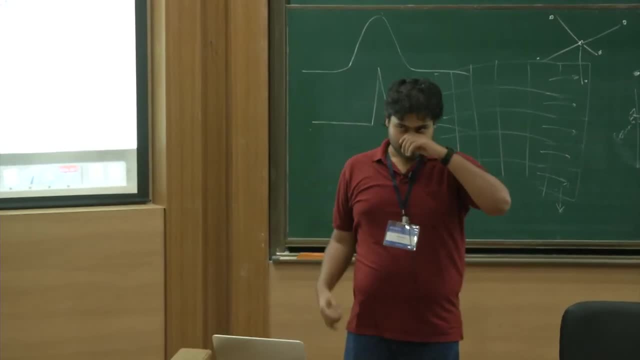 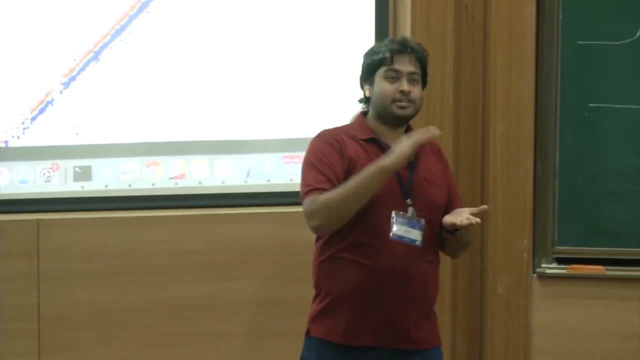 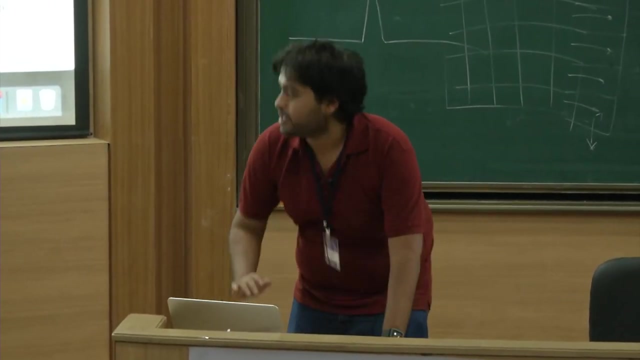 offset as a function of the pixel size. so the the entire exercise of deriving a zero point is just to measure what is the offset between the instrumental magnitude and the known catalogue magnitude. and that's what we'll do in the next step, where what I'm doing here is effectively for each aperture diameter. 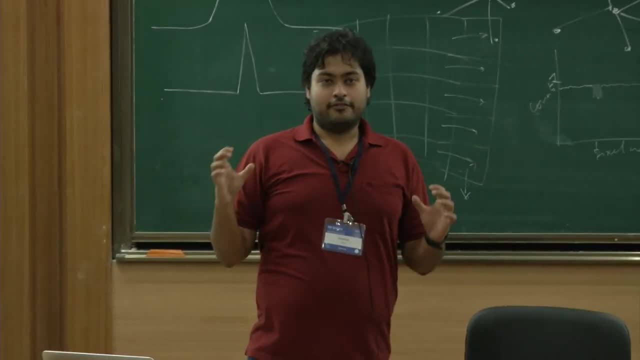 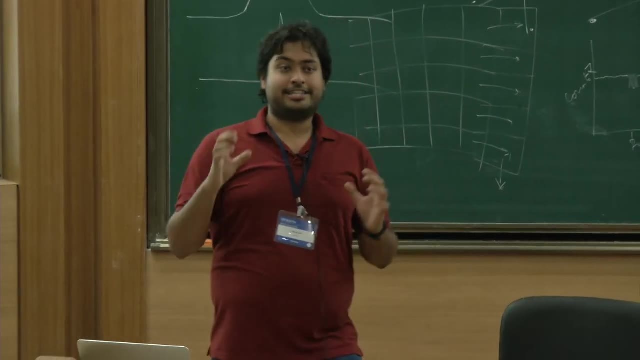 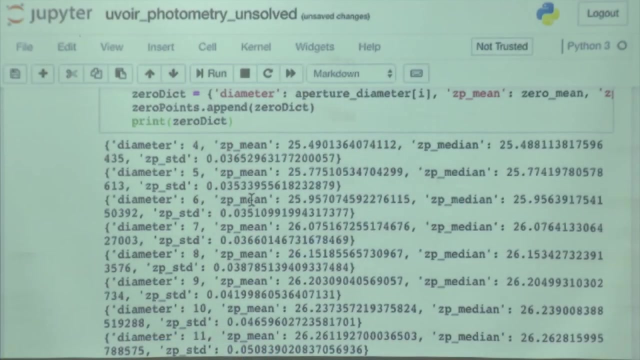 I am computing a zero point because you, for each aperture diameter, you can compute a zero point because, as I said, the the you want to measure the flux of your source in the same aperture as that of your science target. so I'm computing this here. so what I did here was I just stored all the results. 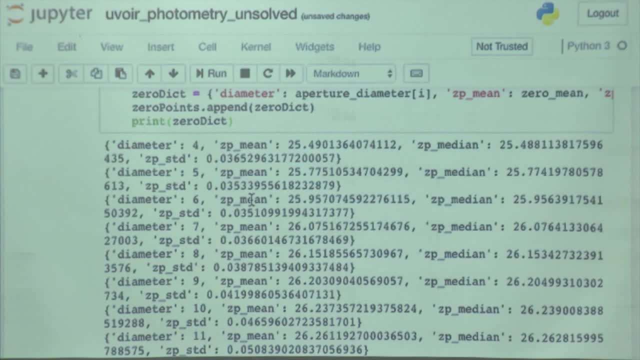 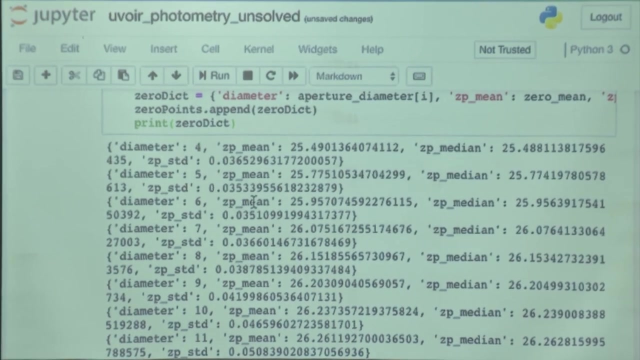 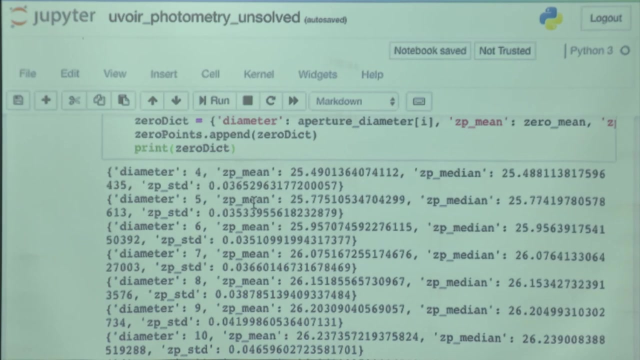 into a Python dictionary where what you're seeing here is the diameter of the aperture, the zero point and the scatter in the zero point. what is the scatter in the offset between the known, between the known pass as magnitude, and the instrumental magnitude? it's more of a computing, a constant offset. I'm not fitting. 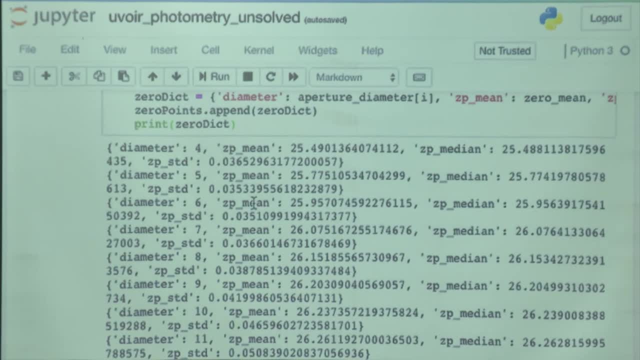 us is this: it should be a constant offset. yes, yes, unless if your slope is not one, then it's not this. yes, yes, in the slope should be: yes, yes, yes, the slope should be one for a good instrument. yes, yes, yes, yes, exactly, yes, right, so okay, so. 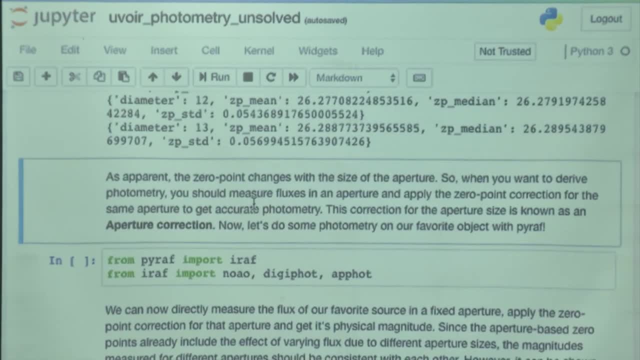 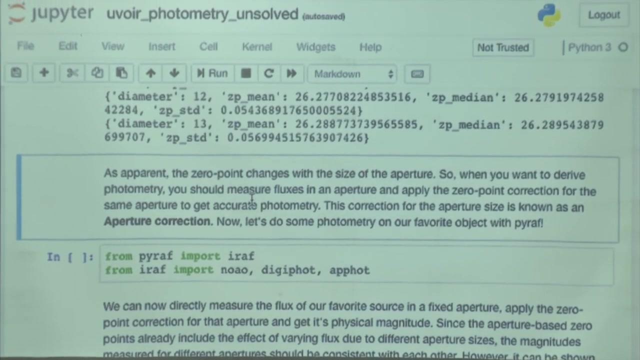 the next step is a bit tricky. I we were, we had some. we had to struggle a bit to get pi ref, so pi ref is so I'm okay. so i ref is a general set of tools that is quite useful for doing many things in astronomy, except it's ridiculously difficult to install and we had some. 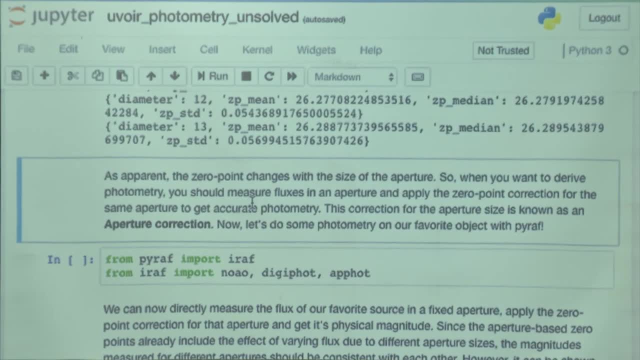 difficulties in installing it. so in principle. so once you have the zero point for each aperture, you want to go to your favorite science target, put an aperture on that science target and measure its flux. and I ref does have really well laid out routines for doing that, except we don't have that running. 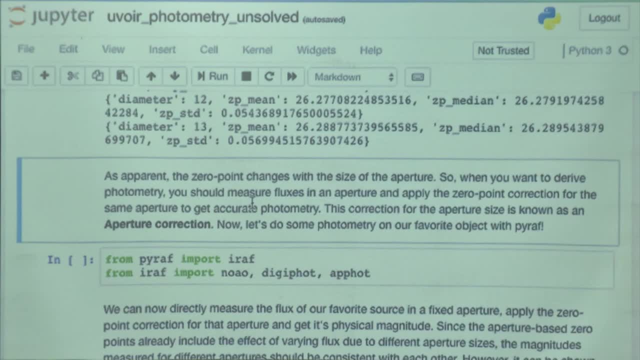 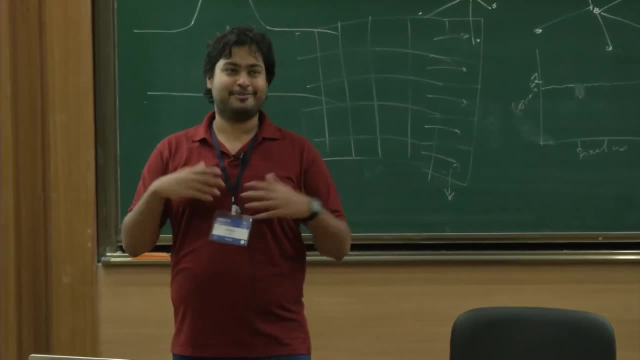 in this docker right now. so what we'll do instead is I I've run it on a another machine that actually has pi ref installed, and you should just use the output from I ref. just believe me this, so you don't have to run these steps. these steps will not do, is this? these steps will not work. 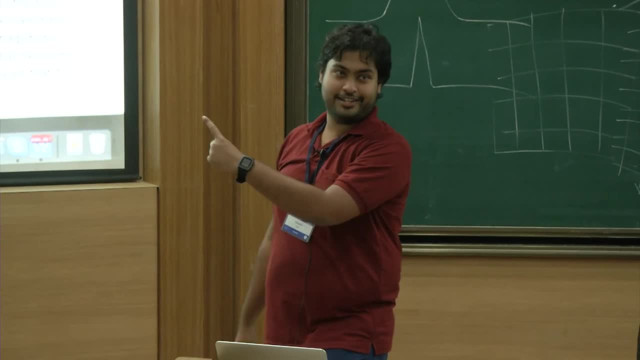 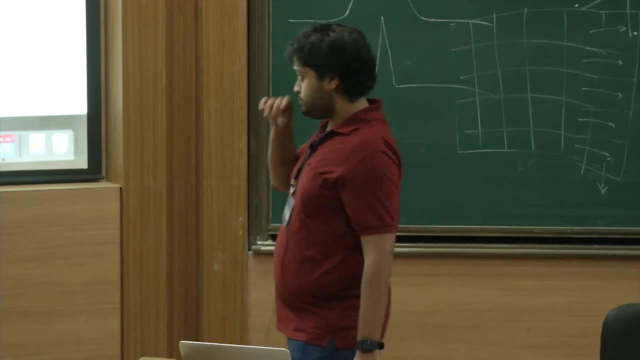 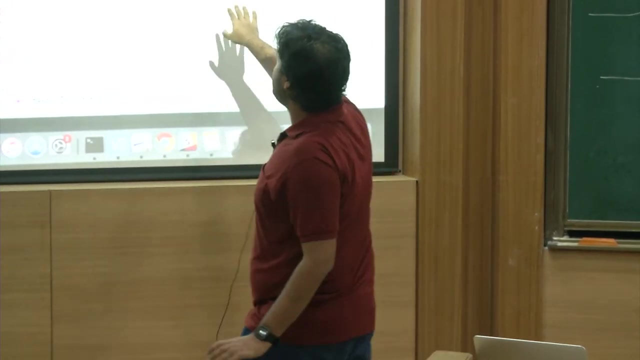 in case you have a separate running machine where I ref works, this might work. doesn't work on this docker, so just skip over to the next cell where, if you downloaded the latest data, that latest data folder that you got pointed you to, there should be a file in that folder. if you go to data photometry plus this: 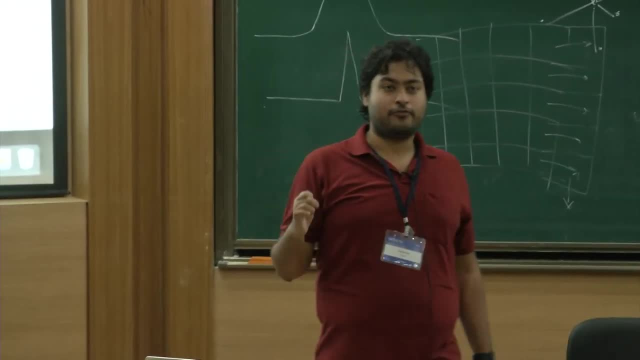 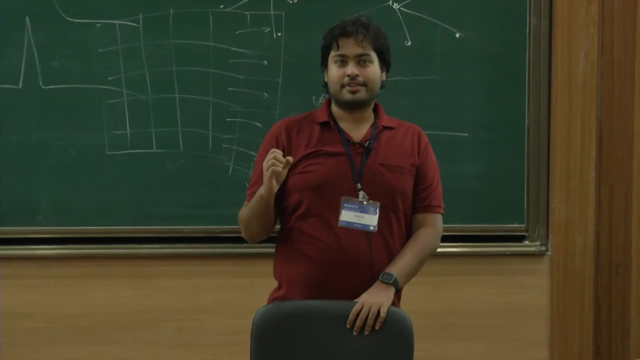 extension. this already has the measured magnitude of our science target. so in this case, just so you know, yes, our science target in this case is a- is a Cepheid variable. it's called v641signe. you can look up v641signe, it's a. 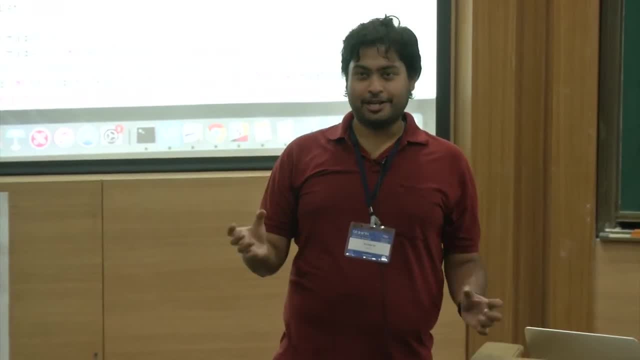 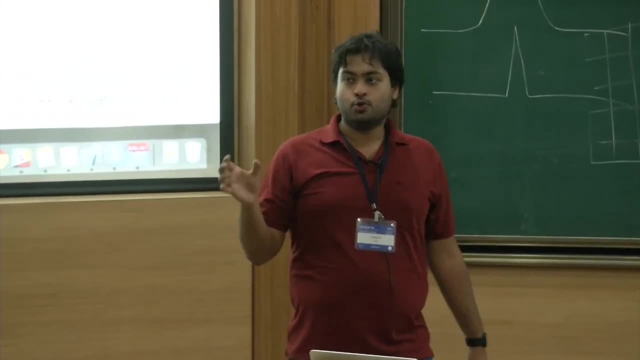 Cepheid variable that, as, as the name suggests, it's a. it's a variable, so its magnitude changes with time, and in the light curve analysis module you'll actually be using photometry to do to actually see what the Cepheid variable does as a function of time. but 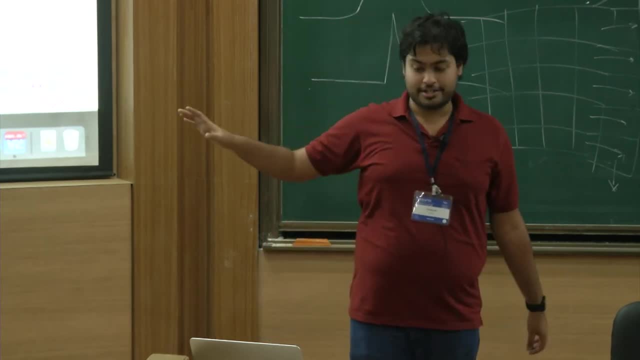 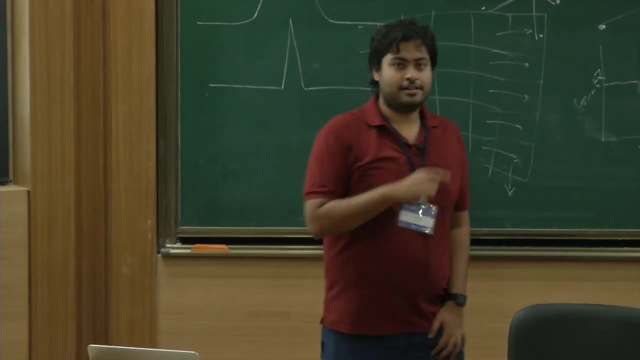 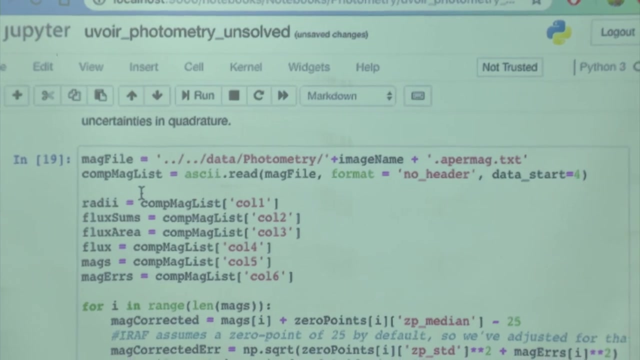 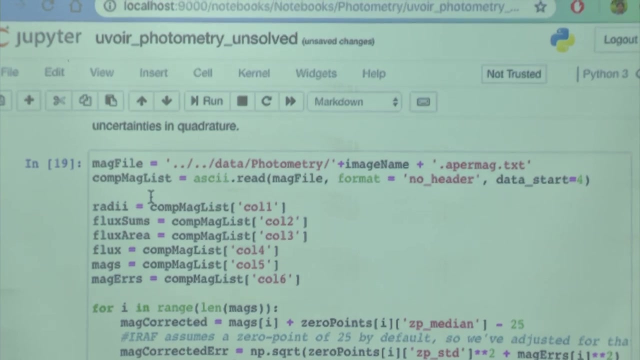 in this case, you are actually seeing how that photometry was generated. so if you just run this cell, okay. so try running this cell, if so, okay. so, path, yes, the path, yes, okay. so I want you to pay attention to the, the magnitudes that were actually measured. 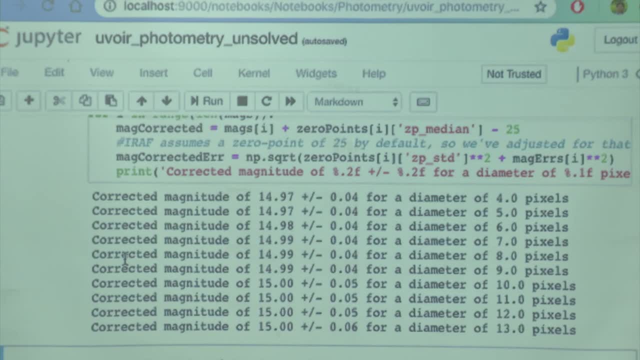 for this source. so if your aperture correction worked fine, in the sense that your zero points were consistent with what you would expect for bigger and bigger apertures, it should not matter what your aperture really is. you should get the same magnitudes across all apertures. that's the point of the 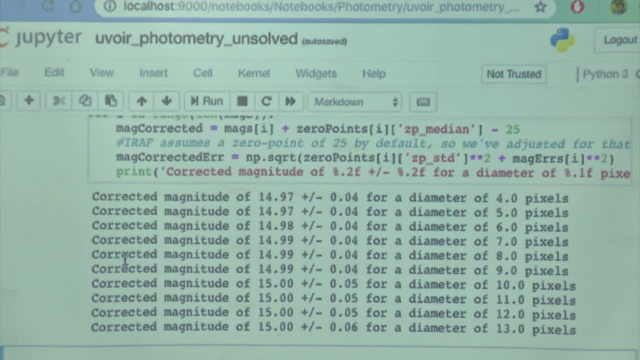 aperture correction. so, as you see, here the magnitude are all magnitudes are all consistent with each other within the error bar. so the error is about five percent, less than five percent for most cases, and what you are seeing is that for diameters already ranging all the way from four pixels to about fourteen pixels, you get exactly the. 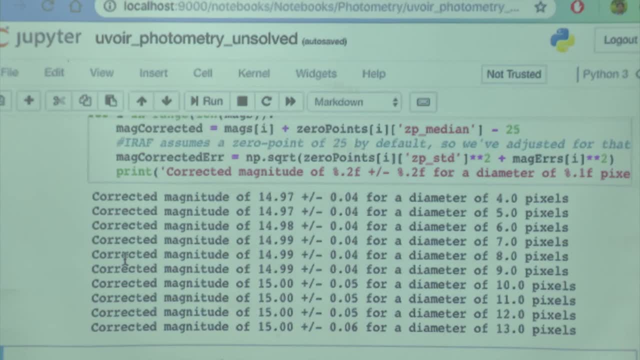 same magnitude, which means that your aperture base zero points are fine, and in this case so. in this case, if you wanted to decide the size of the aperture, you should really select the one that maximizes your signal to noise, but otherwise there shouldn't be any difference. 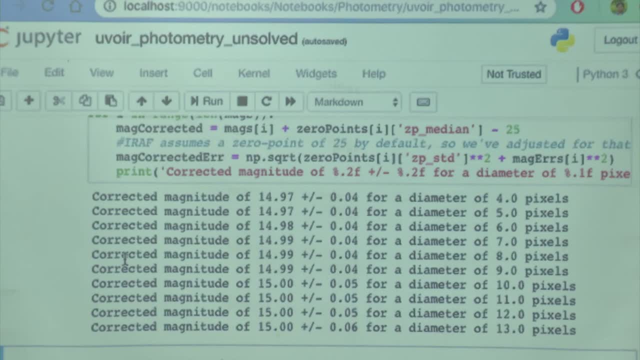 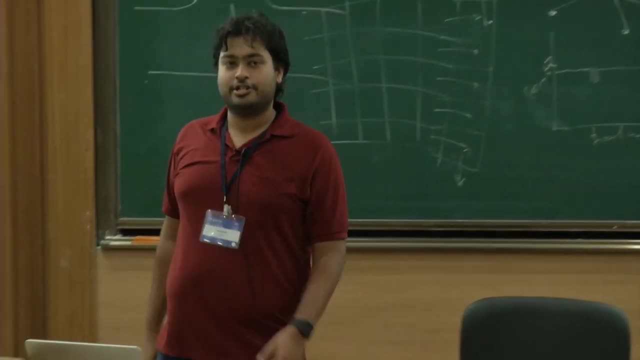 between the approaches that you sorry, the magnitudes that you measure in different approaches. So we are running a bit short of time, so there is. the rest of the module is actually dealing with PSF photometry and, as you already heard in the lecture, the idea behind PSF photometry. 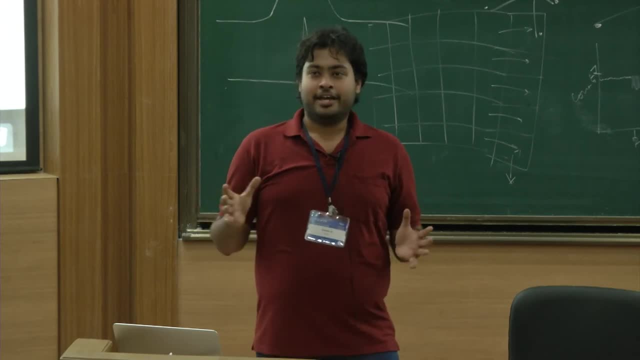 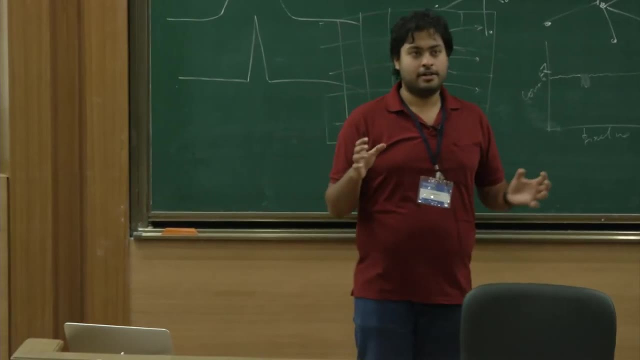 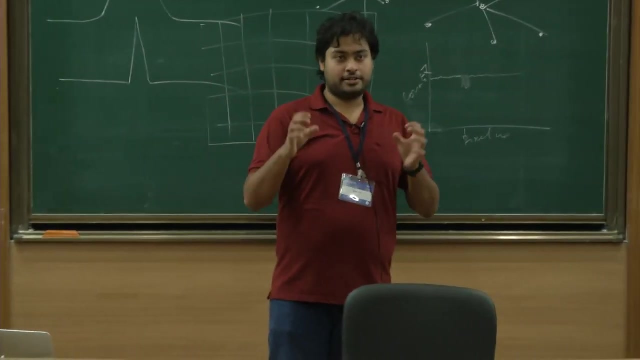 is not to measure magnitudes in fixed apertures. instead, you take a few good stars inside the field and you compute. what is the PSF, the point spread function of stars in the field. and once you get you get a model for what the PSF actually looks like, you fit that PSF. 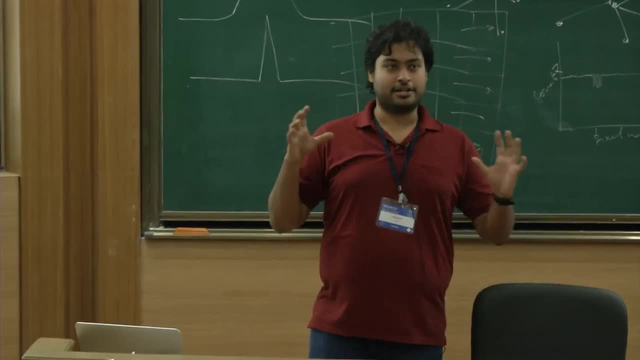 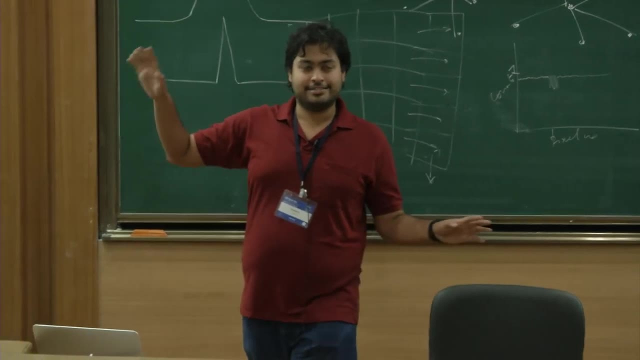 to all the sources in the field to derive PSF based magnitudes. these are all PSF magnitudes and these are particularly important when you are dealing with crowded fields, because in this case, it is a crowded field but it is not as bad that you would not be able to. 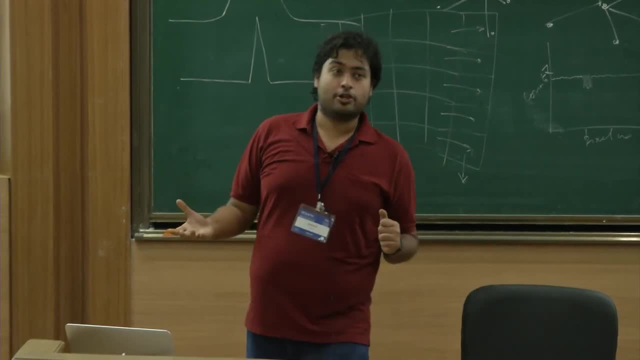 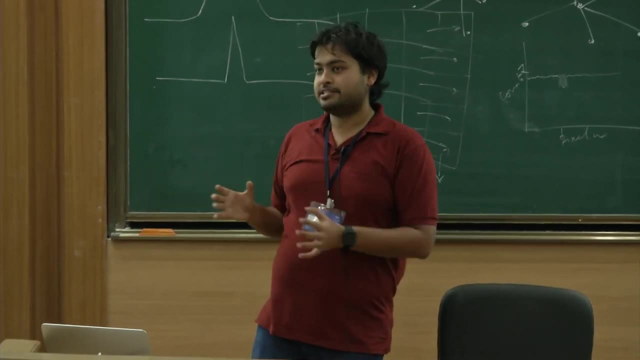 get aperture photometry from this. but if you are looking at fields like globular clusters, for example, where you have stars overlapping everywhere, in that case you want to actually compute a PSF model for then stars in the field and then fit each and every star in the field. 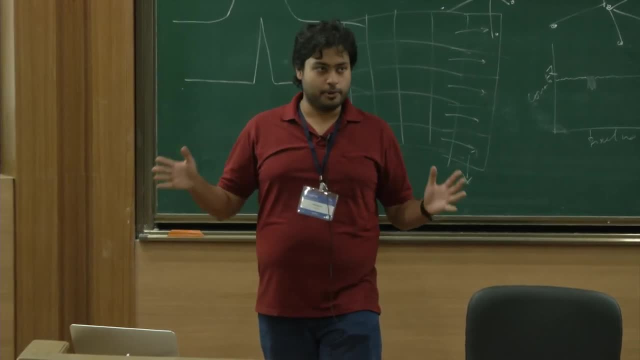 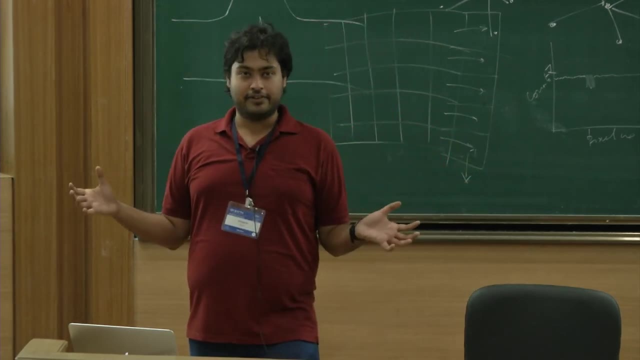 with that PSF model. and once you fit a PSF model you can compute what is the total flux inside that PSF and do exactly the same thing. you fit a PSF model, derive fluxes for all of the stars in the field and then derive a PSF based zero point. once you have that, 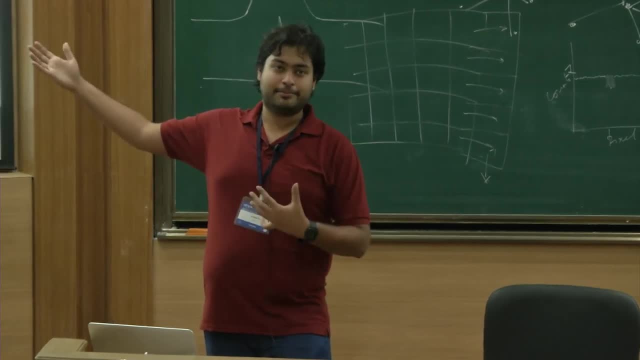 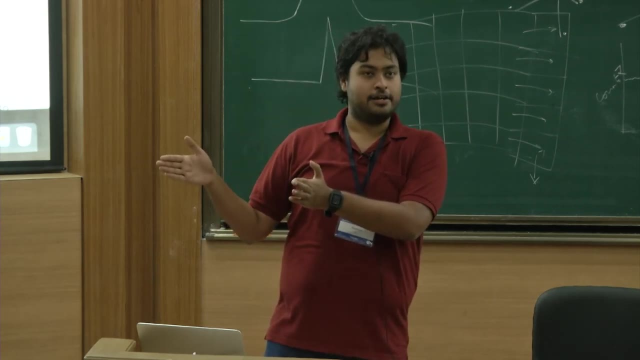 once you have a PSF based zero point, you can again apply the same correction, which is: take the PSF based zero point, add the, add the instrumental magnitude, which is again measured from a PSF, measured from PSF fitting, and then apply the same thing. you should get exactly the same. 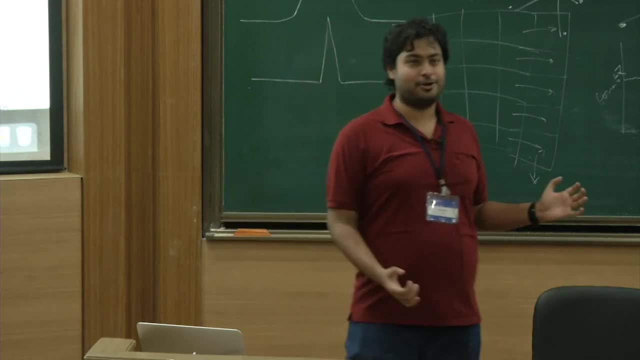 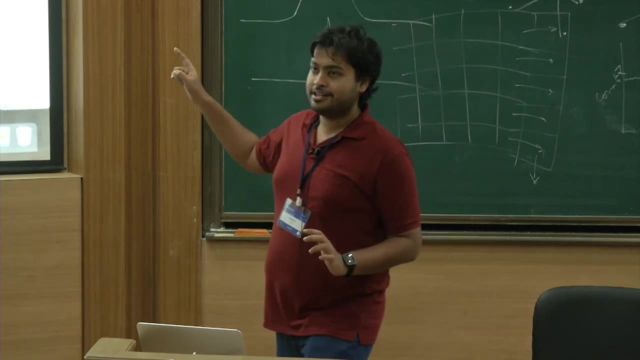 answers. it should not matter what you are using: aperture photometry and PSF photometry. this is different ways of doing the same thing, but the magnitude should be the same. unfortunately we do not have time to go into this, but the solved module will have all the stuff that 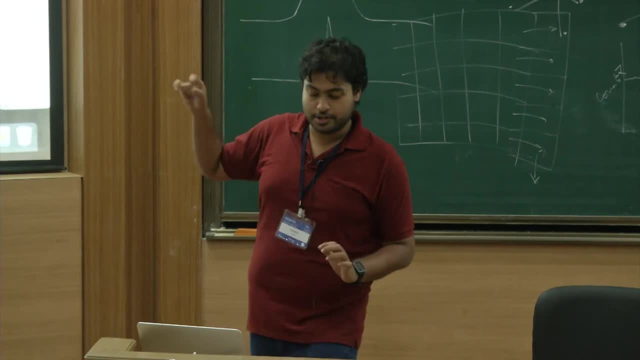 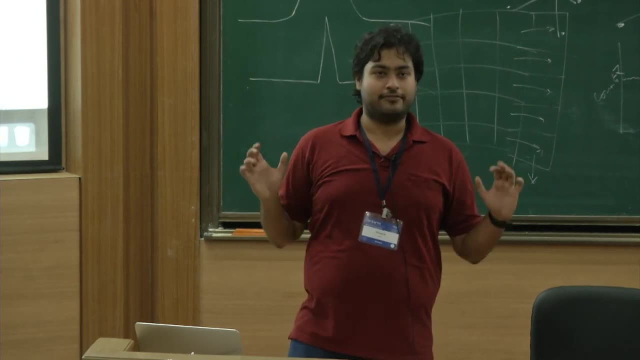 you need to run. so in this case we were using a code known as PSFX. its PSFX is what it does is: does this PSF computation and does this PSF computation and does this PSF computation and fits all of the sources with a PSF and gives you PSF based magnitudes. but we do not. 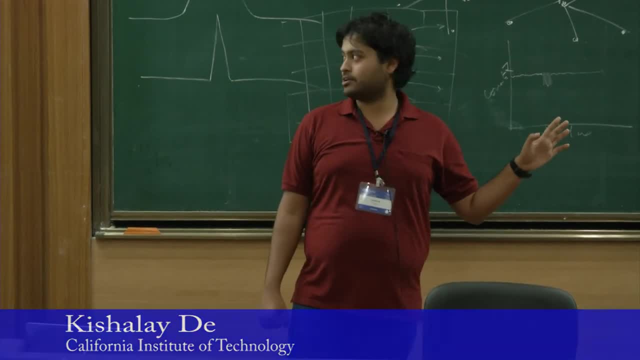 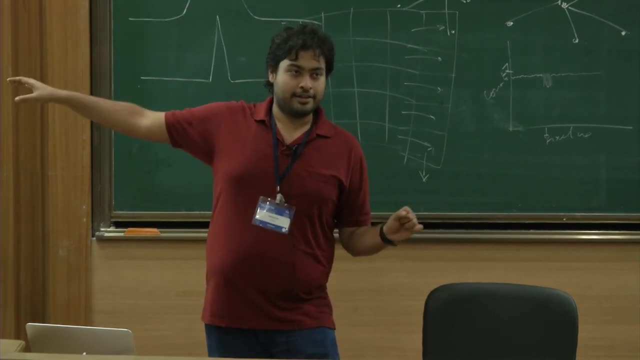 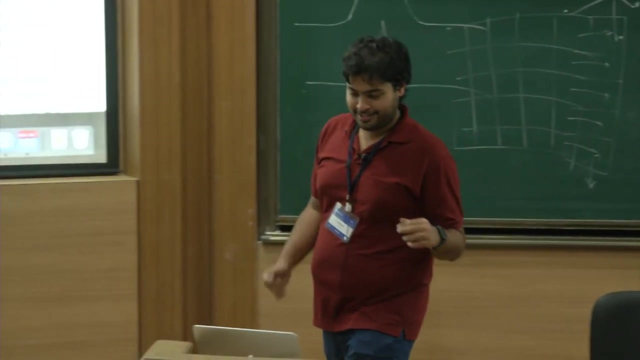 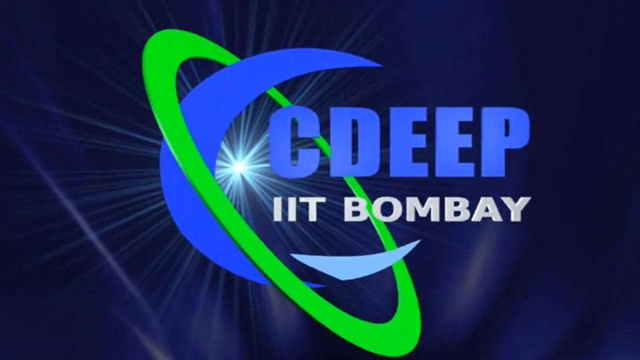 have time for that, but if you have any questions, please feel free to contact me, and you should be able to run this, the solved version of this notebook, when you are trying to run the rest of the thing at your leisure. so